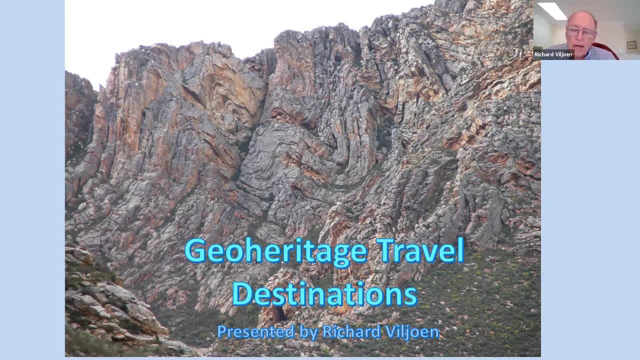 particular thing, aыс, Vineet Demachos, and in fact we way. we start to think about our locations heritage in South Africa. As you are aware, the COVID pandemic has affected tourism pretty badly during the past six months, not only in South Africa but worldwide. but we believe that they. 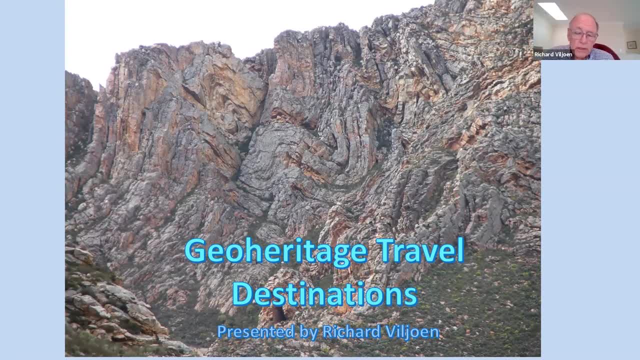 could shortly be a shot in the arm for the local tourist industry because of the pandemic and the lockdown, Tourism products- of which geotourism could figure prominently- exist, and so what we'll do is present a brief overview of how, by using the input and the knowledge of the geological 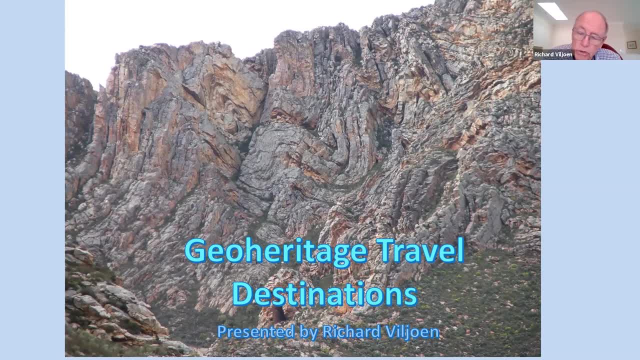 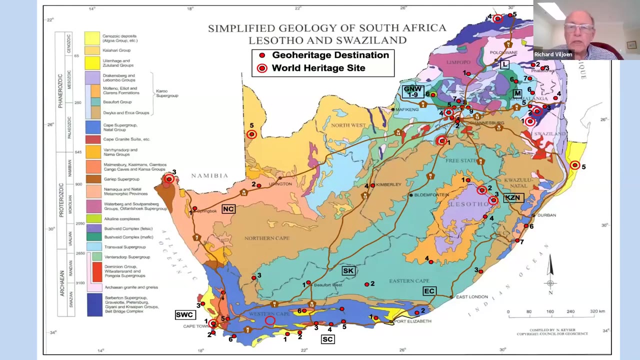 community develop some of these geotourism travel destinations, as we've called them. So if we have a look at this map, we have listed over 50 potential geotourism travel destinations in South Africa, as shown in this slide here and, however, at this: 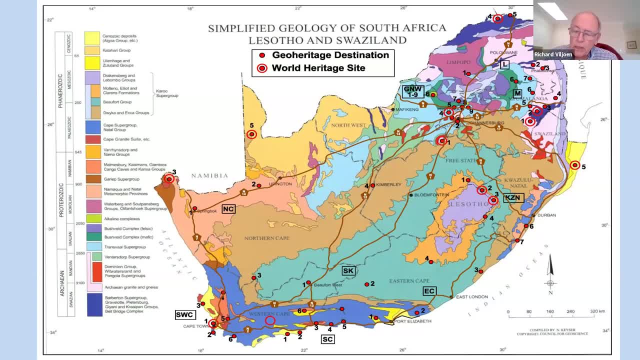 stage, there's no real coordination of geotourism products for most of these areas and we believe this is a huge gap right now which needs to be filled. So, although circumstances, I should just explain that the sites that you see here are sites that we have investigated or seen or deemed suitable for. 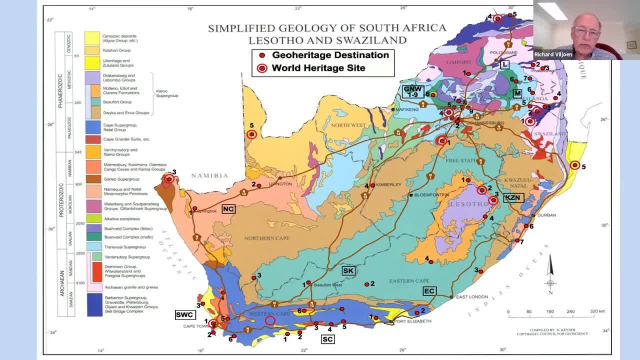 a geoheritage travel destination. As you can see, most of them are on main roads and pretty close to main centres, so they are, in general, accessible. They include 10 of the World Heritage Sites of South Africa and, as you know, out of the geoheritage sites, virtually all of them have some very significant 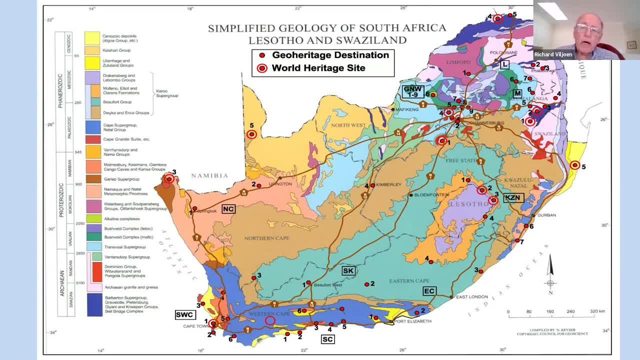 geological features, and this applies, for example, to the Barbiton Mountain Land, the Barbiton World Heritage Site and to the Freeridefort Dome, but also to others. For example, Mopengubwe has a strong geological component as well, obviously, as the cultural component. So 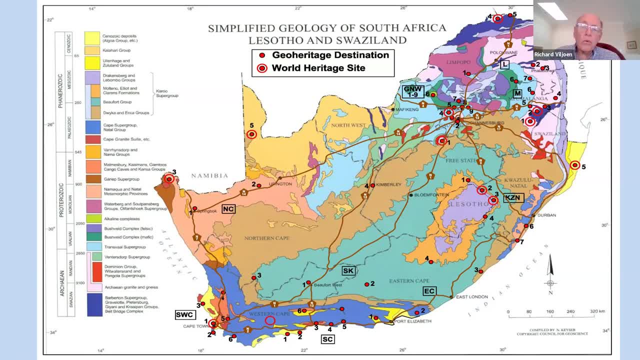 geology is playing a very, very, very important role in this. I think that's why we're looking at important part in our World Heritage Sites. But besides the World Heritage Sites, there are these other at least 50 sites or destinations which warrant. 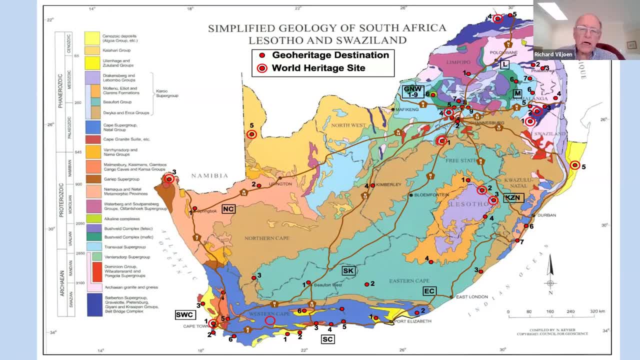 recognition as tourist destinations, and it's these sites and the World Heritage Sites that need upgrading to world-class geo heritage destinations. So this is what we're talking about, and so what we envisage is that, although the circumstances might vary, we envisage the following general scenarios and: 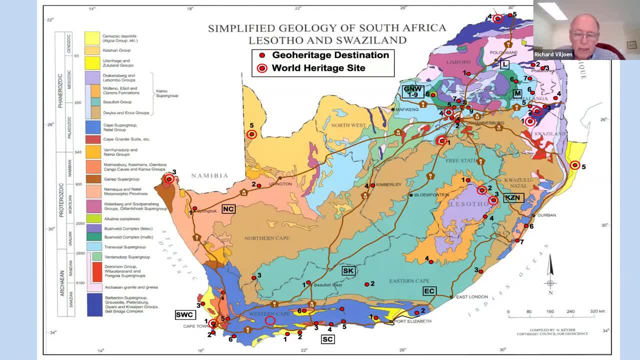 procedures for each of these travel destinations, So each of the destinations take one of the red spots there- would typically incorporate a number of important geo sites which the Geological Society of South Africa are working on at the moment: Geo heritage sites, Heritage Committee and other attractions close to and linked to the local road system. 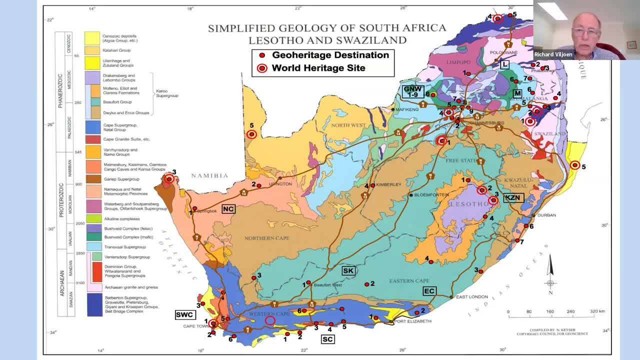 with the potential of developing one or more geo-tours. So the geo-tours are pretty important. in all of those destinations, Sites or features of archaeological, paleontological, scenic, historical, scientific or other interest within the destination, including the fauna and the flora, should also be incorporated. 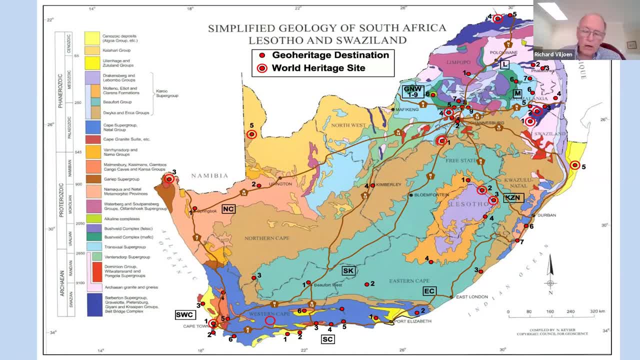 where appropriate, to provide a more holistic view of the destination. The overriding theme, however, should remain geo-heritage. Another point is that a central information centre with the exhibition providing details of the geo-heritage destination should ideally be established within the destination. 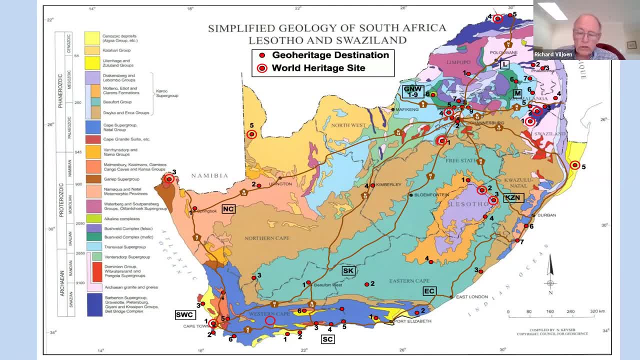 A video of the travel destination and or virtual tour Should be produced both for the information centre and the geo-tourism website. A tour guidebook for the information centre and website should be produced. Local guides and tour companies should be involved in arrangements made for the training of tour guides. 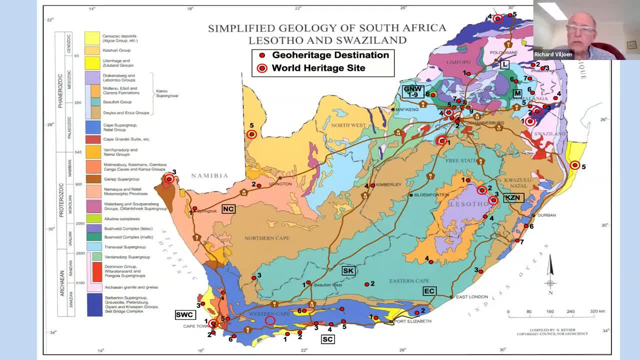 And then there are also huge educational opportunities at each of the destinations, And special products to cater for learners and others should be developed. Thank you, Thank you, Thank you, And as a result, we'veceğ побед as well. 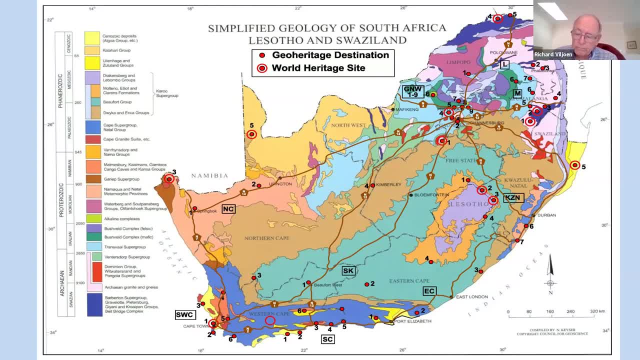 Importantly, sponsorship should be obtained to get these developments going, And also the support of the geological community is essential to help in getting these various initiatives going. So the buy-in there, we believe, is crucial to the whole thing. There also needs to be, and there's, room for, coordination and communication between the two. 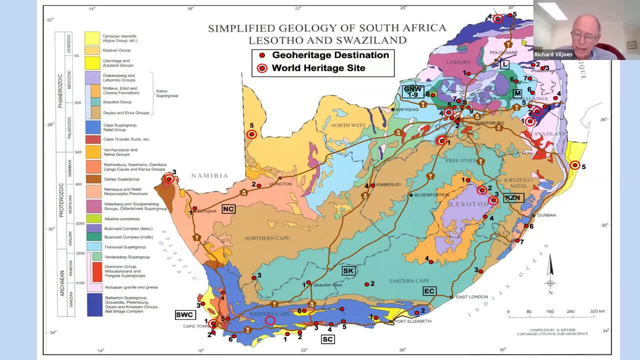 There's a lot to come. the various geotourism initiatives and geotourism destinations should ideally form part of a country-wide network with links to SA tourism and provincial tourism, and Alan later will provide some ideas in this regard of our thinking at the moment, and Morris will provide an example of a 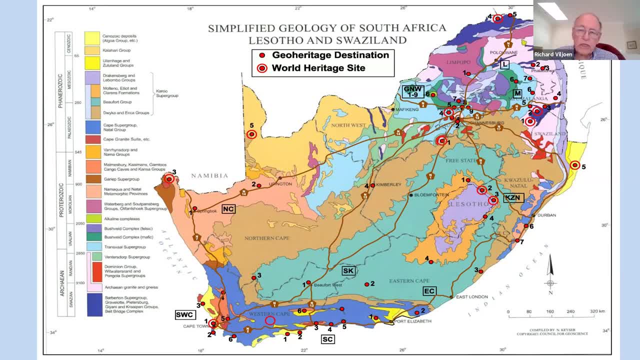 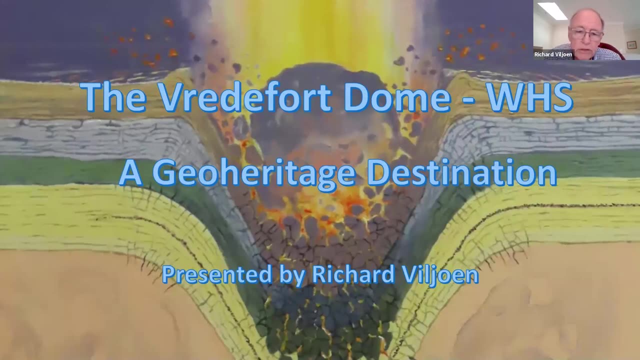 travel destination in the southern cape, in fact the garden route. so that will follow this presentation, which looks briefly at the the Firafort story now. the Firafort dome world heritage site has been on the table for a number of years now and a major information center was. 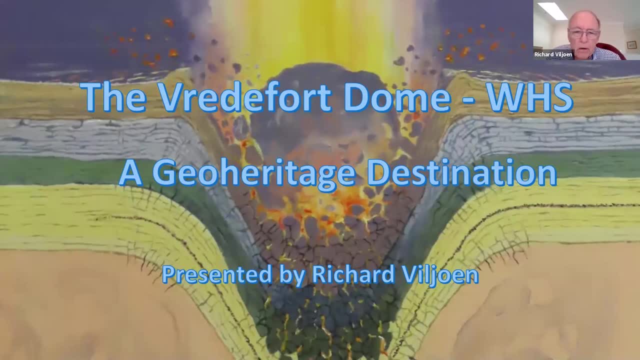 built this. the center unfortunately collapsed and no longer exists. so so tourists arrive at Firafort, the world heritage site- and and they don't know what the heck they should be looking at. so it's a very, very sad state of affairs, and this not only applies to 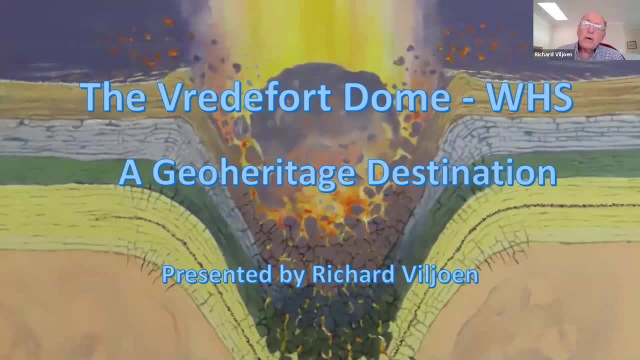 Firafort. it applies to other areas as well. so about 18 months ago, a group of people, including the, a newly established museum in Firafort, and with the Maggie Newman, who is the geo artist, and, incidentally, geo art plays a very important role. we believe in tourism. 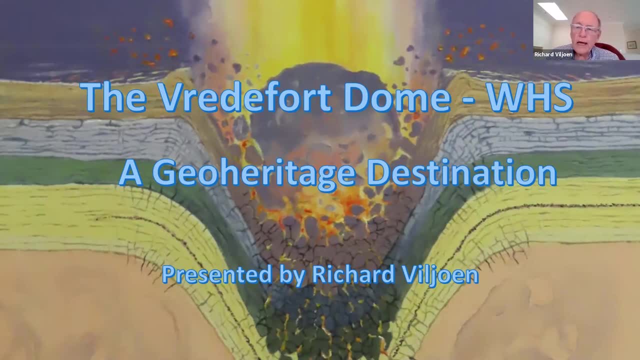 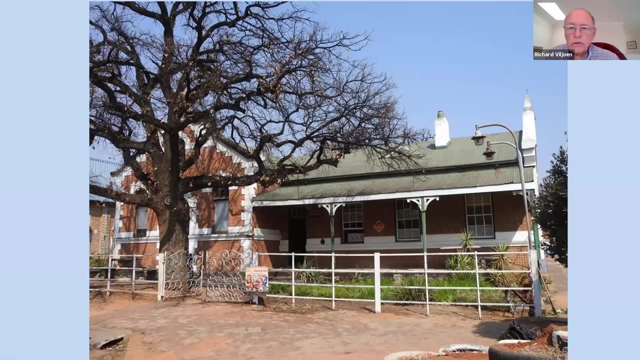 because it depicts things in a in a more pleasing and understandable way. so, getting together, we decided to use the Fira the Perace museum as an information center for the Firafort dome world heritage site. and that's a photograph. it's an historical heritage site and it's a photograph of the Firafort dome world heritage site and it's a photograph of 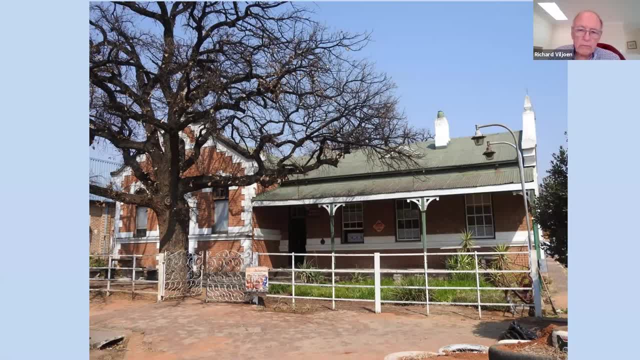 from the lego β away you can see the buildings that will go on a right- the Cyprefero sandals on the left now, with no icaid, belong to the natural heritage nyt against the Willis الم and the original building in its own rights, and it was in a rather dilapidated state. it's now been upgraded quite considerably and a info and an information centre has been established over the last six months or or so and went ahead to this below, so you can. we are planning a geo heritage stage tour as well, but we'll talk about that a bit later. so these are type of exhibits and other. So these are a type of exhibits and other. ogre Sabala, there's also a new type of achievements which have been built from this research site, but after this was built in this 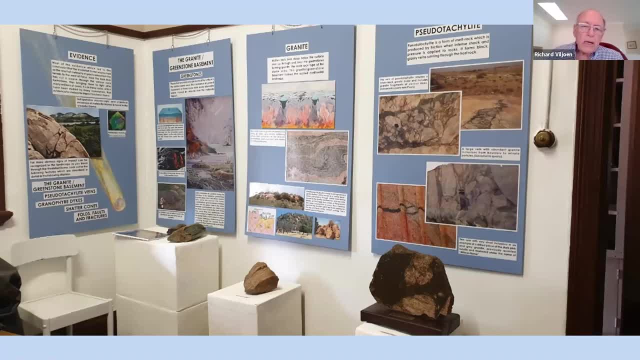 within the museum where the different panels showing different aspects of the meteorite impact and also showing different rock specimens that relate to the panel. So, for example, on the right here is a nice little piece of pseudotacolite which is a hallmark. 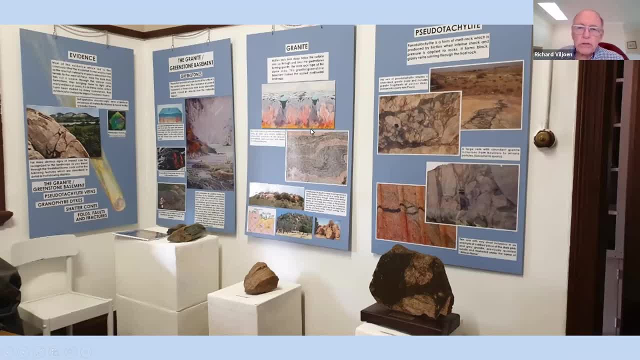 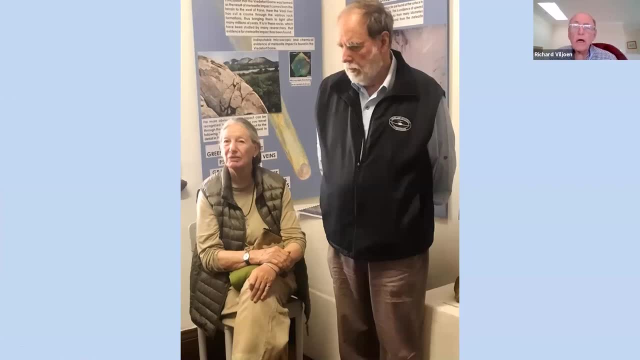 rock of Feuderfort. And then of course, sponsorship was quite important and in this area we were quite lucky to have the input of the Oppenheimer Trust and they were actually at the opening of the Feuderfort Museum Information Center and they thoroughly enjoyed it and hopefully we can get 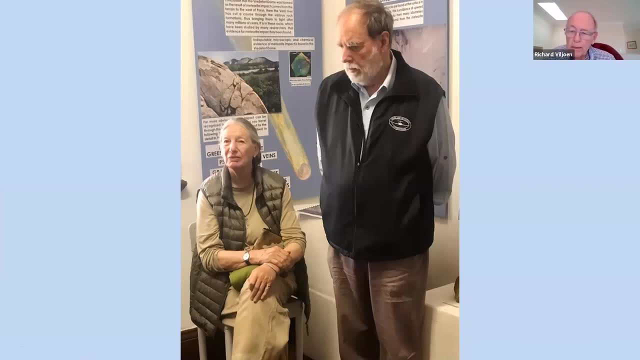 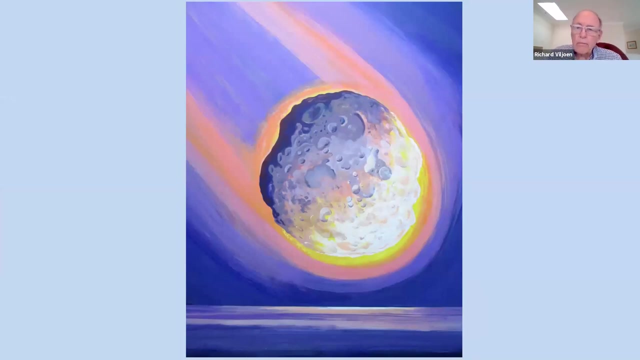 them on board through their trust and other channels to help in the financing of some of these geoheritage sites. So the exhibition starts off with the artistic portrayal of a meteorite- Sorry. incidentally, I should also point out, very importantly, that another sponsor of the geoheritage initiatives has been the 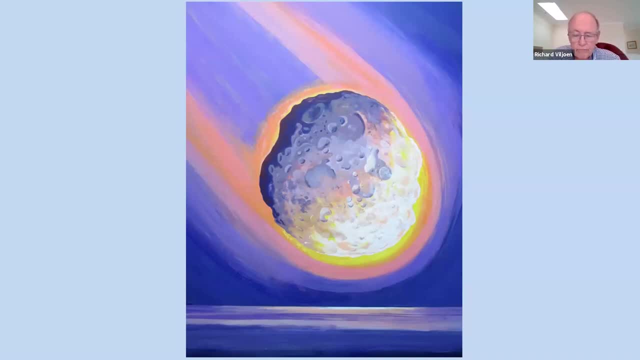 legacy fund of the 31st International Geological Conference. So they've played an important role and will continue to play an important role in helping to finance some of these initiatives. So the Feuderfort exhibit then starts off with a portrayal of a meteorite. 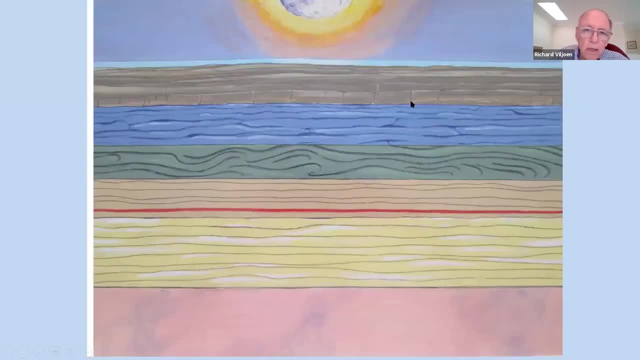 plummeting towards the earth at high speed. As it approaches, it comes into contact with a sequence of layered rocks. bearing in mind, this is now for tourists, for tourist consumption. So at the base we have a granite basement of very old rocks. We then have a sequence of yellow and brown rocks. 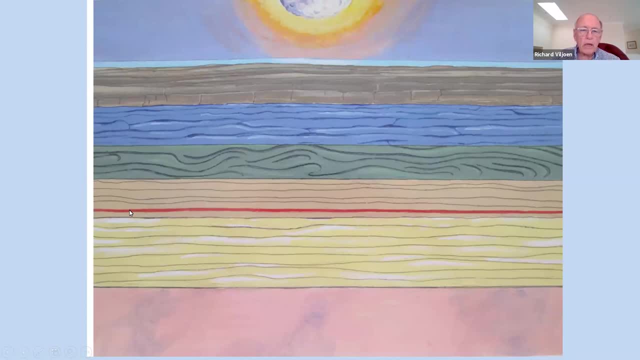 which are the Witwatersrand Stroke, which contain the gold-bearing rocks of the famous Vidvarasram gold field. Those are overlaid by larvas sequence of larvas, and the larvas are overlaid by a sequence of dolomitic rocks. 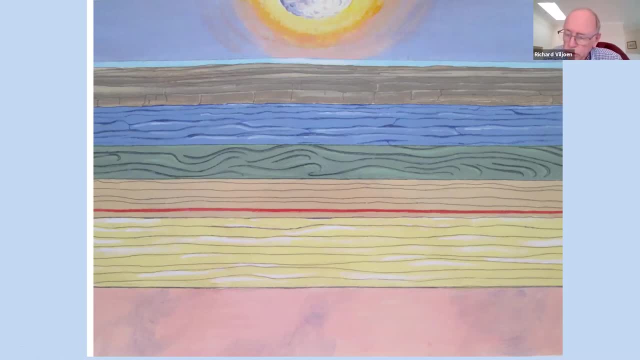 which, further north, as you'll see later, host the World Heritage Site of the cradle of humankind. So very important rock formations here and at the top, some further sequences of quartzites and shales of the Pretoria series. So those are the rocks that are impacted by this incoming meteorite. 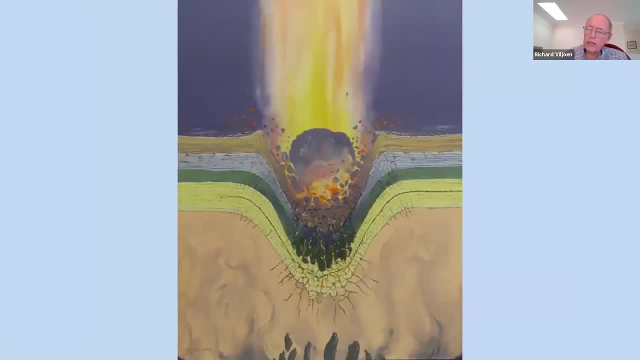 And so what happens is a major catastrophe. The meteorite was larger than Table Mountain, a huge event. It caused instability, Total instability in the crust. It caused the down-warping, Also told by way of pictures or paintings. again, May's paintings. 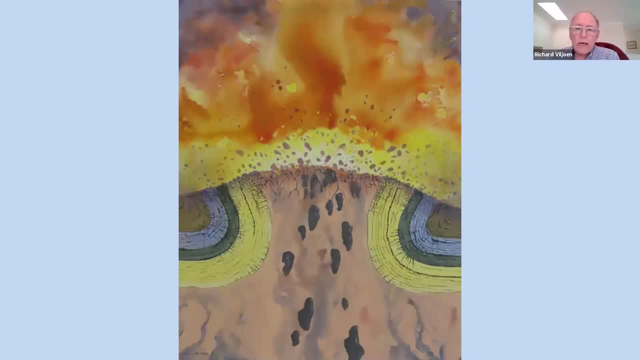 And then, very importantly, the rebound of the central uplift. So, after the impact, there's release of pressure and everything comes up as a dome. The meteorite is largely vaporized And, as you can see, the basement granite with fragments of the greenstone. 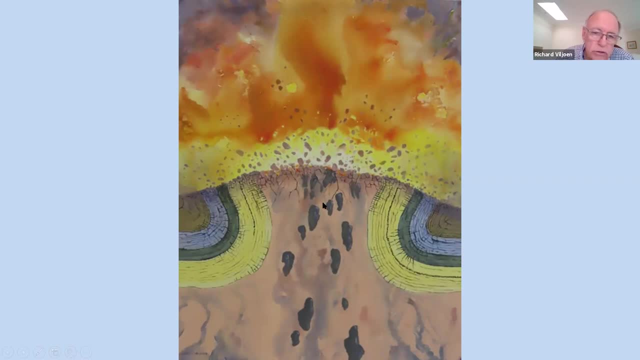 which are the very ancient volcanic rocks and others of the Earth's crust, are up-domed into the center And the overlying sediments which I explained are overturned And a fallback Pretoria is formed in a crater, forming a melt rock. 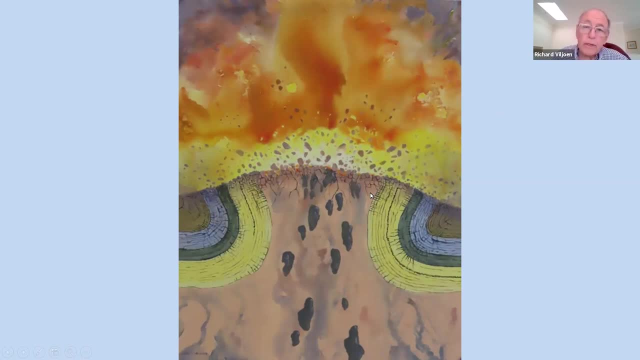 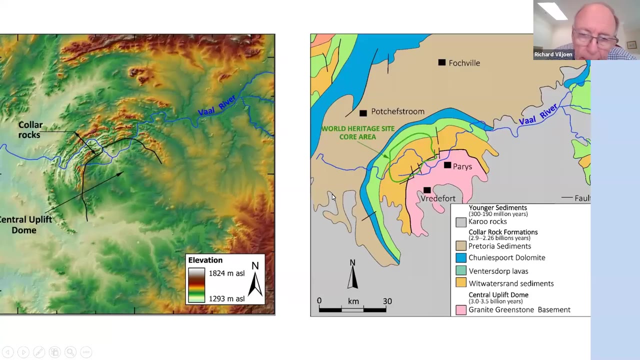 So all of these things happened just immediately after the impact of this meteorite. So what happened is that at the moment, what we see on a satellite, or actually a digital terrain presentation, is a beautiful circular structure, here caused by this impact and with the overlying collar rocks etched out. 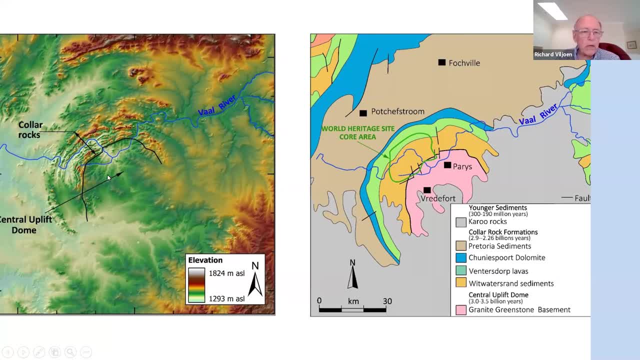 and the central uplift dome over here, And then you can see how it relates to the geology. the central uplift dome, There's Piraeus, where the information center is, And these are the Vidvarusron strata, the volcanics of the Vandersdorp. 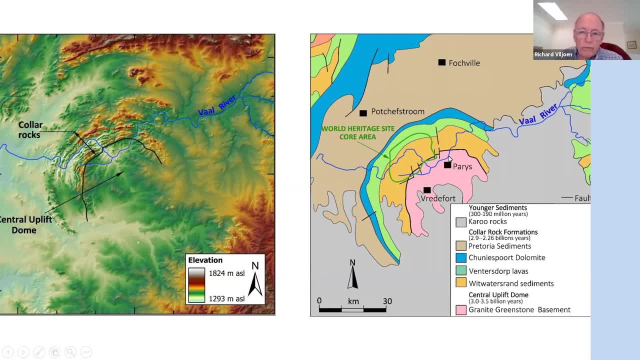 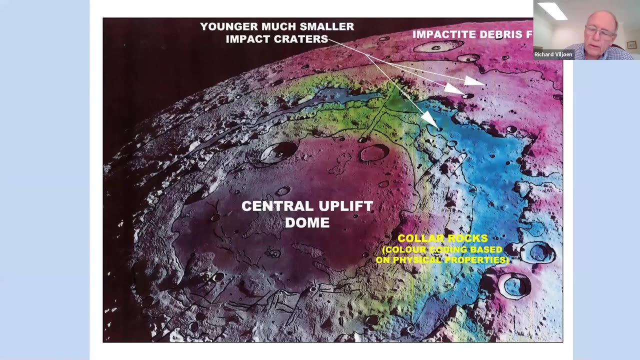 and then the Dolomite strata. So that's really the evidence. Some of the evidence is this fantastic structure which can be seen from space, this beautiful circular range of hills And, to emphasize the point, one has a look at a meteorite impact structure on the moon. 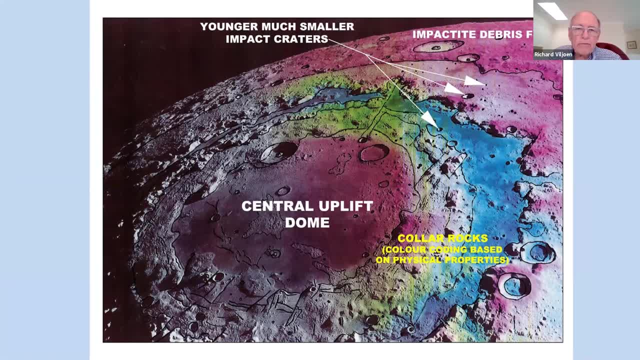 This is actually, I believe, the far side of the moon, where you can see the central uplift. over here You can see the surrounding material of different materials, the blue and different colors here. So those would be equivalent of the collar rocks of Piraeus Fort. 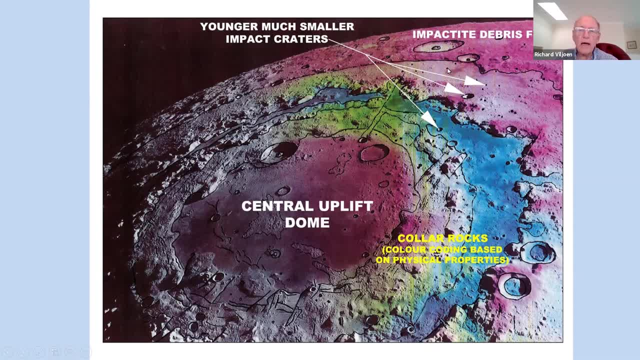 And then a huge impact debris field over here which, in fact, has now been removed by erosion in the case of Piraeus Fort. And it also draws attention to some younger meteorite impact craters, smaller ones- You can see them here- little ones. 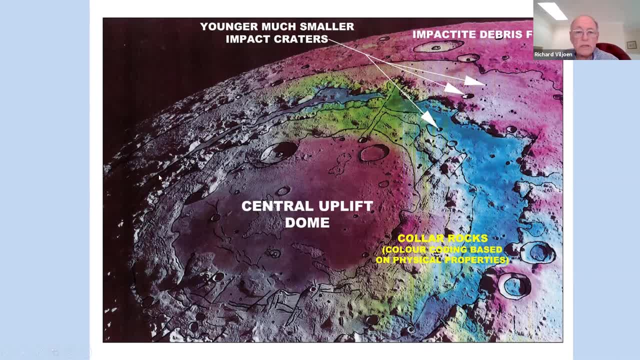 Those, of course, we don't see at Piraeus Fort, But we do see the major structure which is analogous in size to this structure that we're seeing on the far side. Well, some people have seen it, but on the far side of the moon. 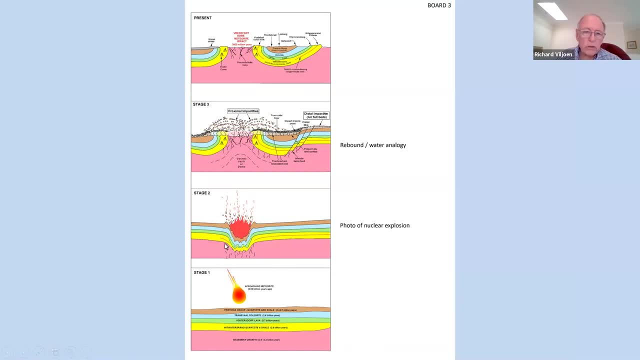 So, again pictorially, the events are depicted over here, And then there's the fallout breccia, the debris material, And then finally the section across over here where you can see the uplifted area, through here And you can see how the strata exposed in the Johannesburg area. 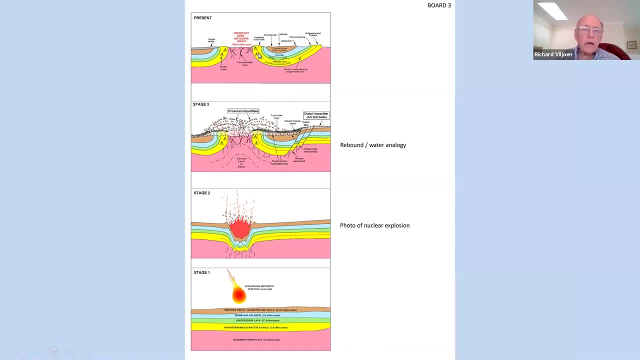 and then, coming through a major, it's inclined and exposed in the Piraeus Fort collar, And the same applies to the lavas, And the same applies to the dolomites, and so on. So an amazing story that the impact has caused this huge uplift. 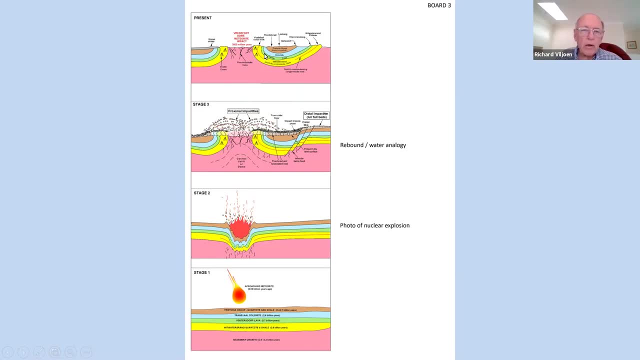 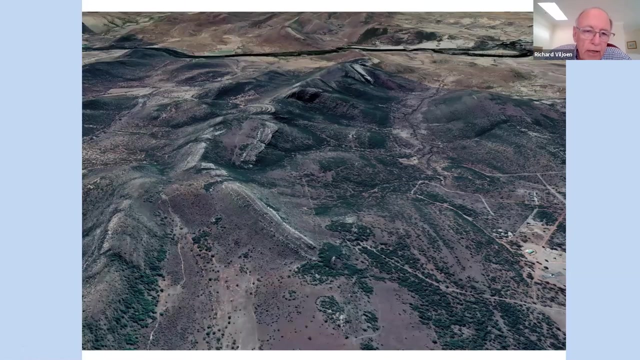 exposing all the rocks that we get around Johannesburg Dome. It's another domal structure around the collar of Piraeus Fort, So that is quite a unique aspect of this impact. So now the structural effects, of course, are very marked, And some of them can be seen here in the collar rocks. 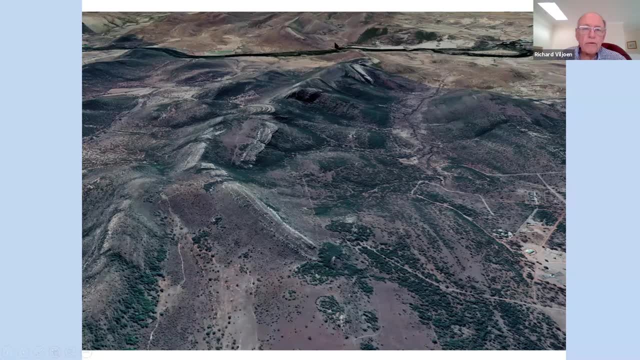 Incidentally, that is the Waal River which runs through the Piraeus Fort Dome area. through there And you can see these white layers here of quartzite. You can see how they have been faulted. These are actually overturned. If you look there you can see a quartzite layer that is lying like that. 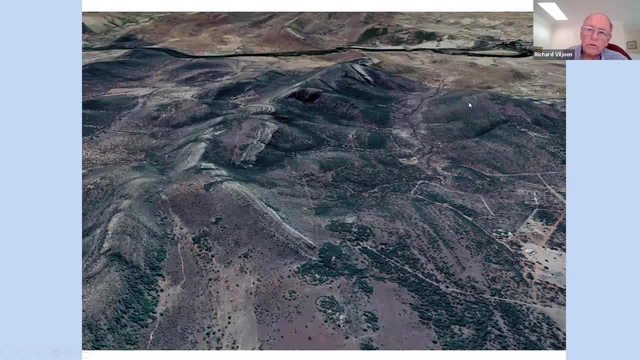 It's actually overturned so that the center of the dome is to the right over here. So major, major structural complexities involved in the rocks over here, And of course, attention is drawn to the fact that one can then go out into the field and observe these various features that we're looking at. 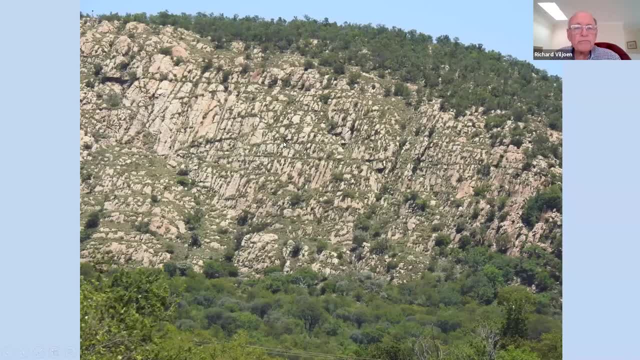 And there is one of the overturned slopes And you can see it's a dip slope on the Orange Grove quartzite, as we call it. You can see the immense amount of fracturing and structural dislocations that are going on in that particular thing. 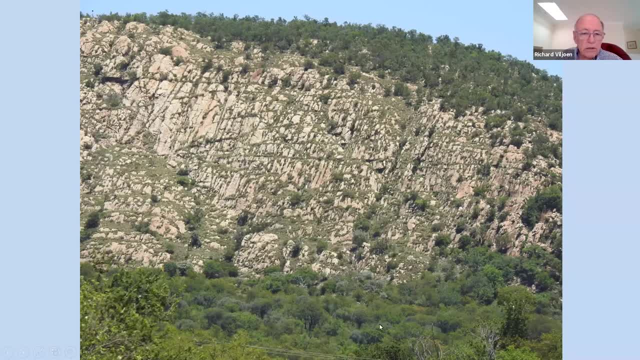 Another thing that you'll notice here which is very important, and that is: just have a look at the vegetation growing here in this material. down here It's got a lightish green hue in general, with more olive green in between, as opposed to the vegetation growing on top of this very silica rich soil over here. 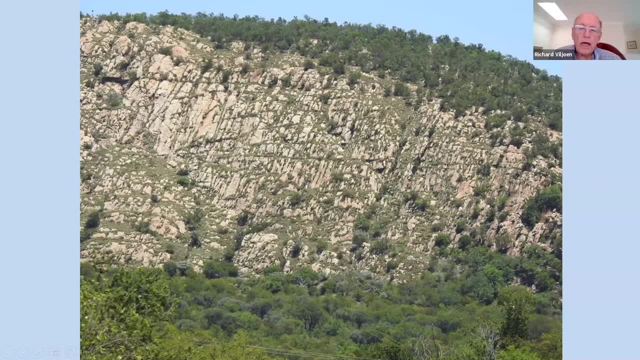 And that highlights the importance in the Fierrefort area not only of the geology but of the vegetation and the differences in vegetation, between vegetation growing on different soil types And, in general, the fact that a bush felt type environment has been preserved in the ridges of the collar rocks of the Fierrefort Dome. 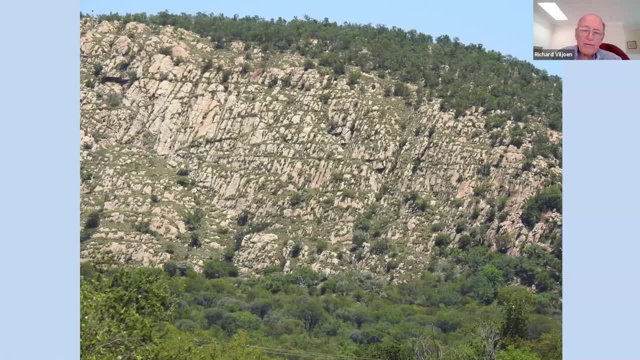 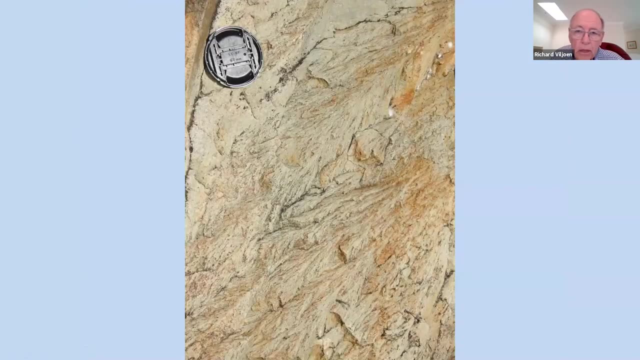 So that whole meteorite thing has had an impact even on the vegetation which we now see in the Fierrefort Dome. So that's a big story that links in with the geotourism in this area, And then, of course, the features that you see in the rocks. 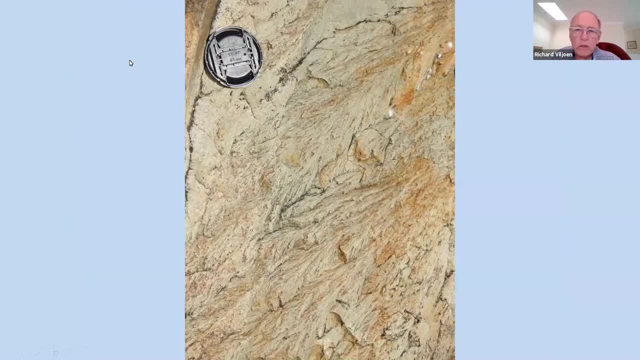 these incredible feathery-like cones of percussion, which are called the shatter cones, And those are caused by the impact of the meteorite, So attention is drawn to those. This is on the field trip And here are a variety of some of the structural features. 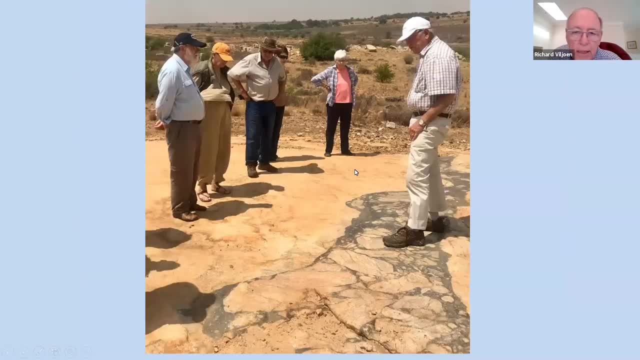 shown in a panel at Fierrefort And then in the field. another very important rock is the pseudotacolite itself, which is a melt rock which contains these large fragments. sometimes they're even rounded of the surrounding granite. 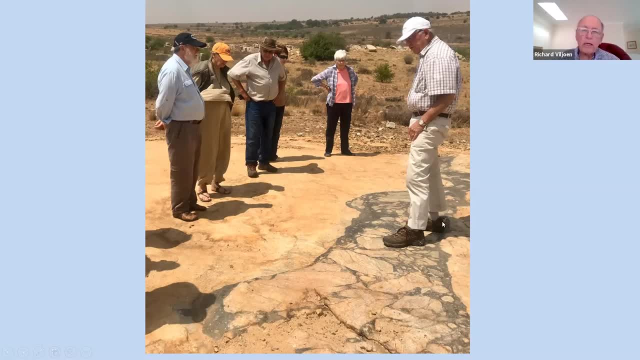 It's all granitic rock round about. So these things are plentiful within the dome area, particularly in the granite, and are sure signs of this incredible temperature and pressure that caused melting and the formation of the so-called pseudotacolite. Nikki, Oppenheimer and Strilli are looking on. 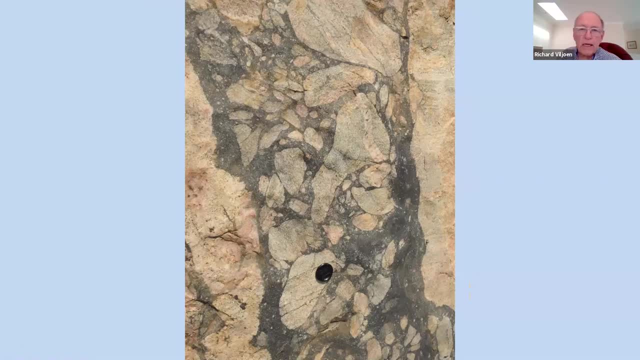 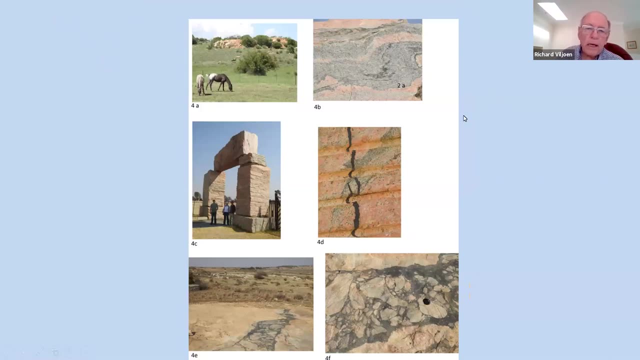 quite fascinated. That's an example of the pseudotacolite And roundabout examples of the pseudotacolite and examples of the perace granite, as it's called, which is also interesting. It used to be used as a building stone, called African flame. 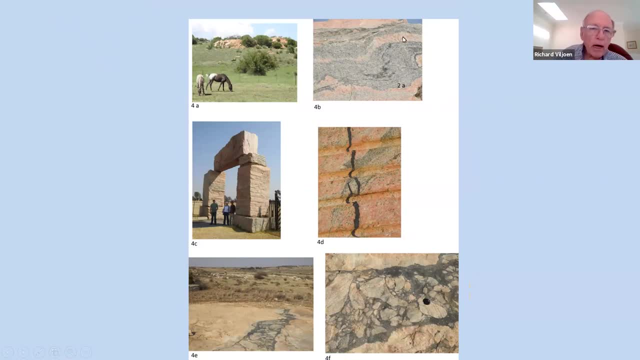 And you can see a gray variety and you can see a pink variety And then in the background you can see a typical type of granite outcrop And also the vegetation. here is the high felt type grassland which you see in the core of the dome. 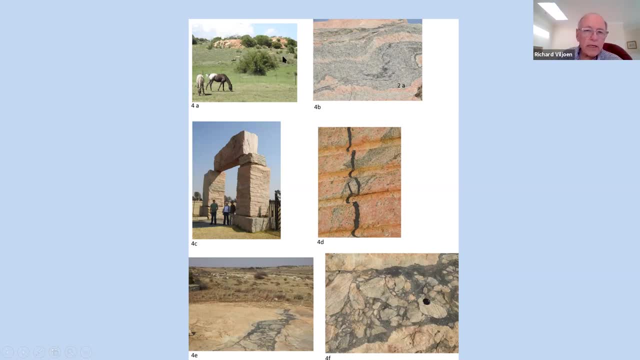 but you don't see in the collar rock. So again, the vegetation is dictated by the the topography and the geology of the area, And these are just some of the guest houses and places around the dome which cater for visitors. 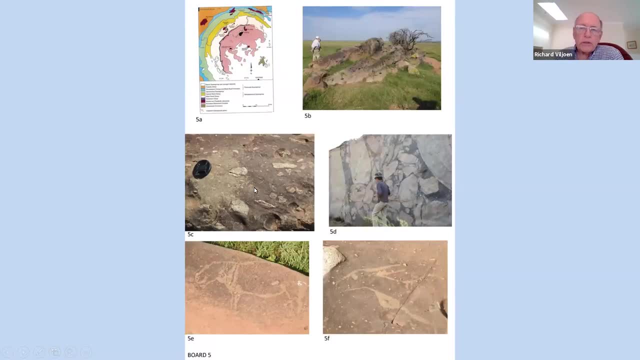 And then another peculiar rock type is the granifier, which is actually a melt rock. So the melt rock from, as you saw earlier, you saw this huge debris thing and from it emerged melt rocks which actually penetrated down into fractures in the granite and other rocks. 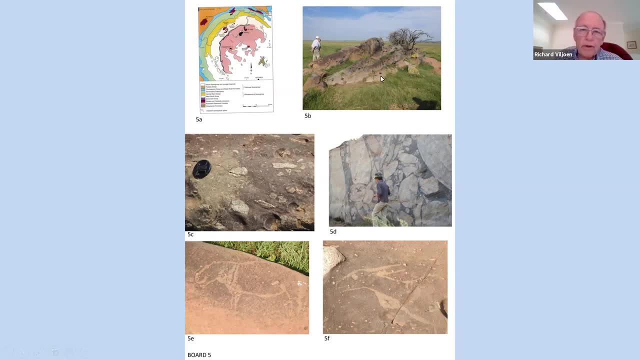 forming this peculiar granifier, which you can see over here, containing fragments of all sorts of other rocks, including quartzites, granites, et cetera. So that's another very important indicator of the of the impact itself. But this rock and another example of the pseudotachylite. 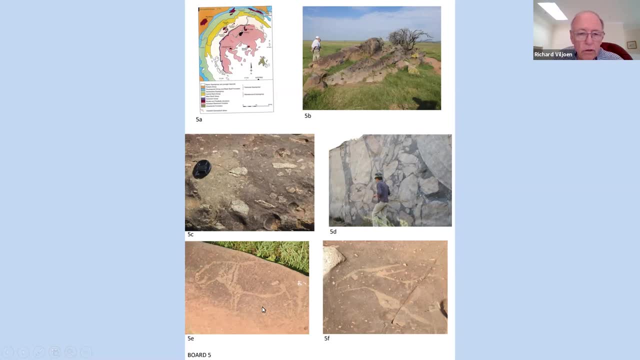 but in addition, it acted as a canvas for early artists, And these are the. these are the petroglyphs that are portrayed on these granifiers- fantastic petroglyphs and a very important tourist attraction as well, but based on the geology. 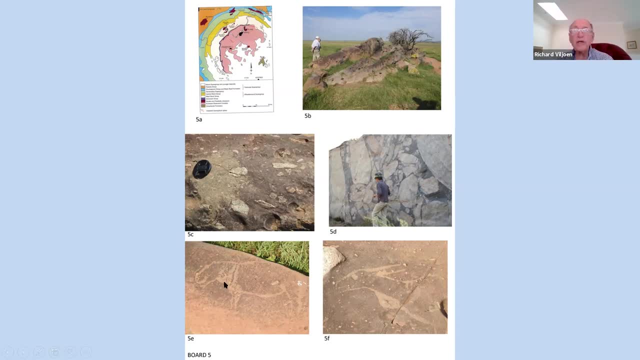 Without the granifier they wouldn't have had a nice little rock to do their engravings on. And this applies to other areas of petroglyphs in South Africa, particularly in the Kimberley area, as well. So that's another feature. 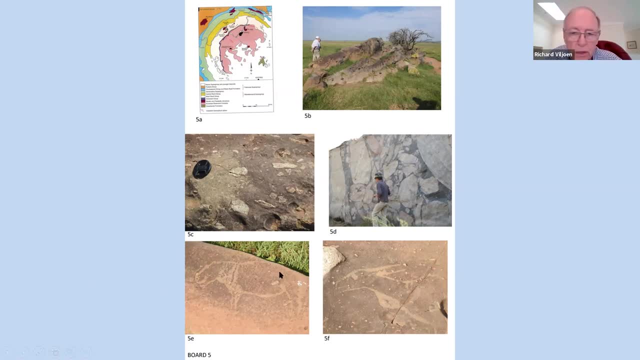 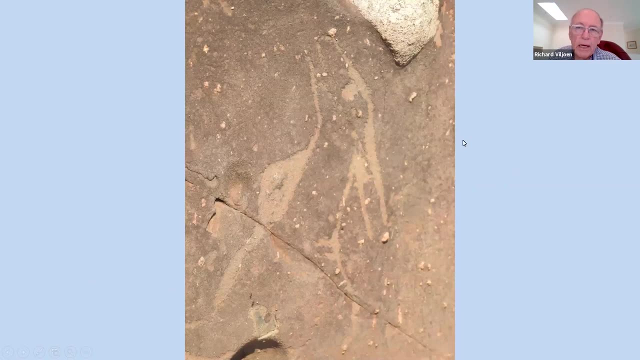 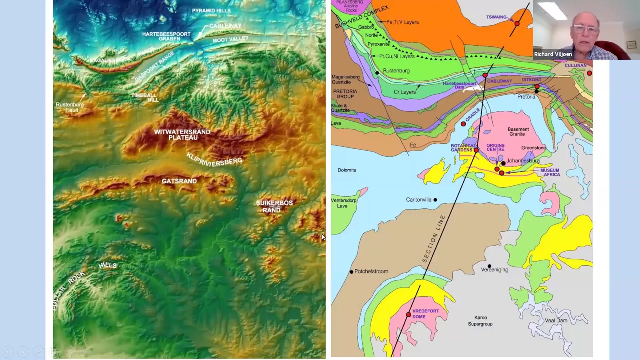 that can be looked at as an adjunct to the geo side of the tourism. Just an example of I think that's a giraffe over there and a rock fragment there in the granifier And then, as I mentioned earlier, the duplication of rocks. 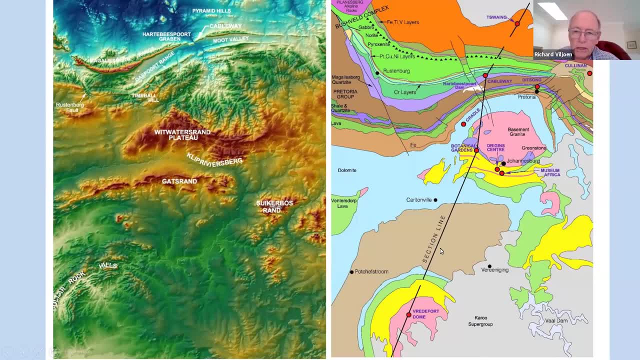 So if one looks at a geological cutaway, like cutting a section right through between the Phaedophore Dome and the and the Johannesburg Dome, one sees firstly the granite and then the first rocks are the are the Badgadisrant rocks. 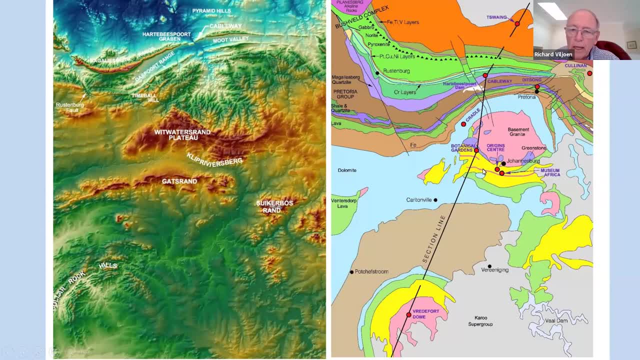 which occur here and contain the world famous gold reefs, And it's interesting to note, then, that the same rocks reappear here in Phaedophore, as I showed in that section earlier on, And the same applies to the larvas, which are duplicated here and here. 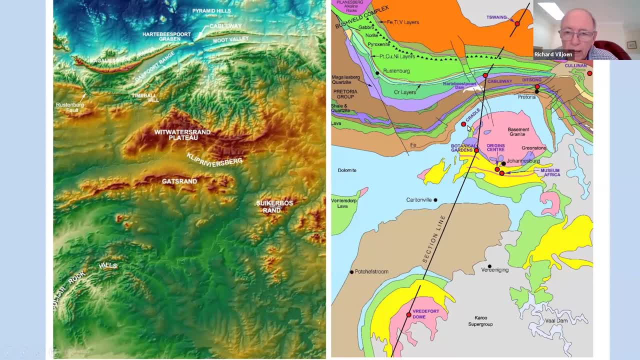 and the same applies to the dolomites, which are duplicated. There's the cradle duplicated there, and then around Phaedophore. So that's compelling evidence of how this huge uplift has taken place around Phaedophore. So if we then have a look, 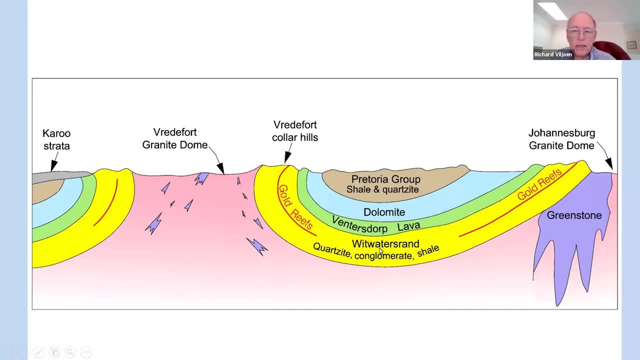 we can see how that works: The gold-bearing reefs of the Badgadisrant coming around upturned and outcropping in the Phaedophore collar hills, and the same with the larvas and the dolomites and the dome in the center. 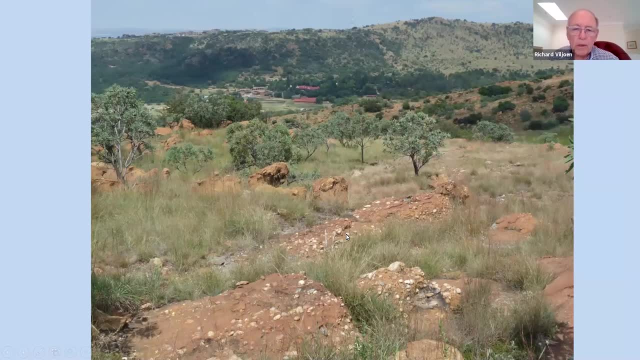 So these are the outcropping conglomerates just south of Johannesburg, in the Mondior Hills, And notice here again the importance of vegetation. Now you can see the typical sugarbush which grows on these acid soils of the Badgadisrant quartzites and conglomerates. 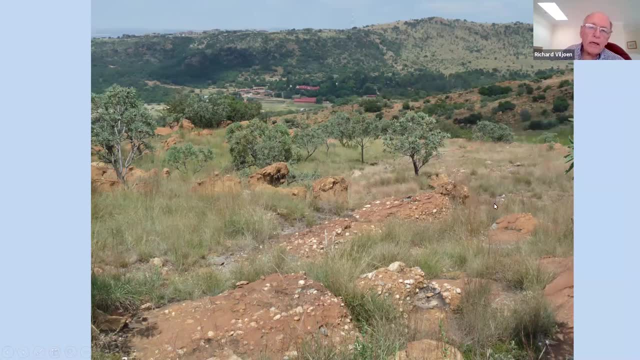 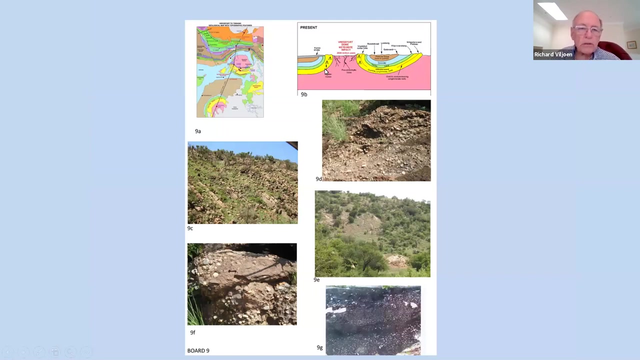 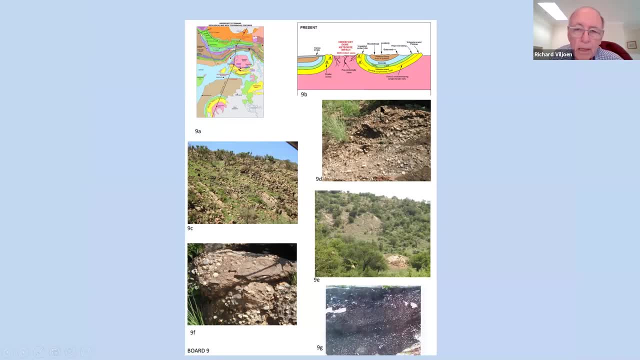 some court sites here. conglomerates are interlayered with them, Some of the conglomerates over here and another one there. And this was an old mine working. it was called the Felskuhn Reef And in fact it was quite a thriving gold field at about the same time as the discovery of 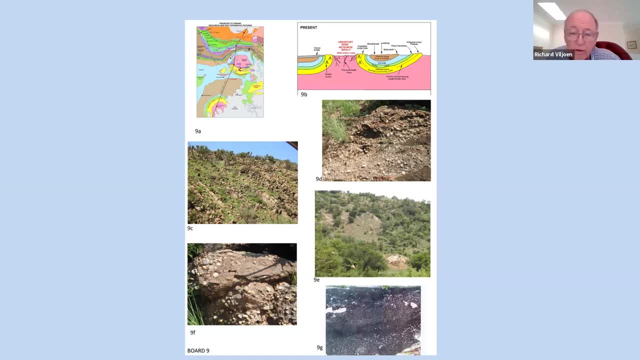 very soon after- I think it was in about 1887 as well- that this gold field actually thrived at about that time. So it's interesting that. but the gold grades, sadly, were not anything like those of the Witwatersrand and eventually mining was terminated. However, of late people are having 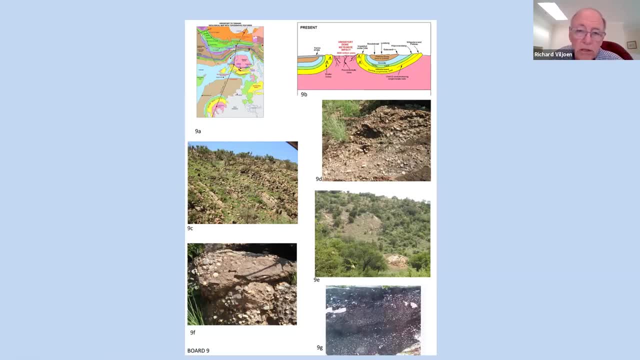 another look at it, But being a World Heritage Site now makes mining a little more difficult, And it's probably not worth it in the long run. And then, overlying the Witwatersrand, are the Fennersdorf Larvas. This is a lava with gas cavities called amygdales, And there you can. 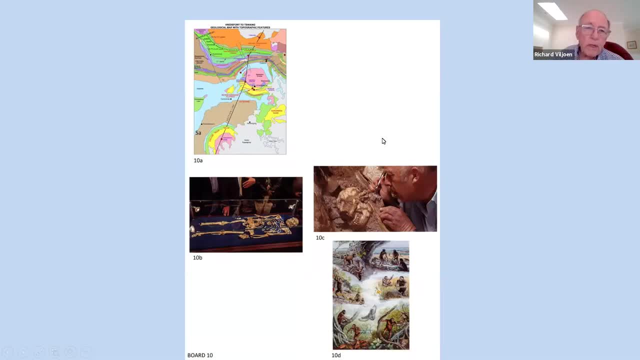 see it quite nicely. And then, of course, in the Dolomite Formation, you find the cradle of humankind. Caves have developed, And within the caves we get these hominid fossils, And this is an example of one of them, called Littlefoot. 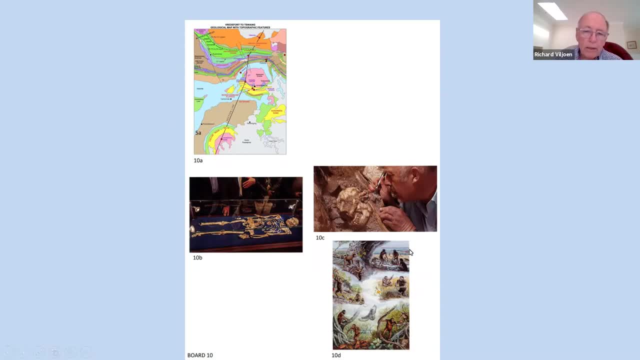 Being examined by Ron Clark over here, And then a depiction of how people lived at that time on the Dolomite Formation- I mentioned the Dolomites because the Dolomites occur around the rim of Fjordafjord as well, And a number of caves have been noted. However, no excavations have been. 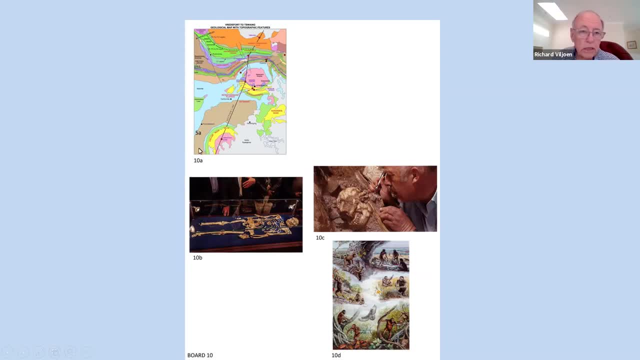 carried out, to my knowledge, or no major excavations and potential exists for finding hominid fossils. So there are all sorts of intriguing kind of side effects of this meteorite impact And this is the kind of story that can be told at the Fjordafjord Dome from the information center or from a video. 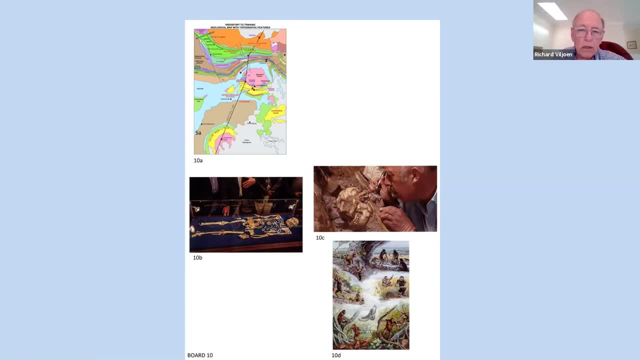 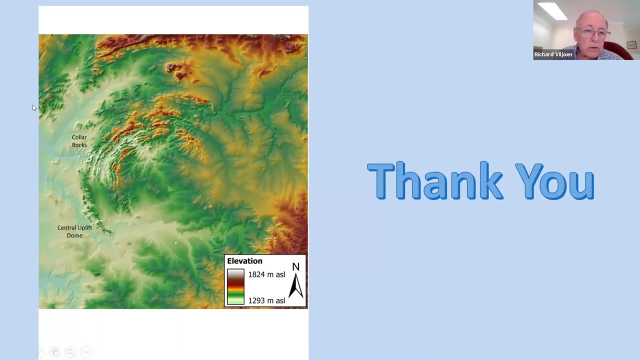 or whatever, But certainly it should become a major tourist attraction, which sadly it hasn't come up today. So we hope that this can change, together with many, many other sites in this country. So with that I will hand over to Morris And just another final image to a pretty 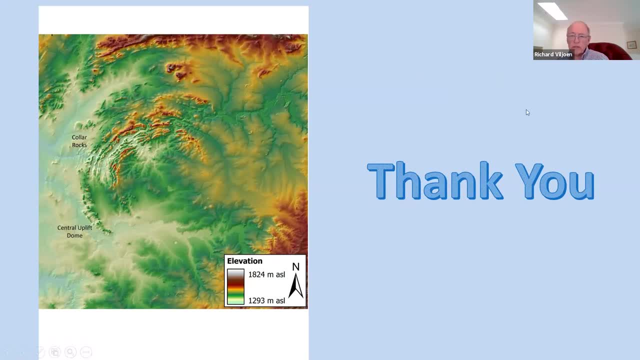 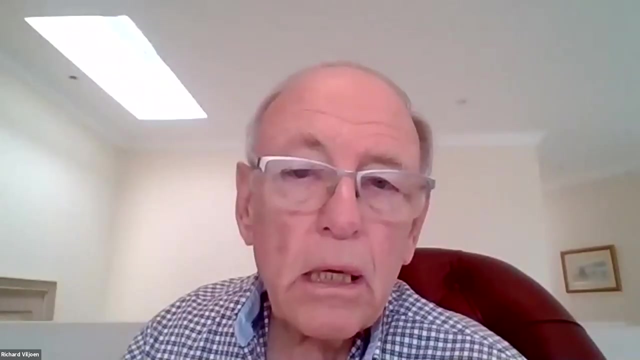 convincing one. That is quite a phenomenal structure. So thanks very much, And I think, Morris, if you could hand over, I must just get out of here, So I must share. you're sharing the screen. stop share, okay. so okay, Morris, if you can. 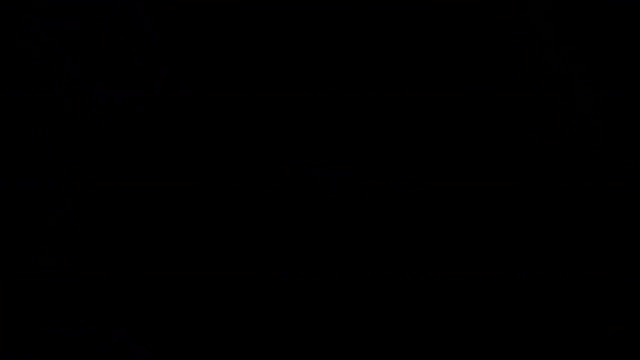 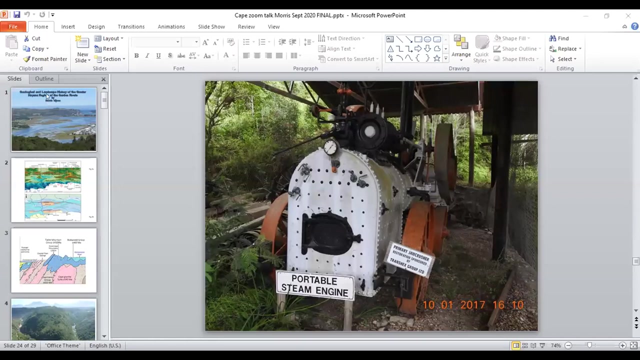 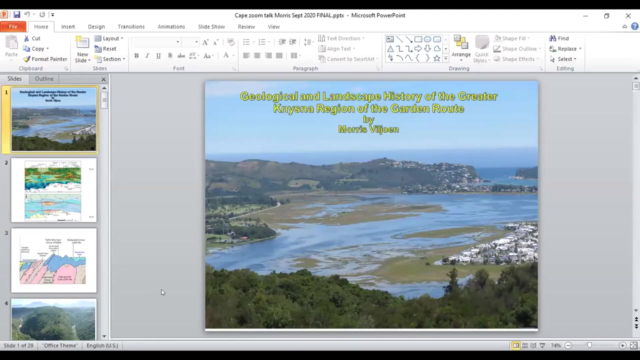 share your screen now and if you can get it into presentation mode, you're there. okay, that might be better. can everyone hear me now? hello, we can hear you, okay. yes, the presentation in the presentation mode, though is it not coming up on the screen? yes, but it must be full screen. 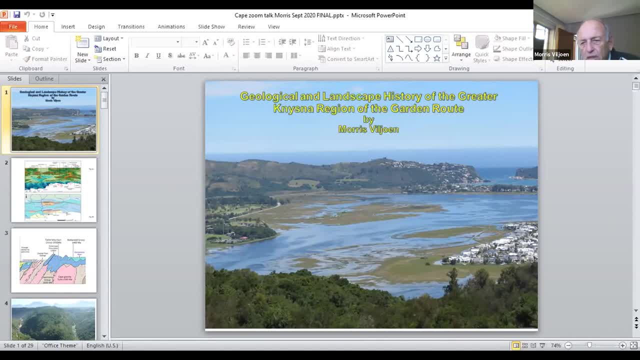 please put it in presentation mode. where do I get that? make it slideshow, slideshow. so if you take your cursor up a bit towards the top of, and then to the left, left and to the right and in the middle of where you were, this it says slideshow. next one to your right. there you go, there you go. 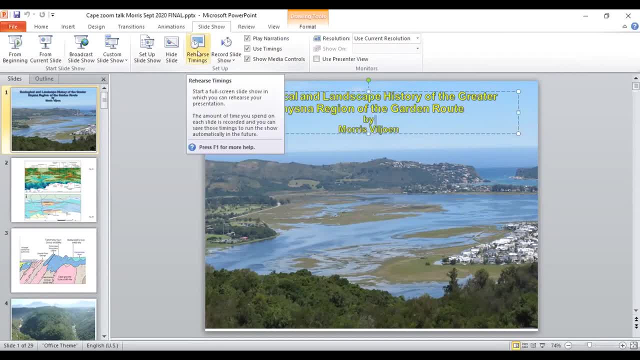 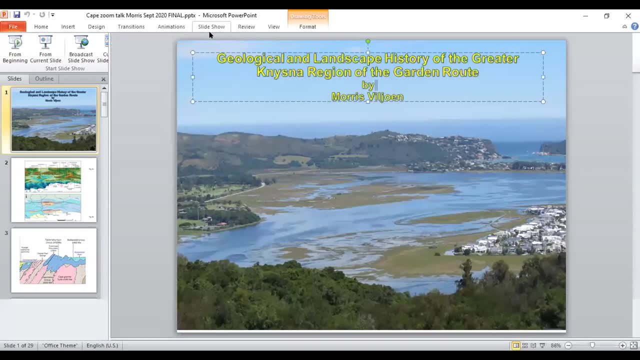 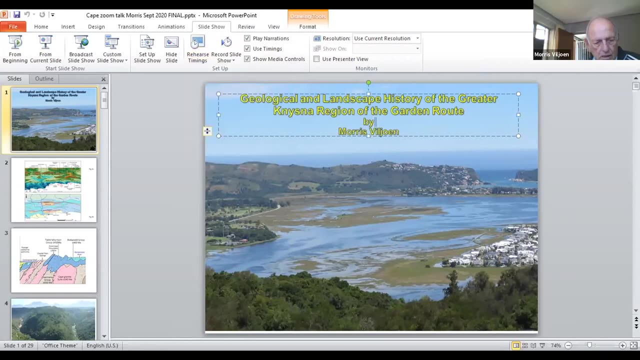 on that and click no slideshow. click on slideshow. it doesn't click. okay, it'll be easier actually if you go down to the bottom of your screen where it says 74 percent, and just to the left of where it says 74 percent. click on that little icon. 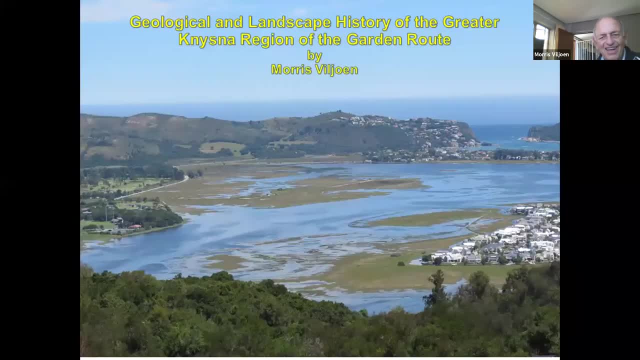 there, that's it, okay. you know how its' trouble is delicious thanks. thanks for that. okay, following up on what richard has just said, i'd like to give a brief overview of The Garden Route as a classical locality where geoharitage tourism can be developed. 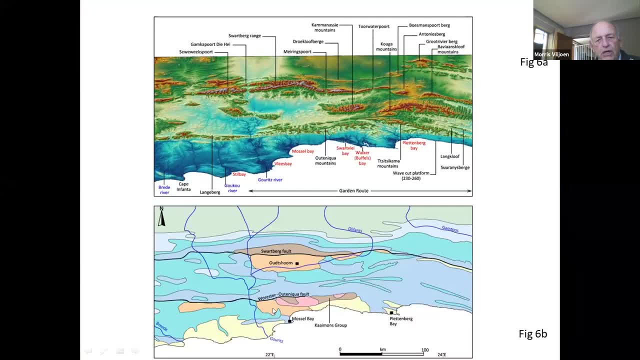 so we start in the Gnaıznar area, or was centered on Gnaiznar. it's the greater Gniazinter region and the things that one needs to portray and show about every case- and Richard has done that- would be essentially the topography of the area, because 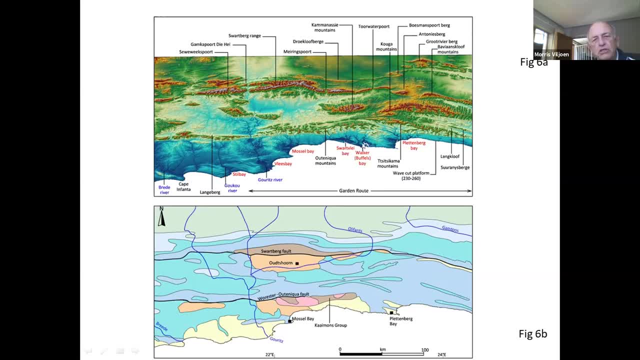 that's what people see, the landscape. so digital terrain image shows that very nicely. over here you can label the major features you know, for example the Otonequa mountains at Tsitsikama, and then over here this light blue is the coastal plain. it's a high standing: 260 meter high coastal. 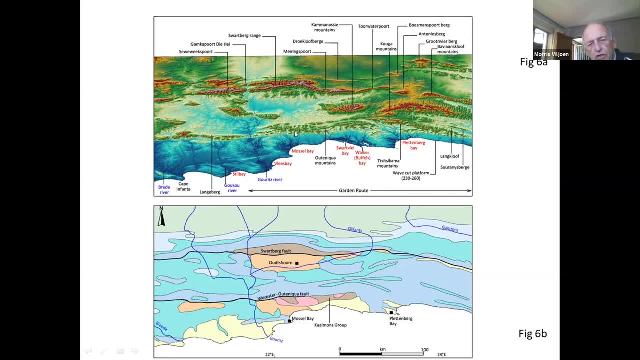 plain, cut by various rivers and the darker blue, and they cut and form different canyons and features depending on the rock type that they're cutting through. they all have the origin in the coastal ranges over here, so I'll be talking really about this region, the garden. 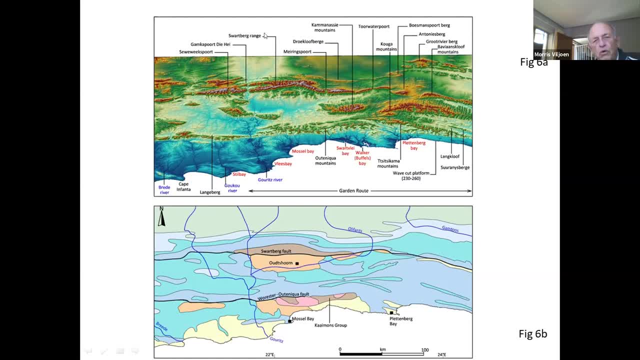 route, the heart of the garden route. there's obviously another big story inland, the Cape Fold mountain belt, but that's for another time. then one would compare the topography with the geology and then, very briefly, the. these harder rock formations correspond to the the table mountain group, which are hard court sites. this is, they've been amalgamated here. but 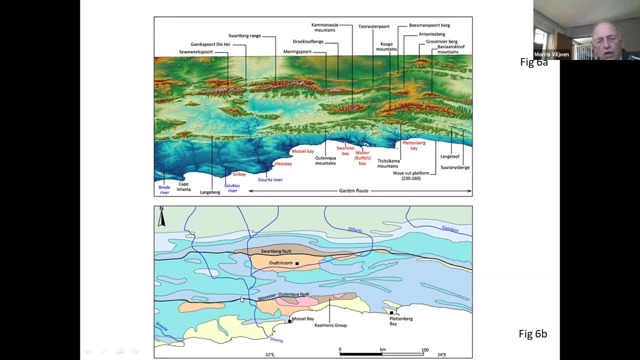 they're all essentially hard court sites and the valleys are underlain by, essentially, the Bokkerfeld shell, which is this turquoise color over here. in addition to that, there are a number of major faults and such as the Swatberg fault here and the Buster Otonequa fault, which have they formed during the? 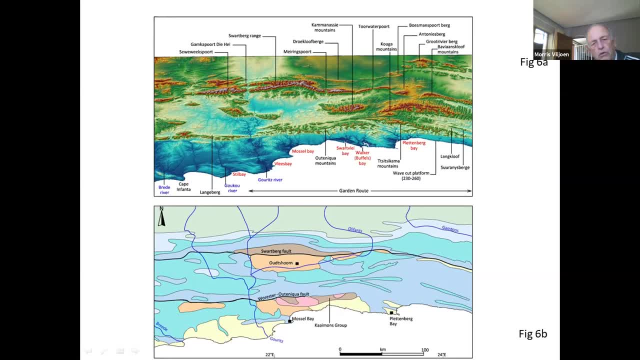 split of the Gondwana continent, and that's another story that can be told as well. but erosion from the up faulted northern side here resulted in big sedimentary, younger sedimentary basins being formed, such as the Otsoen basin and the basin here at Mossel Bay area, and and and many others. 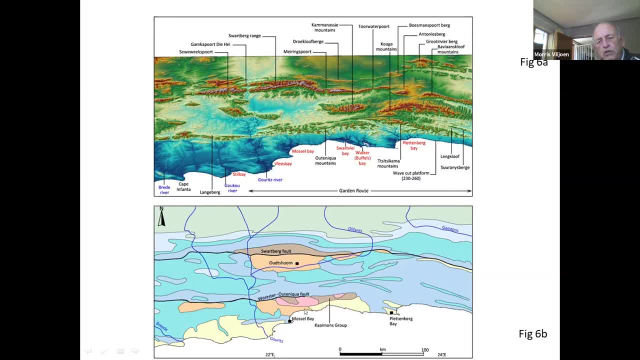 in the valley, over to the east and so on, and these consist of? consist of conglomerates, course, grain conglomerates, court sites grading into finer material. but as they get away from the active fault zone, so and then the oldest rock in the area, rocks in the area are exposed along the 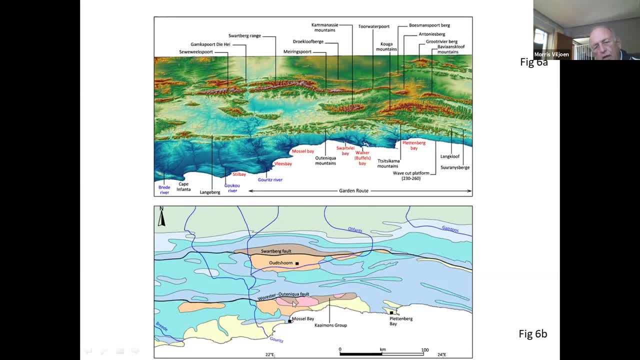 the Buster Otonequa fault and they consist of the the most ancient sediments: 600 million year old hills in the area of the야 and, so far, six traditional natural ravine. we can high standing wave, ancient wave cut platform, And then this is an example of the platform. 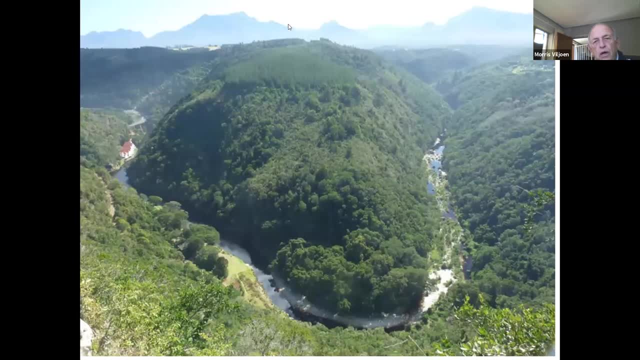 you can see here at this level, with the Otunikwa mountains in the background and a very well known tourist locality called the map of Africa, in which the Cayman's river has cut this gorge and all the way along it's cut through the Cayman sediments. 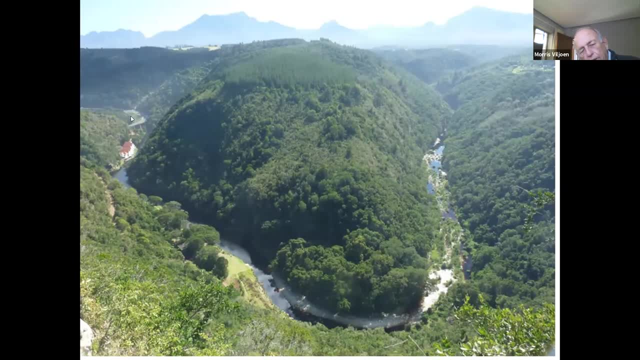 which are essentially ancient shale and sandstone- mud and sandstone- very well exposed to the Cayman's mouth, for example. but there are a number of localities where you can see good exposures of the Cayman sediments And this is a kind of gorge that falls fairly steep. 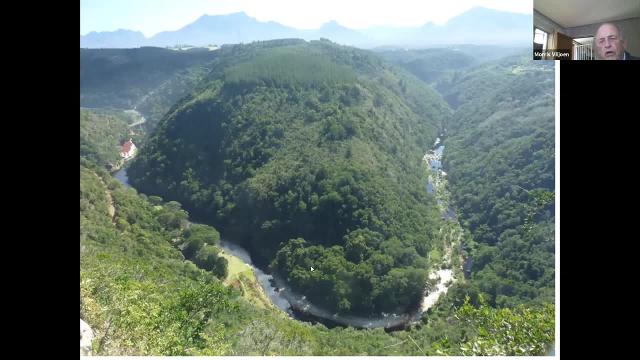 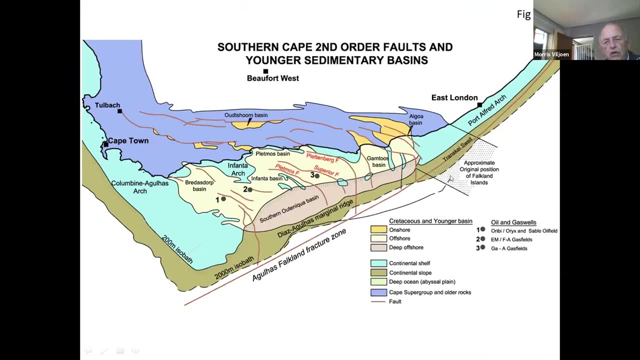 but it's not nearly as steep as some of the gorges cut into the harder rock, And this actually shows the Gullifalk Falkland's shear fracture zone and these second order structures that come off it, including the Otunikwa, the Otunikwa fault here. 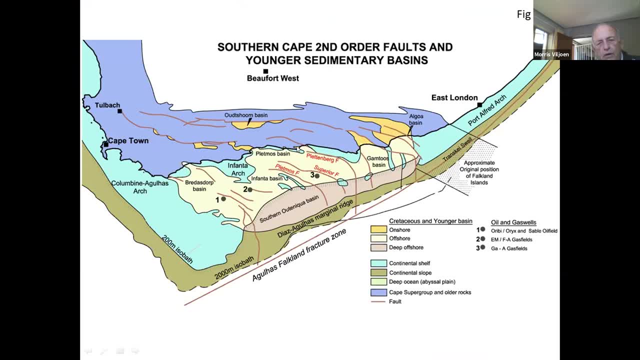 and the Booster Otunikwa fault along here that I've mentioned. And then this also shows offshore sediments had formed and of course they contain the gas fields, showing one, two and three of the some of the major gas fields off the southern Cape coast, on the continental shelf. 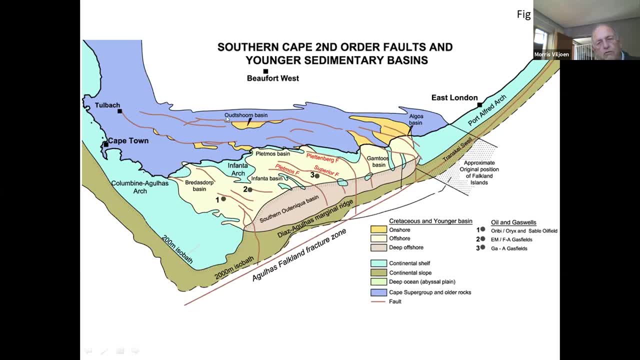 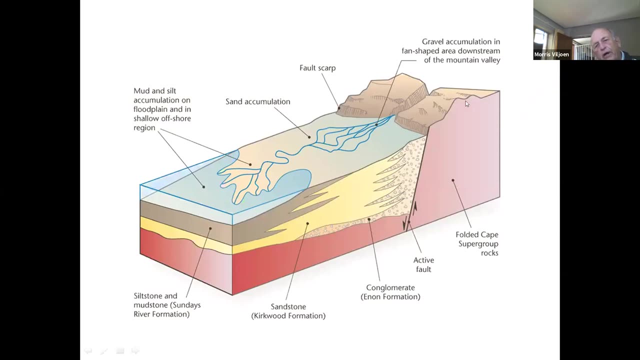 So this just gives that general setting of these faults developed when South America moved away from the African continent And this shows a diagram. So, once again, simple diagrams are important to portray features and this shows how you had erosion and the dumping of the coarse conglomerate close to the fault edge passing out into 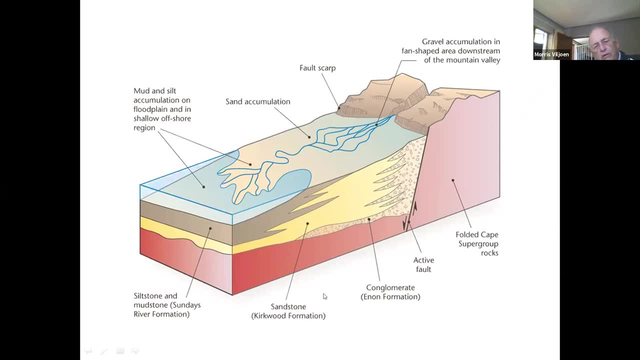 sandstones and then finer grain mudstones, And these formations have different names in different areas. For example, the Sundance River formation in the Eastern Cape would be these fine sediments And these are called the enon conglomerates in many areas as well. So that, in a very simple way, shows how 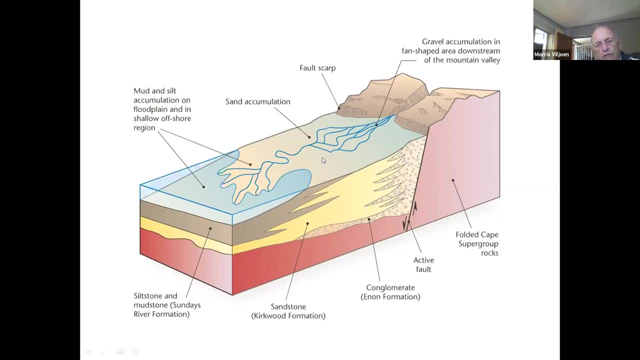 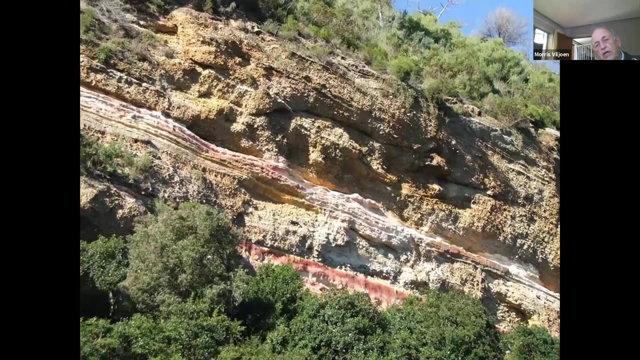 these younger sedimentary basins formed adjoining these big faults. And then you show examples of the material. And here are some classical exposures on the northern side of the Knysna estuary Where you can see very good exposure of conglomerate and very nicely colored. 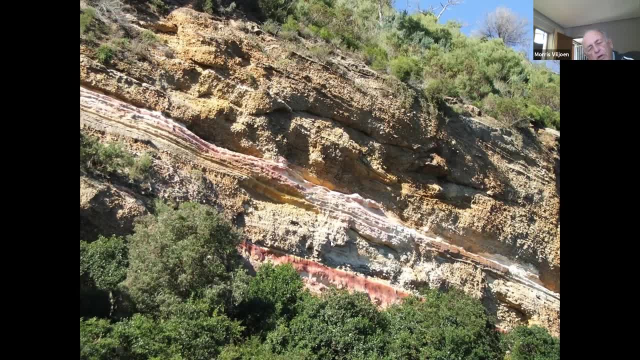 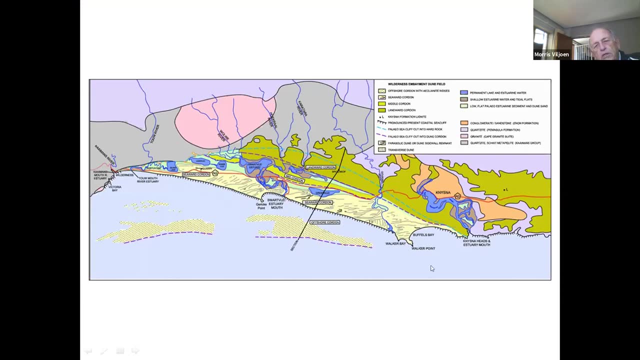 sandstone and conglomerate, basically, And a number of localities very well exposed. And then the other feature that occurs much younger would be a series of sand dune cordons occurring within an area called the wilderness embayment, extending from the wilderness over here towards Knysna over here. 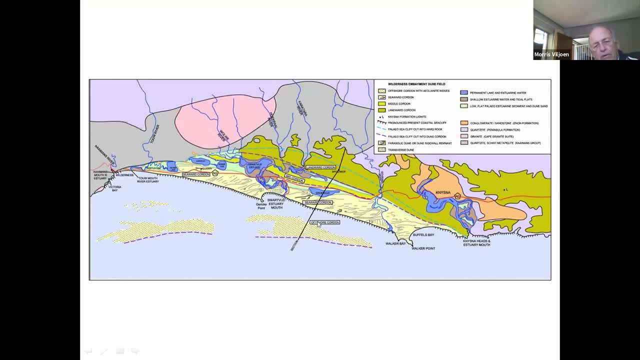 And a number of people have mapped these. There's a hidden sand dune cordon here as shallow as 10 meters below the ocean. here You then get the coastal or the seaward dune field, The middle mid dune field over here, called cloud nine in the 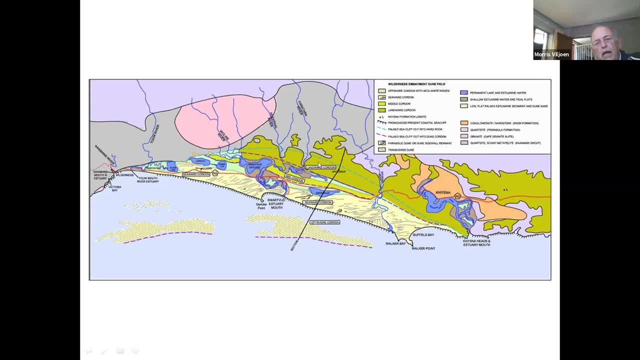 said field area And then the landward sand dune over here. That's the oldest one, I think that's probably about 750,000 years. The coastal one is 120,000 years And it is overlaid. Incidentally, these are generally calcified, the older ones. 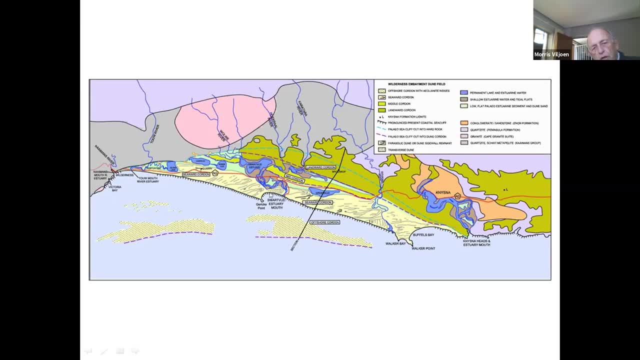 And classically exposed all the way along the coast. here are these calcified wind blown dune rock material forming the sea cliffs, But they're pretty unstable sea cliffs, as I'll show you, And they, in turn, are overlaid by much younger wind blown. 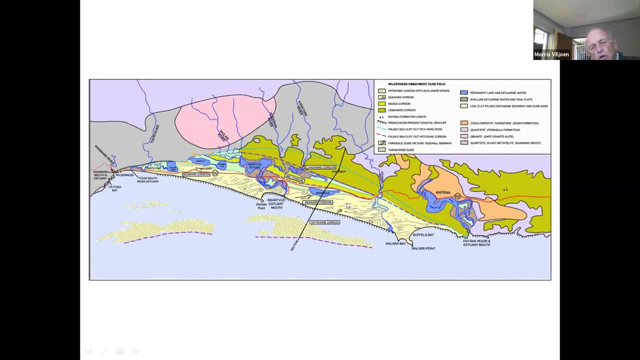 sand less than 6,000 years old, shown in light yellow, and forming these classical parabolic sand dunes. And another feature would be: in between these dune cordons, a number of lakes have formed, And this is due to the fact that the rivers 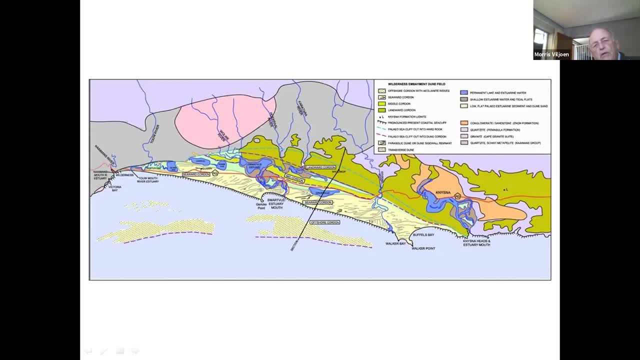 cutting gorges into the harder rocks. once they hit the softer sandy estuarine, the old estuarine and sand dune areas, they start spreading out and meandering around and spreading sideways. So you get these huge meanders Eventually forming big estuaries like the Swatflay estuary estuarine sediments. 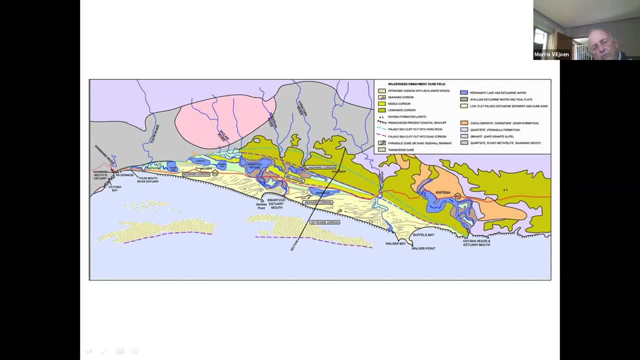 And rivers go nowhere really. They just meander around until eventually they find a gap to the sea. And the Knysna estuary would be a similar phenomenon: big meandering channels cutting sideways rather than cutting down, as you find in the harder rock. So a classical control by the. 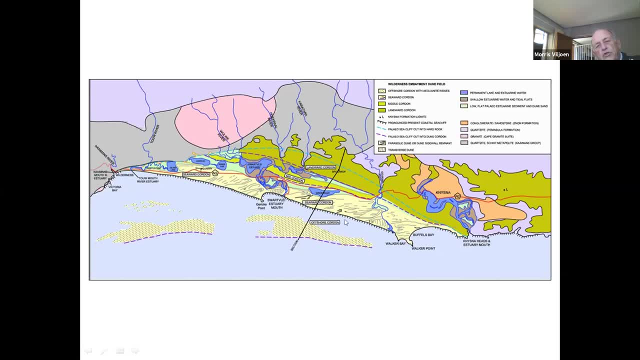 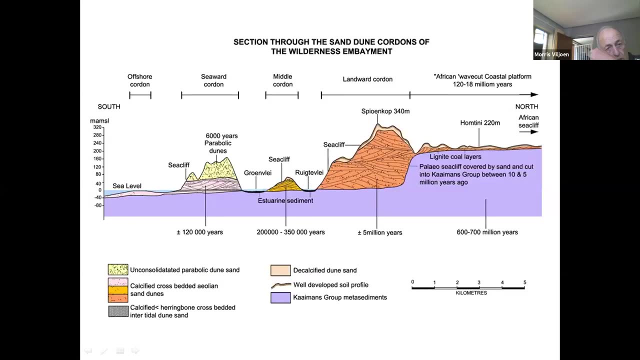 sand dune, cordons of water, And then this is the lake district of the garden route, And then, once again, it's always important to show a cross-section, And here is a cross-section of what I've just shown you. Here are the 120,000 year old calcified dune rock, beautifully exposed along the coast here. 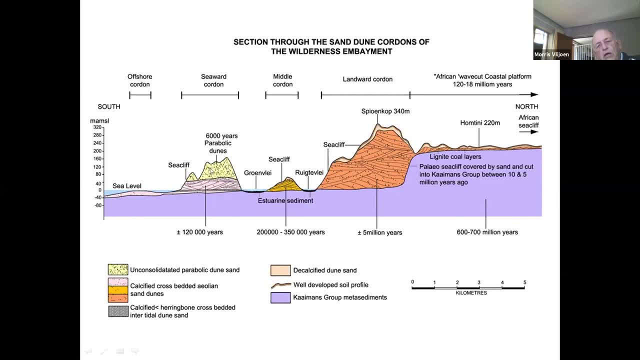 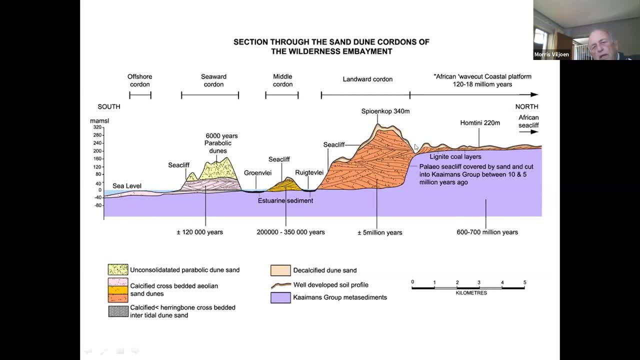 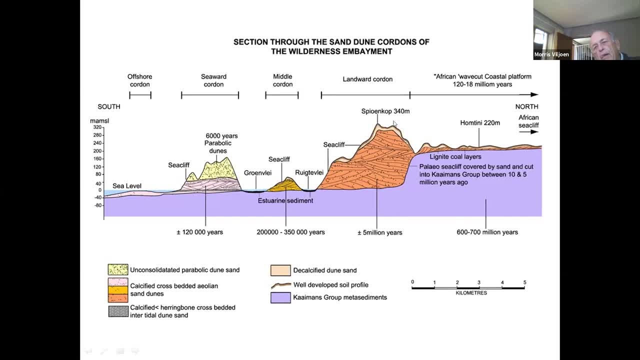 And this is where you see a lot of forest growth. A lot of forestry in the area grows on these dunes because you've got a reasonable soil. Over here on this there's hardly, there's no soil really- And you get a scrubby kind of coastal type of fine balls of grain. 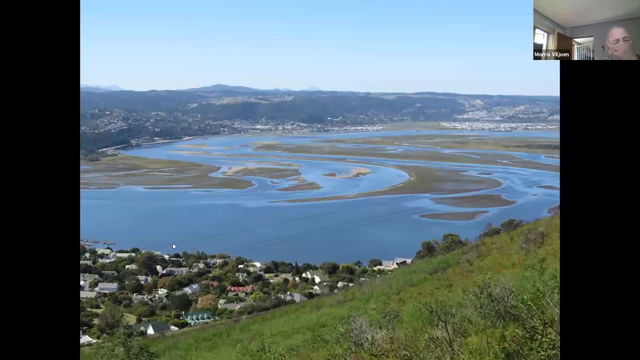 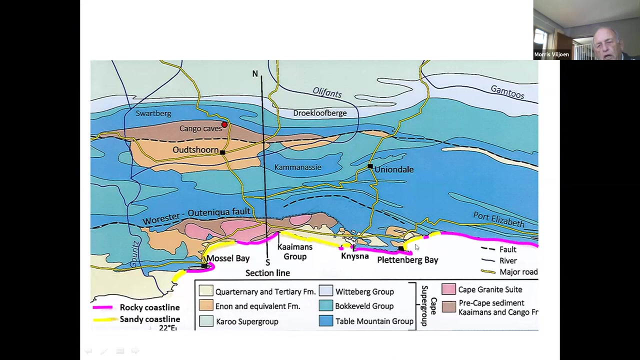 And here you see the Knysna estuary, with classic examples of the meandering nature of the river system, cutting sideways into the less resistant formations over time to form a broad estuary. And then, if we have a look at the actual coastline, it can be divided up into essentially rocky coastlines, for example from Plettenberg Bay to Knysna, sandy coastlines, Knysna to the river. 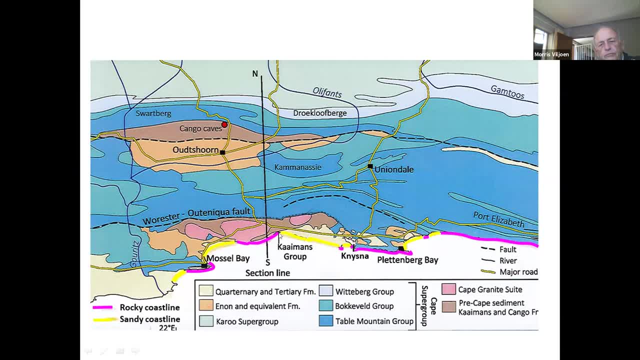 To Kiamans And another rocky coastline along here, and then sandy coastline again. The sandy coastlines occur where you have softer rocks and where these embayments were able to form and sand was able to accumulate, such as this Mossel Bay embayment. 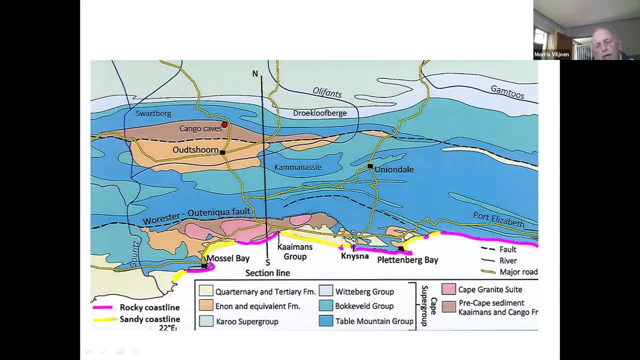 And Fliers Bay embayment over here and the Plettenberg Bay embayment over here. All of them have hard rocky, prominent trees or these hard rock formations such as Capes and Blades over here and the Rohrberg Peninsula. So it's then it's a matter of the kind of formations that one sees. 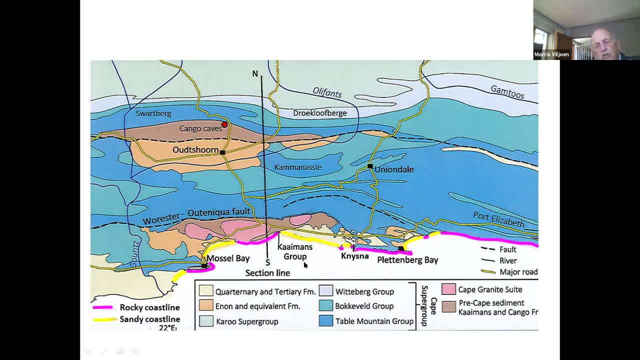 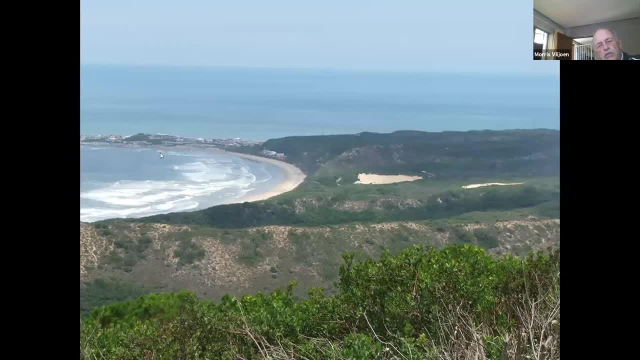 along these hard rocky coastlines as opposed to the sandy coastlines- And here is the Biffles Bay embayment- There is a hard courtside spine, really quite narrow, overlaid by classically developed parabolic sand dunes. These are the younger sand dunes overlying some older calcified material, but dominated in the 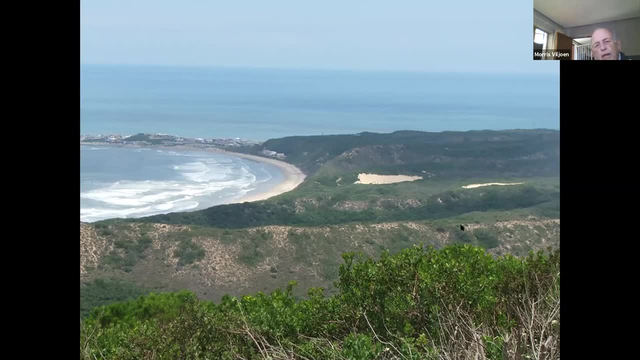 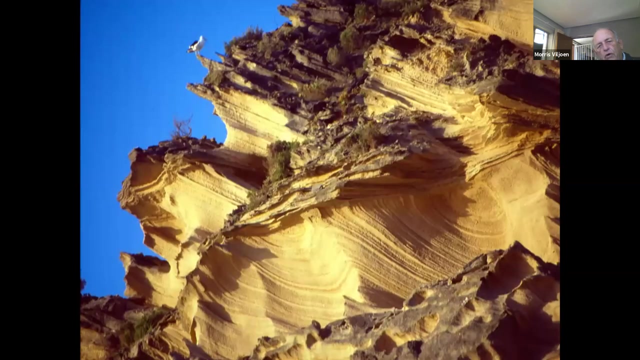 Biffles Bay. this is Biffles Bay over here, dominated by these parabolic dunes, And then these classical beaches form in these areas where there's softer rock formations, And these are now some of the examples of the calcified dune rocks that you find, for example. 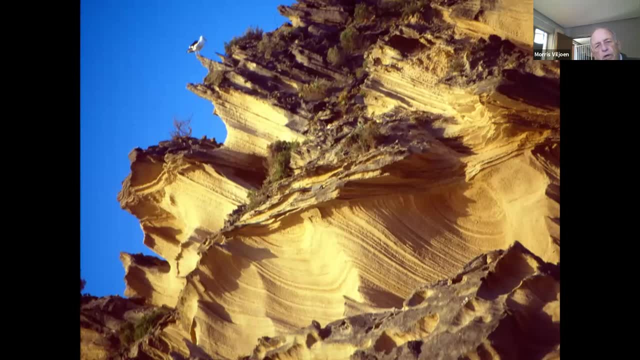 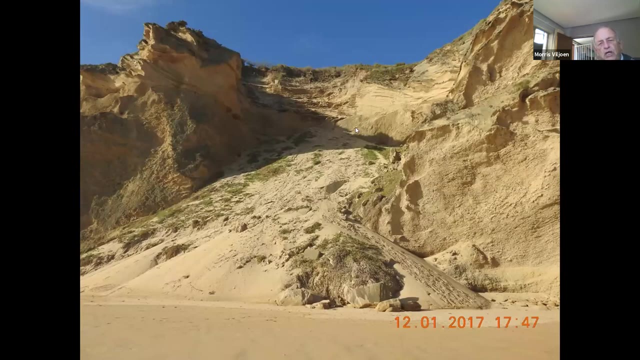 at places along the Sedgefield coastline- Plotterbunk- this is Classical calcified Aeolian sand dunes, And but then you also see this phenomenon here- And they're not evenly calcified, so you get weakish areas not quite as calcified. 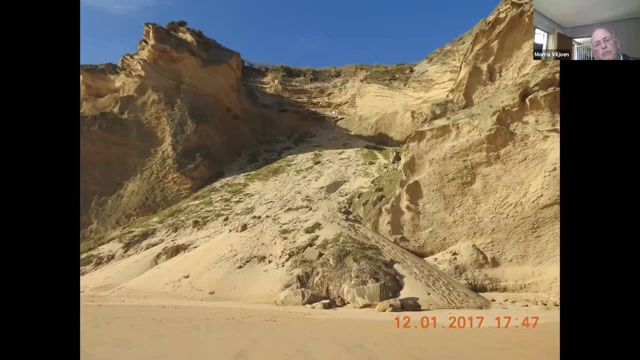 And these often just collapse in the form of massive landslides- This one happened only about two years ago, in fact- And this whole mass of sand and material, this is called the Biffles Bay. The sand and material comes down, and this, obviously, then, is the source material of the sandy. 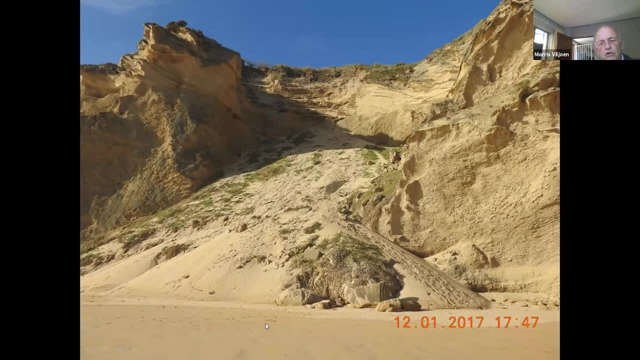 beaches, the sandy beach that forms over a considerable distance here. These are calcified dunes, more calcified, less calcified and forming this major landslide. Incidentally, about, probably about- six months ago, I went here with Willow Steer. 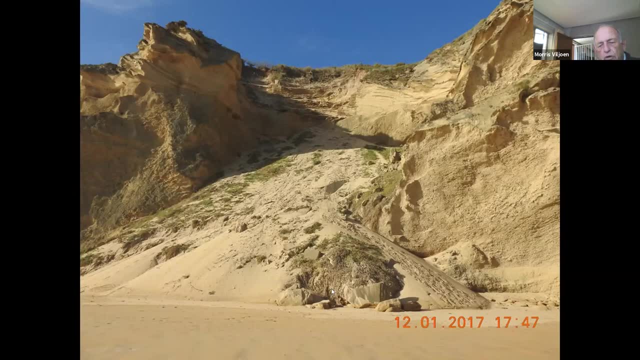 and one of the things they're finding in these 120,000 year old calcified dunes are human footpaths, Human footprints and animal footprints, And on a slab of rock- here I don't have a photo of it- we actually found 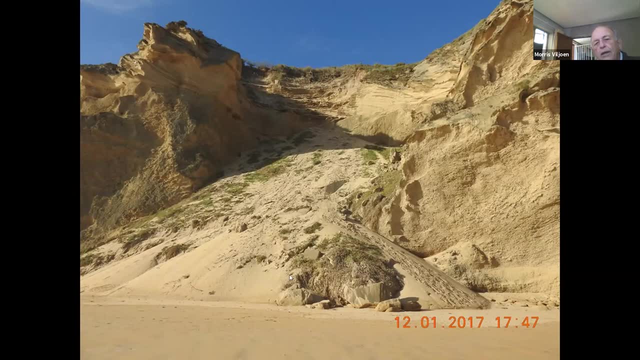 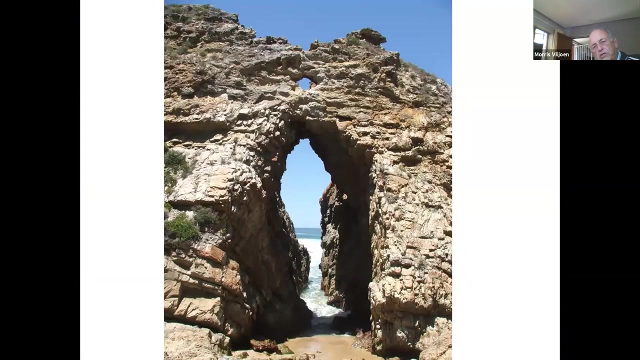 some classic examples of animal footprints in this 120,000 year old calcified dune rock, in a nice slab which is exposed in this area, And then, when you get to the rocky beaches, it's really difficult for erosion to eat away. 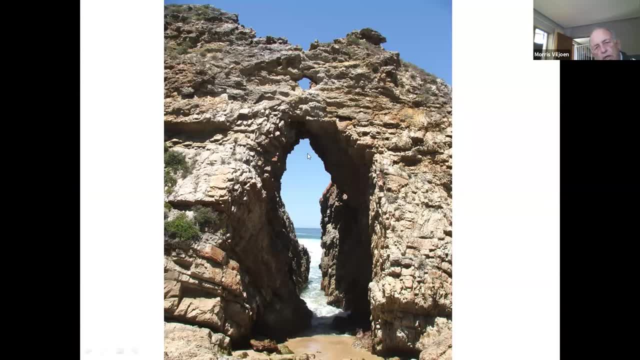 at the hard quartzite. So what you need is a weak zone and here we have a fault zone. it's a fault breccia and a fault zone and it runs. it's vertical and you can see that's been preferentially. 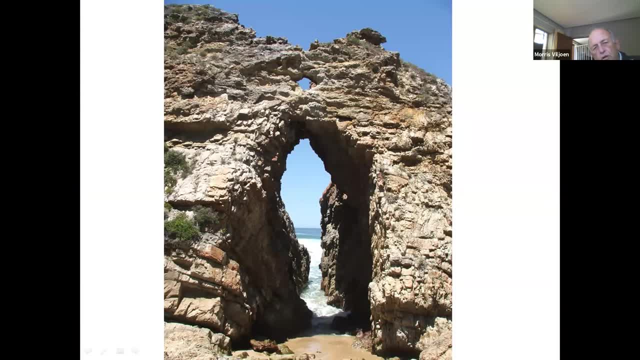 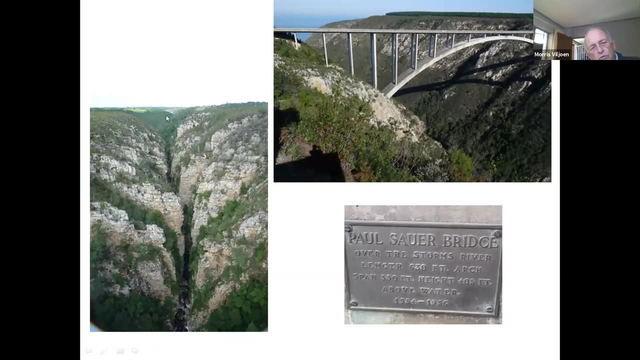 eroded and for it to form the arch rock on the west side of Keobooms Beach area. But classical control of structure, controlling the formation of this feature. A very similar feature, a feature formed in the same way, would be Storms River. 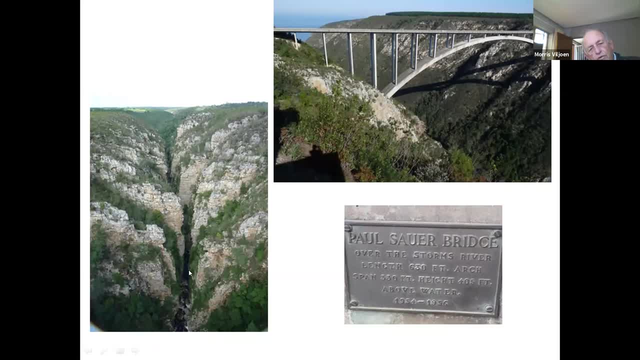 which is an incredibly narrow gorge- very deep, very narrow- where the river could only cut down. I mean, cutting sideways into the hard rock wasn't an option. And another example is Bloekrans- over here, the Bloekrans Bridge, and this is also a world-famous. 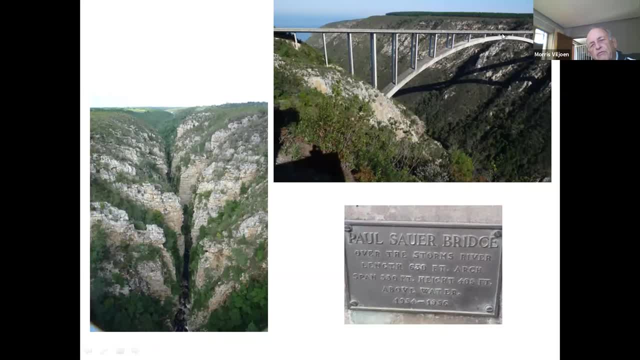 bungee jumping locality from this point over here, so in fact it's the highest bungee jump in the world from a bridge. It's, in fact, 260 meters. It's 16 meters high, the bungee jump, and so it's a very popular locality. 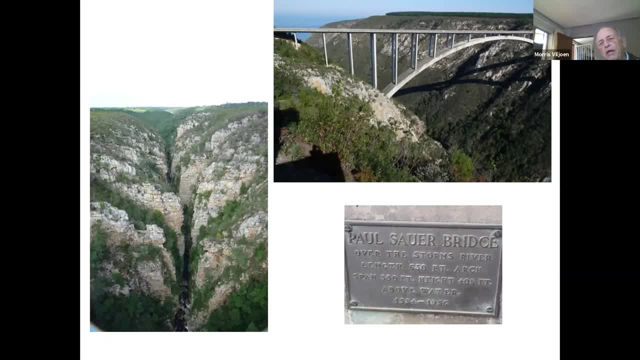 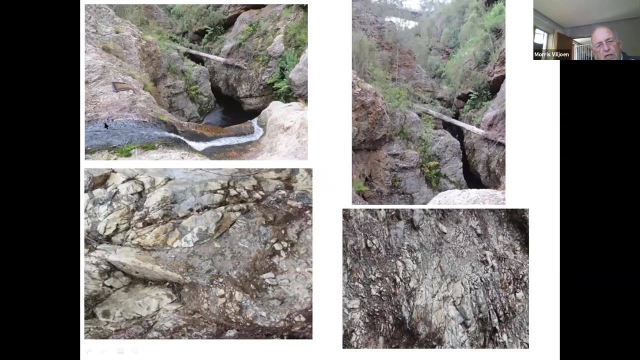 So this whole geology and landscape has spawned this adventure tourism locality, and there's quite a few others of these, In fact, one of them here is a place called Afri Canyon, and you can see, here this canyon is formed and you get people, many, many people coming along to do what is called canyoning. 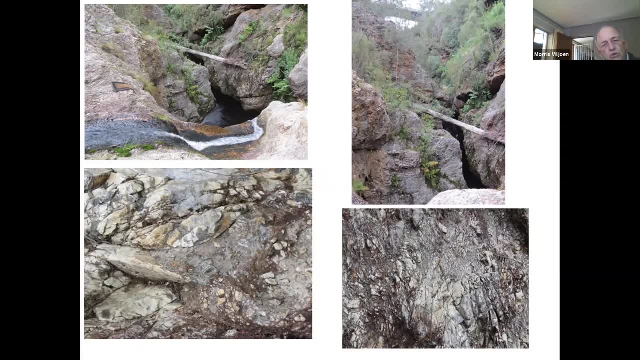 by jumping into the pools, swimming, abseiling, you name it- going down the canyon. But the owners of the canyon realized that there was an interesting geological control to this phenomenon and they wanted to tell people about this. So, for example, you can see classical fault breaches and this kind of thing. so we actually 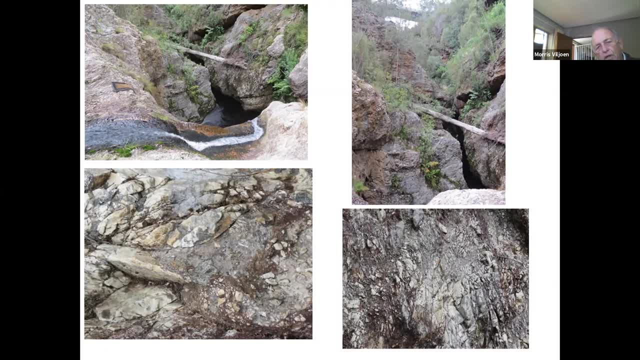 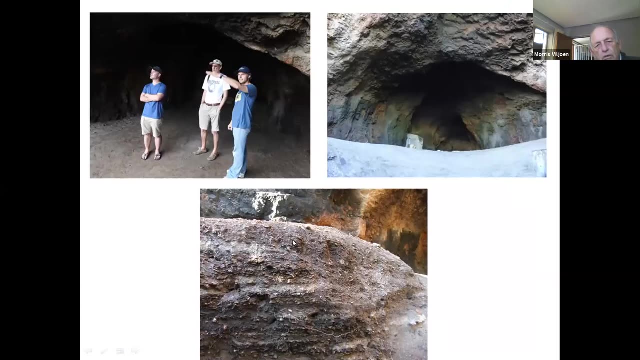 put up. we've designed a complete display along the lines I've been talking, but focusing in on how this canyon actually formed. So that's the kind of thing that could be done as well at other localities, And then if we just go back to, let's go on a bit. yeah, another fault area, yeah, here. 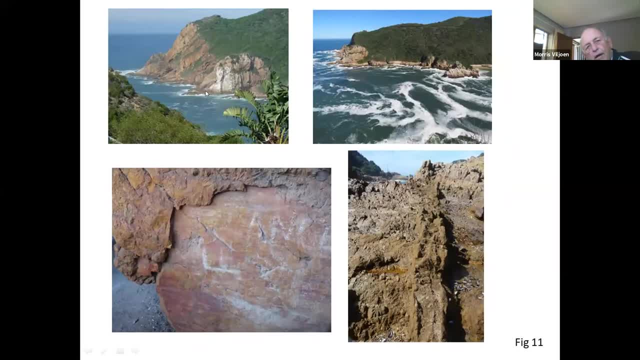 let's just have a look at this here The Knysna heads, the courtside, started deep seaward. but look at these vertical features here. This is a series of vertical faults and breaches, And these were relatively weak compared to this hard rock, undeformed hard rock here. 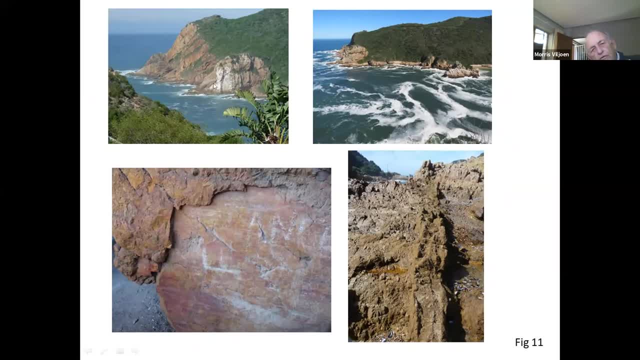 and the sea is bashed away here along these fault fractures and so on- to actually open up the Knysna heads gap, which is highly unlikely given the incredibly hard nature of the courtsides on either side. It's just due to this weak zone epitomized by the umpteen fault features. 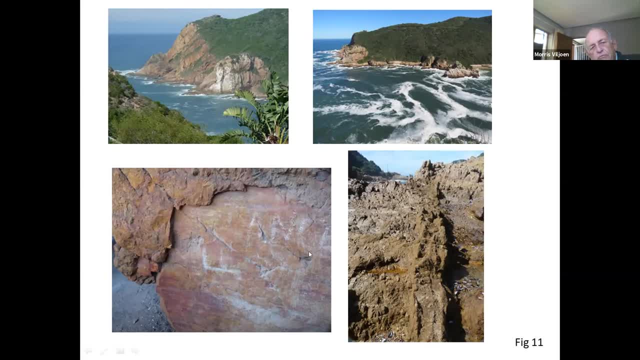 So yeah, Yeah, Yeah Yeah, Fault breaches and features like this. Here you can see some classical slickensides: fault breacher next to it, they're all over the show And those have been preferentially weathered to eventually give the gap which is the. 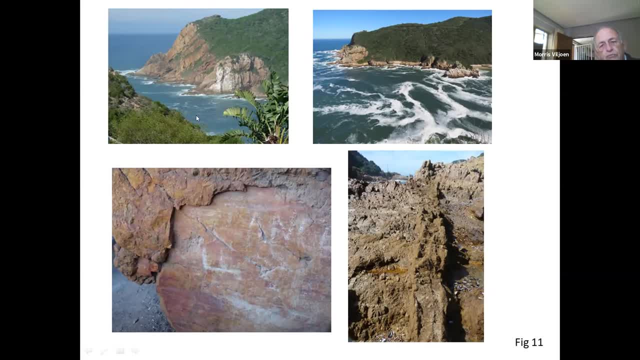 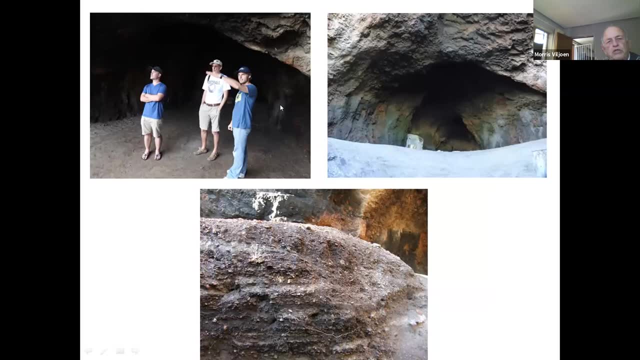 Knysna heads gap between the eastern and the western heads, And we are showed the slickensides right next to that weak zone, as well as being eroded to form a cave. This is on the eastern side, on the east, On the east heads, and this cave is about 130, 140 meters above sea level, cut by earlier. 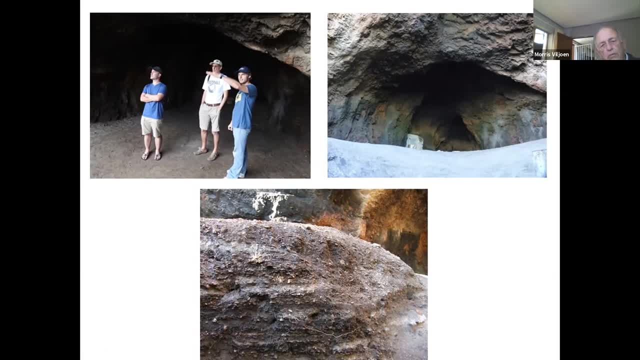 sea action, when the sea was at a higher level and then became a midden or dwelling place for early people. And here are some of the debris that occurs at the base of this midden and, interestingly enough, this was excavated. 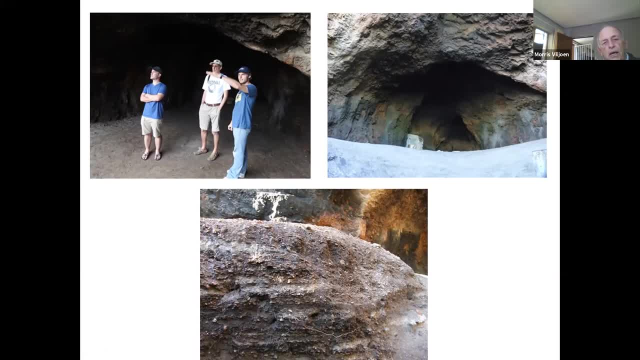 In 1880 by Thomas Bain, and he actually lived in Knysna when he was building a number of the famous passes in the area. Anyway, he found the numerous artifacts, including what he described as artwork on a scapula of a lion, and it's got quite a history. here it is and it's now considered to be the scapula. 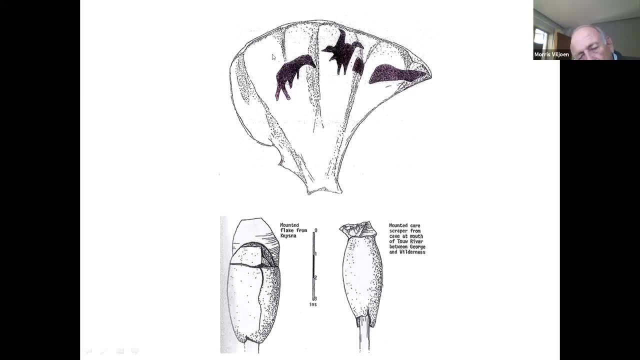 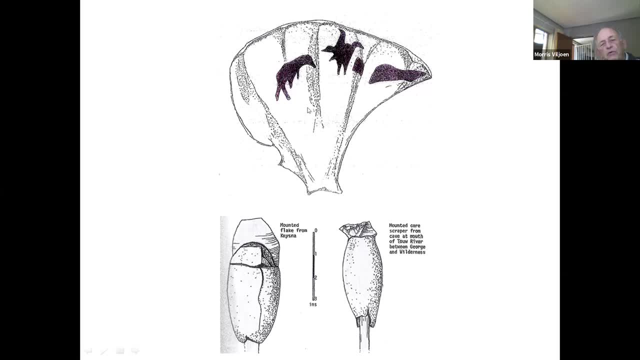 And this scapula, for example, was sent overseas in the early 80s to a big international exhibit in London, and on the return journey it disappeared And about in 1880.. In 1886, somebody called Thomas Headley appeared with this and he offered it for sale to the. 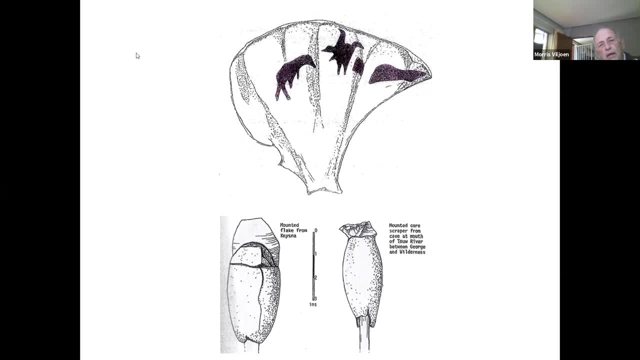 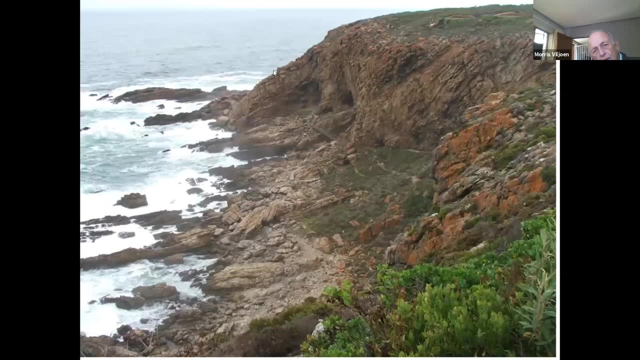 British Museum And in fact that's where it sits now. It's called the Knysna Scapula in the British Museum. And another really famous locality now is called Pinnacle Point, a hard-caught site but with these quite high-standing caves. 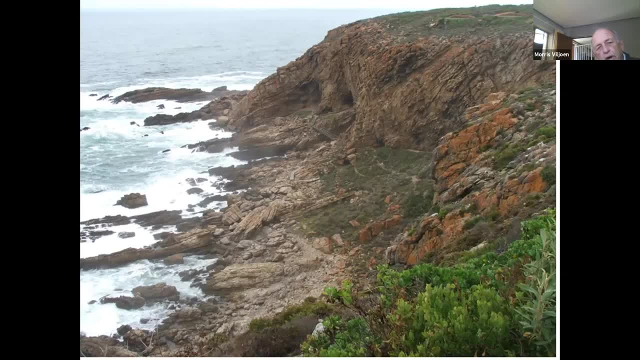 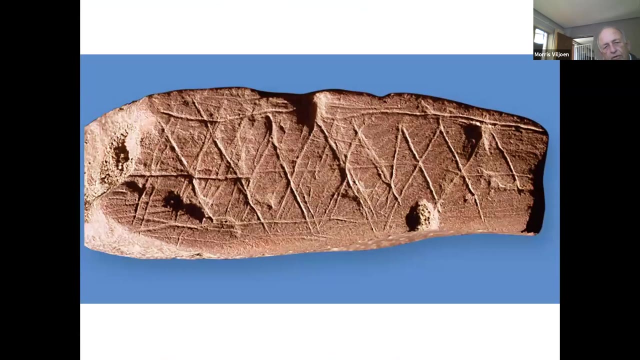 And this is where excavations by Kurt E Curtis, Marion and others have shown the existence of early humans- the earliest humans known, actually 160,000 years ago- who were doing human-like things, And this is considered to be a human-like activity as opposed to, maybe, an ape-like activity. 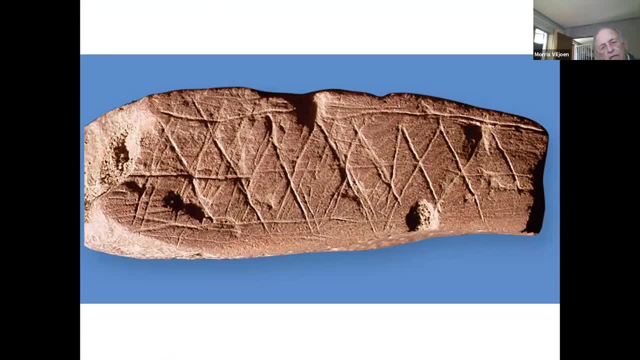 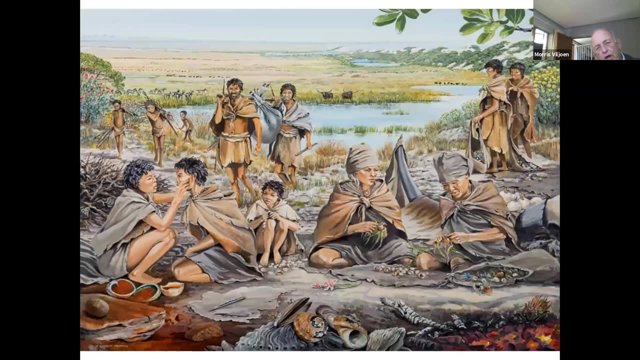 and that is the deliberate carving of a chevron pattern onto a piece of ochre. And then, once again, it comes back to trying to portray what was happening at the time, and this is where Maggie Newman comes in again, And she did this excellent painting of the scene when the sea was at a much lower level. 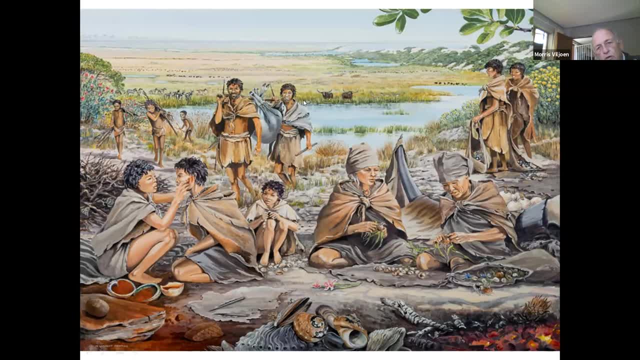 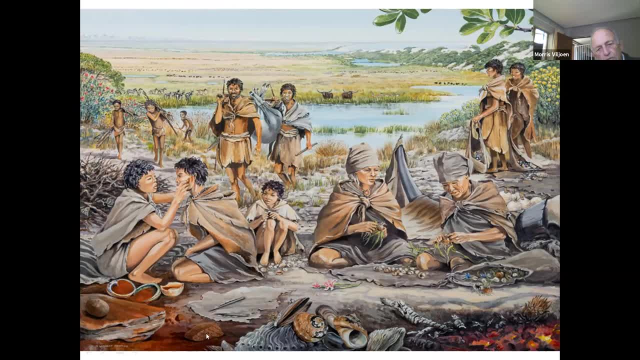 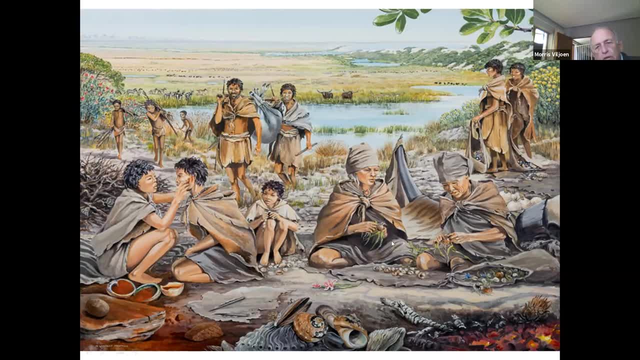 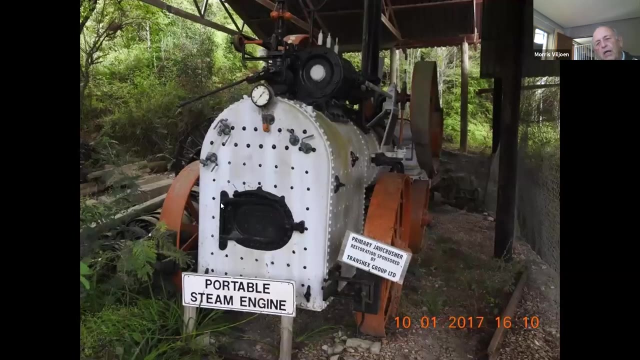 And they were eating seafood as well, so that the sea was close by, and so on. So it depicts the kind of activities that can be deducted from the artifacts found in these caves, And then one can go on to the mining story as well. 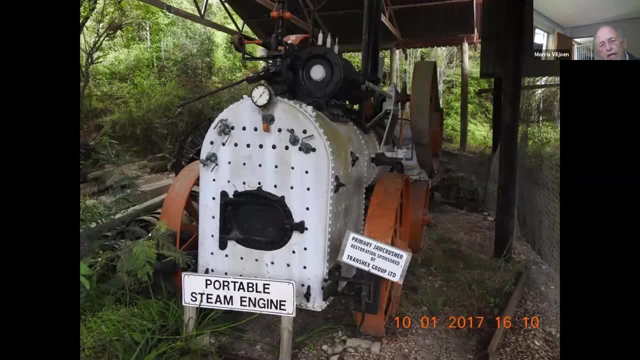 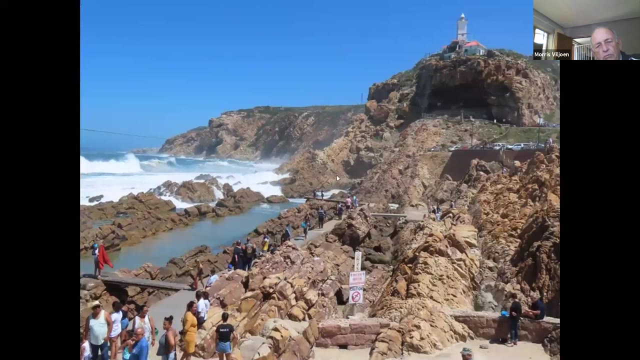 There's the old Millwood mine. There's some classical exposures to the quartz veining that was mined there- big story about that as well- and controlled by the underlying geology. and more recently this is the called capes and blaze and good exposures here of the court sites. 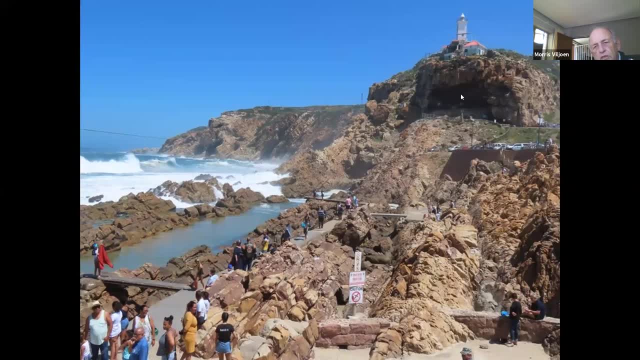 and then with the overlying younger sediments and at the base is this big cave, this muscle bay cave, and with these younger sediments also occupying the top of the wave cut platform here. and but the interesting thing here is that just recently, but probably less than a year ago, 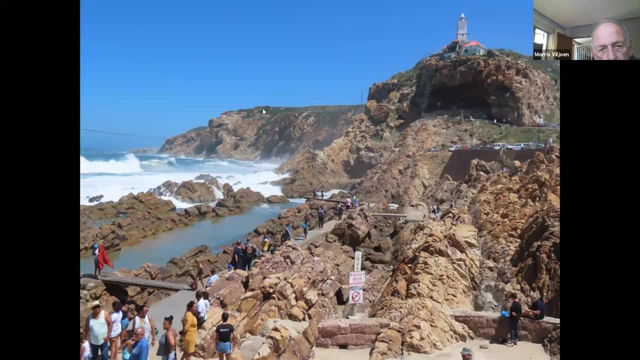 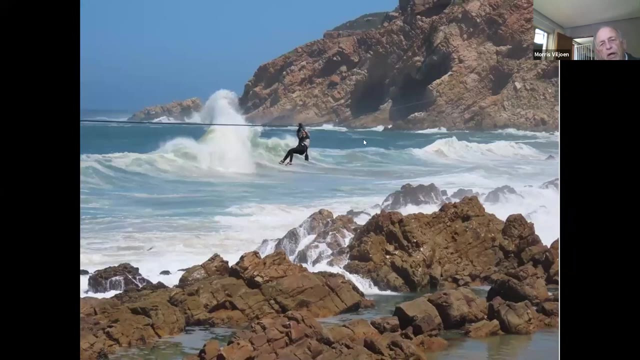 a major zip line was built and it starts up here and it comes down through here. you can see it over here and there's someone on the zip line and it's, in fact, the longest zip line over the ocean anywhere- one, one and one and a half kilometers. so, uh, once you get to the bottom of the ocean, 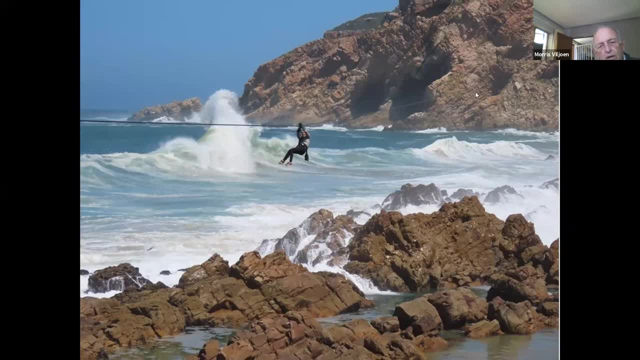 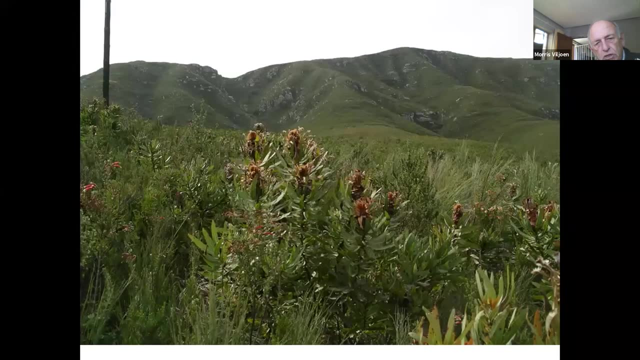 it's a long strip along that bottom line and then up and down, and at the top of that there's a huge bar of the ocean- and this is the base you're talking about, which is the, the arch of the back of the probe, and up here we have some of these, these small. 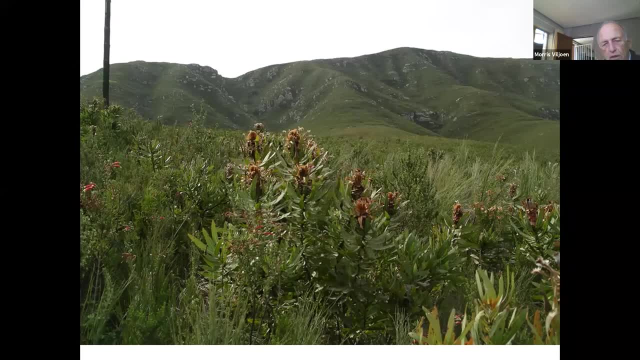 slabs that come down the canteras up to the bottom, and then this is the mainland and that sort of goes down here in the middle of the ocean to the southern part, and along that over here we kind of have an area where the top line is, um, you know, you see, that sort of thing of. 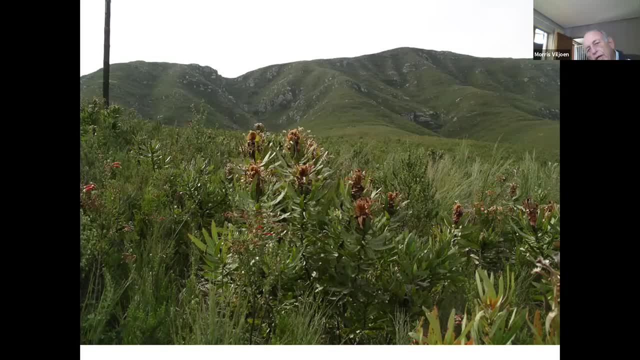 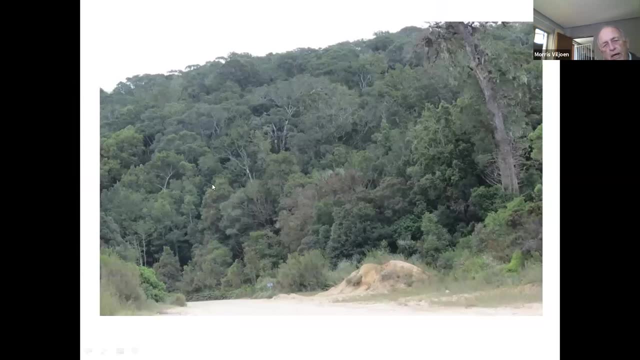 and North Otunuku Fanebores based on geology and landscape. We also, of course, have the Knysna forests, and they are there because in that locality, Knysna to Tsitsikama in particular- 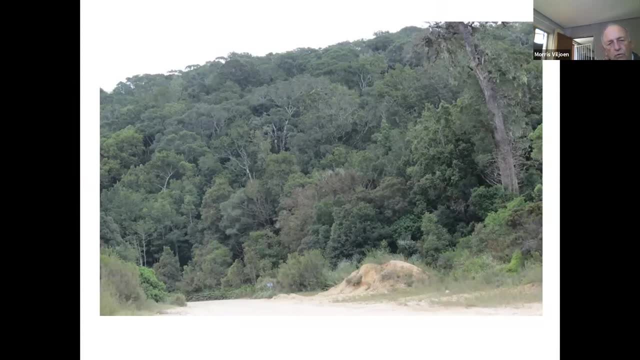 or George to Tsitsikama. you get a lot of rainfall and the coastal mountains are closer to the sea. So you get this classical forest and the big story about the wood industry in the Knysna area, And so that, in essence, tries to bring to one's attention. 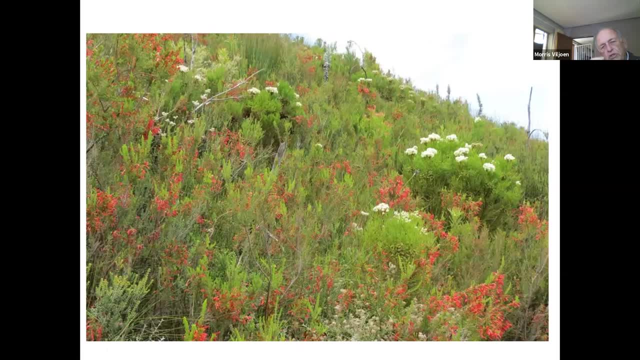 the kinds of outstanding features that occur geologically and how the geology is really determined, just about everything else one sees in the area and tries to give a holistic tour of the garden, not just focusing on one thing but giving the whole holistic tour. 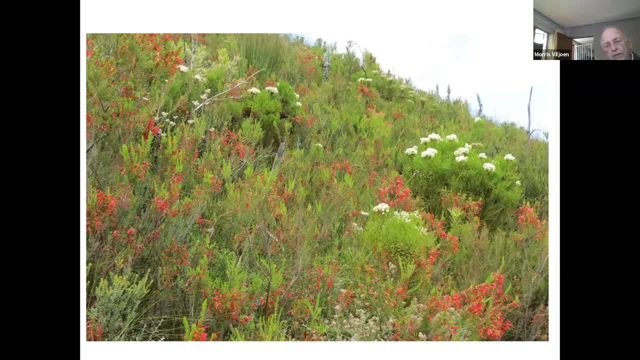 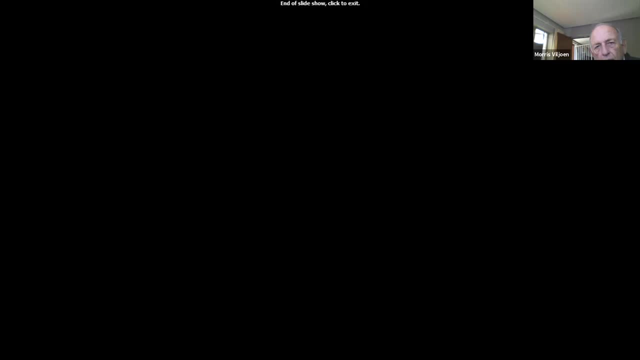 but essentially based on the underlying geology and topography. So yeah, thank you. Thank you, Stop sharing, Stop sharing. Thanks, Mark Helen. you need to share your screen now. How's it coming Interesting, Helen, are you there? 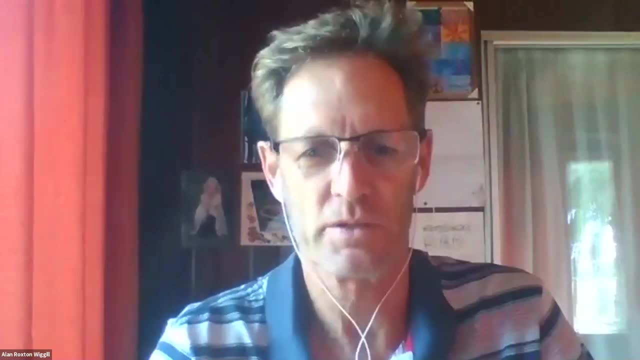 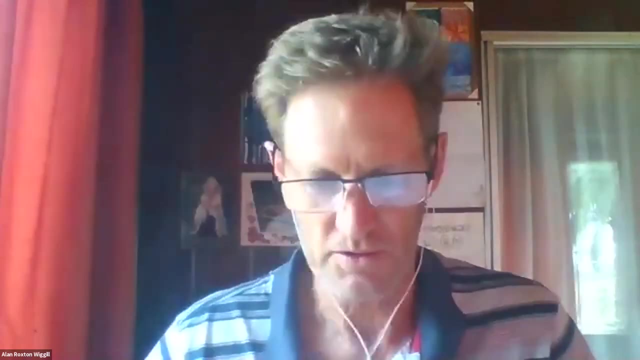 Can you hear me? Can you see me? Can you hear you? Yeah, sorry, I just wasn't responding for some reason. Good afternoon everybody. Thank you so much for the opportunity to chat about a geo heritage community that we are trying to develop. 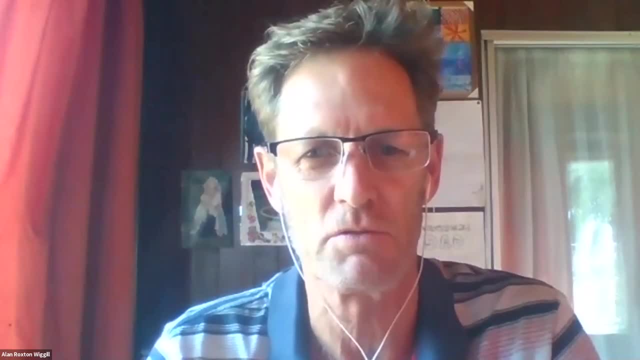 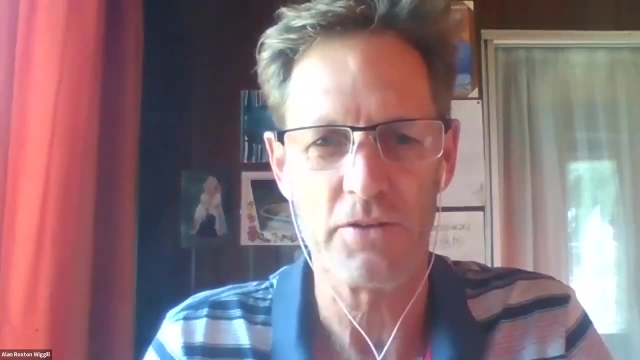 in Southern Africa. Thank you to Morris and to Richard on a number of levels. The fact that they have stood up and driven the efforts to create a geo heritage society over the years- or a geo heritage community, should I say- is a very important thing. 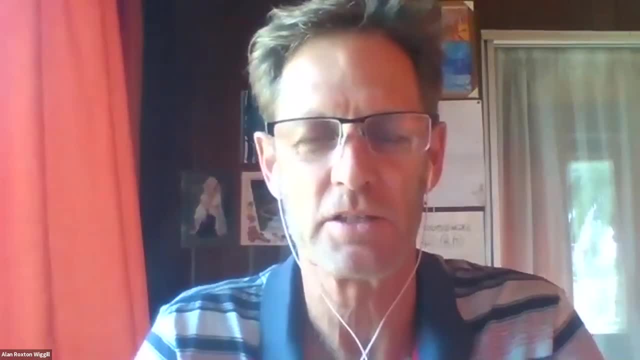 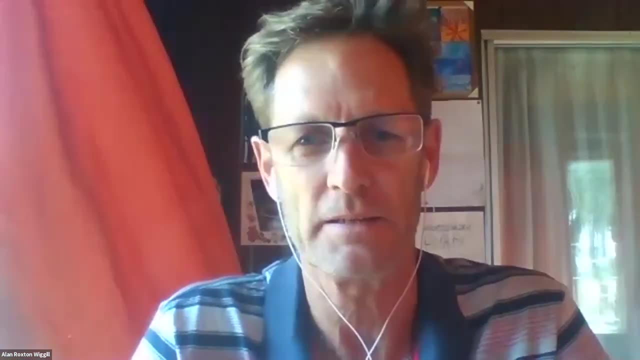 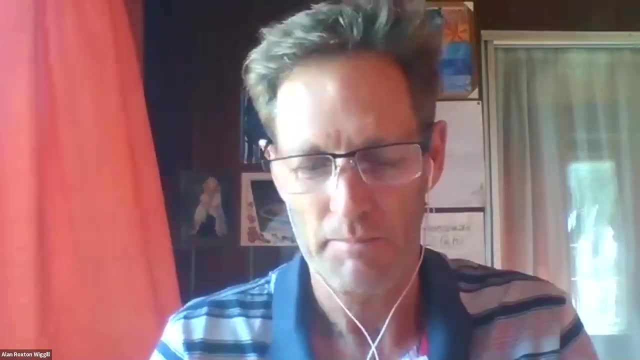 I think, has eventually started to gather some steam, as has the efforts of many others, such as Chris Hatton and Craig Smith and many, many other people that I've been chatting to. There's a huge enthusiasm to try and develop this And basically I've come from the tourism background. 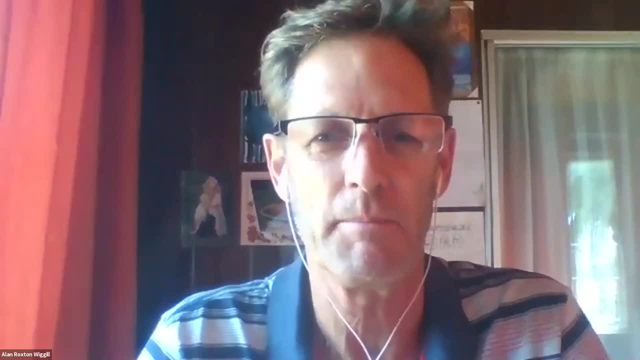 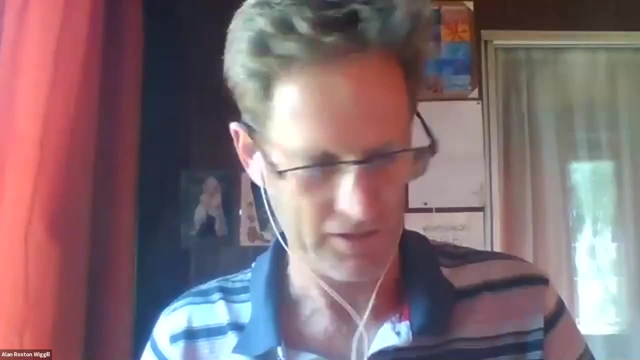 and from a geological background. So I have a very strong interest in trying to make this work as well, because we have a real asset on our hands and it seems not many people are interested in doing this. It seems not many people know of it. 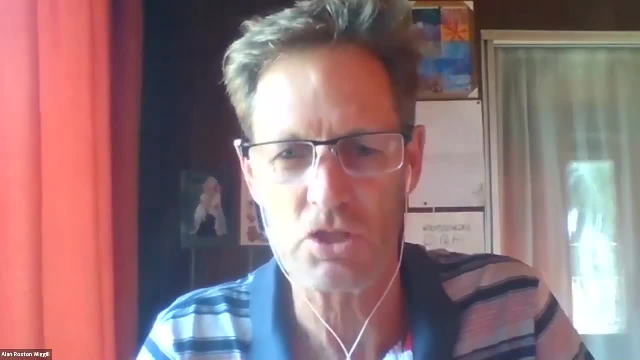 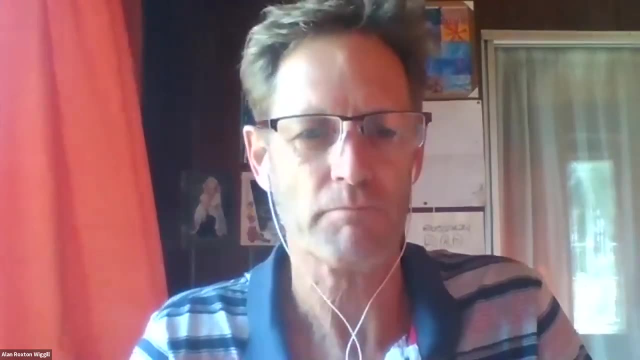 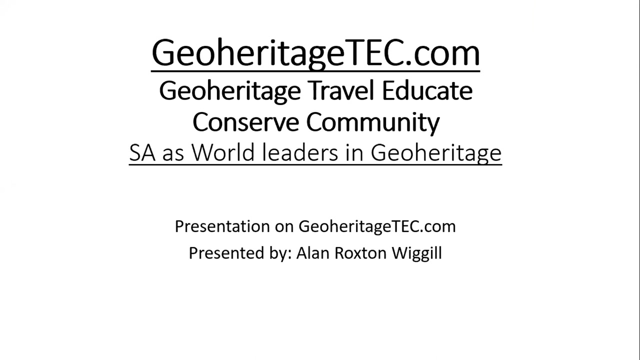 I'm just going to bring up my screen share so I can start my presentation. Okay, here we go, You're there. So basically, we've come up with a concept of trying to create a community of geoheritagists. I'm not sure how that sounds in reality, but anyway. 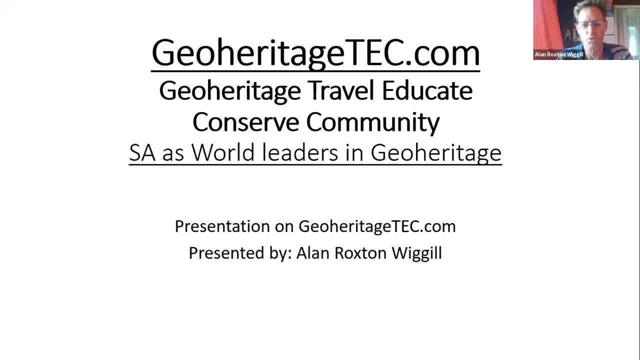 It's people who have an interest in geo heritage, and it covers more than just the rocks. It covers basically the evolution of life and humans around the rocks and the evolution of rocks themselves. So it's a development of the Earth as a holistic view. 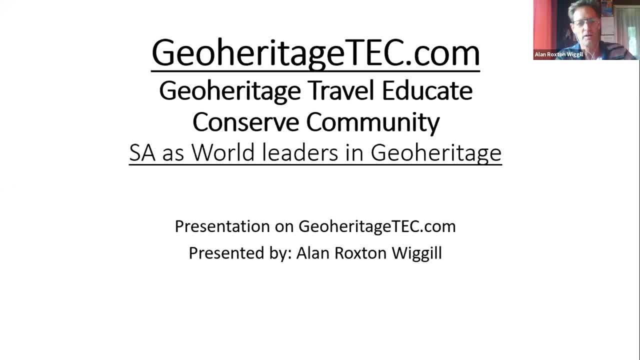 of geo heritage rather than just viewing trees, sands, plants, animals, et cetera. So we're trying to actually give relevance to those trees, plants, animals and life on Earth, which is all based in rocks, and the development of the Earth, which goes back. 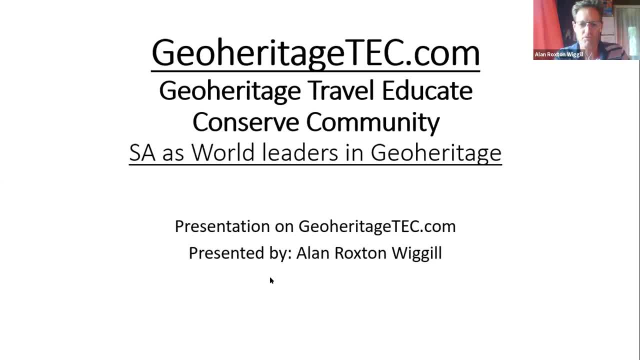 A long way. My name is Alan Rockstone-Wiggle. As I say, I come from a geological and tourism background, So I'm trying to draw or lead the drawing together of our community and take you through a few slides of what we have achieved so far. 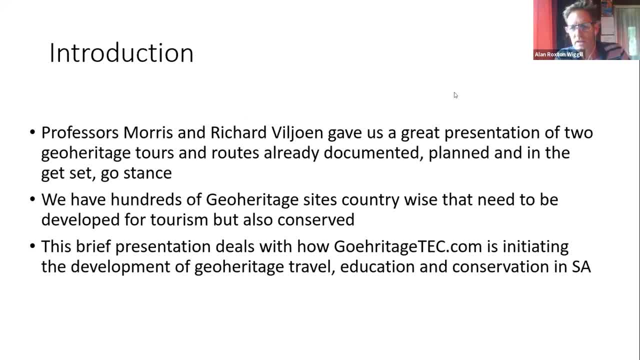 Okay. so I'm sorry, I must just reduce this a fraction because I can't see it Okay. Thank you. So the two profs, for your presentations on the geo heritage, tours and routes already documented and planned and set to go. I think both of the presentations highlight. 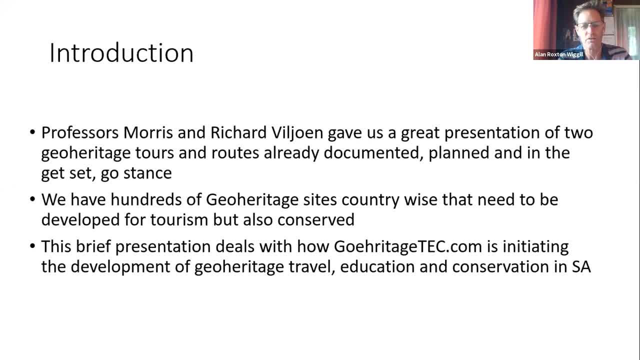 what incredible opportunity there is to create geo routes, geo sites and geo heritage destinations. Very nice presentations, Very interesting. But also something I'll bring to everyone's attention towards the end, when we talk about marketing, is that it does cover geology thoroughly. 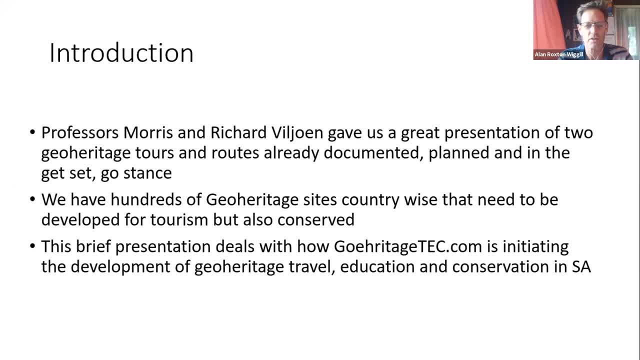 it has a hint and stories of interactions as a result of geology, But maybe something we as a community will need to have a look at more seriously and more carefully is how we explain this whole business to people in terms of a story. In other words, we need to relate our geology. 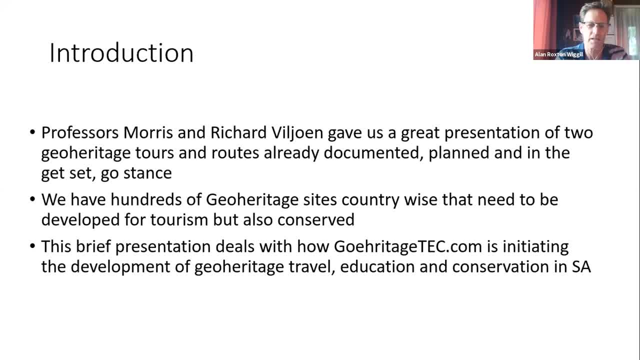 geo heritage to human beings, because it's human beings who are either going to take these tours and love them, and then fall in love with what they are and conserve them, or we won't succeed in the longer run. So we have hundreds of geo heritage sites countrywide. 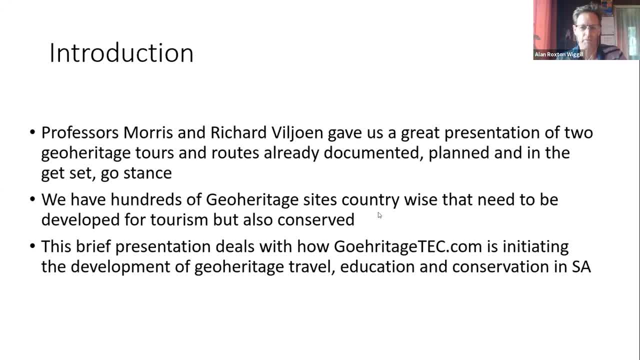 and they need to be developed for tourism, but also conserved. Coming back to my point, if you can't get people to understand them, then don't conserve them. Okay, so we're just going to go into a little bit of detail. 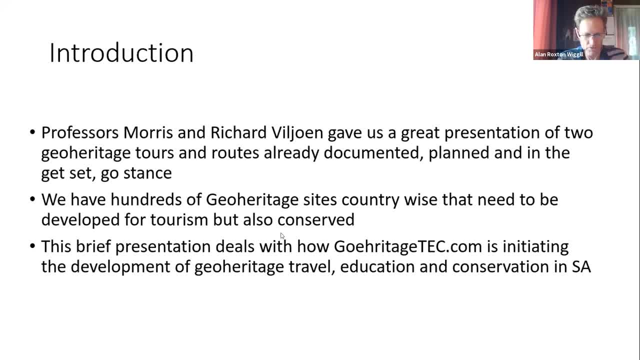 about how we initiated this. Going back into I think it was November last year, I got hold of Craig Smith and Craig directed me to the two Fuyun brothers And we started a little community trying to look at how to develop this process of a geo heritage. 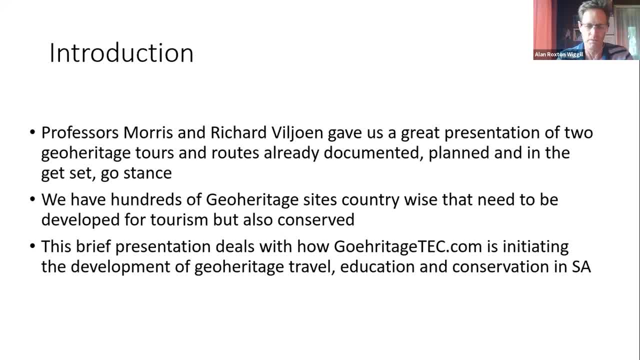 community. As of yet, we have established the actual community itself. We have three founding members, being myself, Richard and Morris, And we are trying to put forward some form of a structure within which we can work as we go along. So next slide. 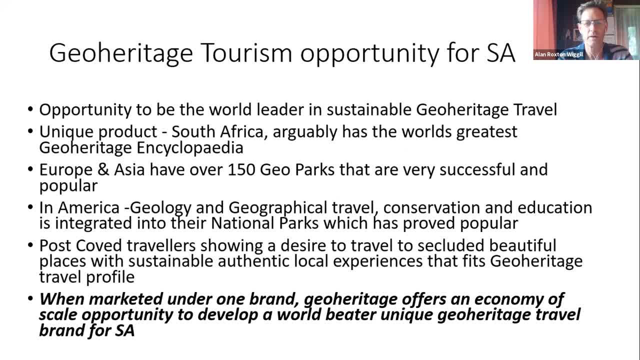 Geo heritage tourism, So the opportunity to be the world leaders in sustainable geo heritage travel. That is really what we're trying to achieve. Unique product: South Africa arguably has the world's greatest geo heritage encyclopedia, If you go back and look at our rocks from start to finish. 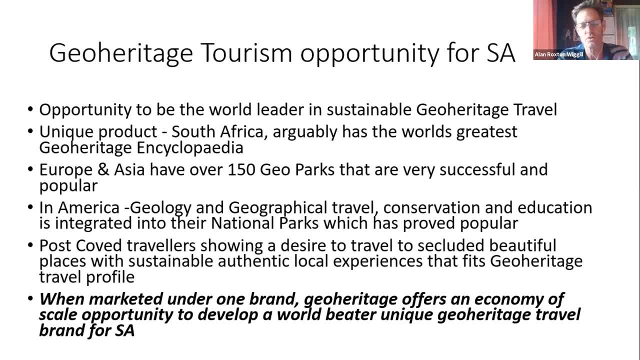 and if you have a look at our life on earth and the records of humans and the development of animals on earth, South Africa has probably got an uncontested number one spot and we need to take advantage of that. Looking a little further outside of South Africa, in Europe and Asia, over the last 30 odd, 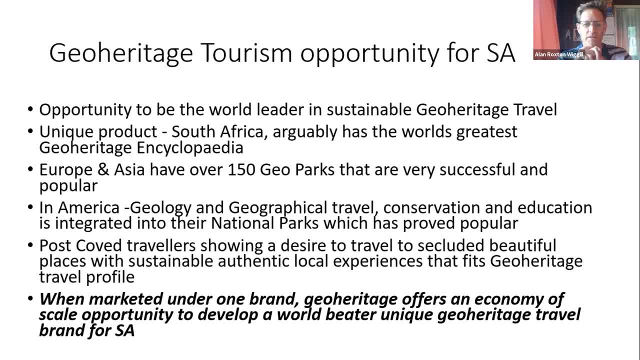 years the UNESCO Geoparks have been developed and there's over 150 in Asia and Europe alone and they are taking hold elsewhere. There's already a couple in Africa. Australia is developing them and there's a number of different places developing them and they've proved to be very successful, which is encouraging. 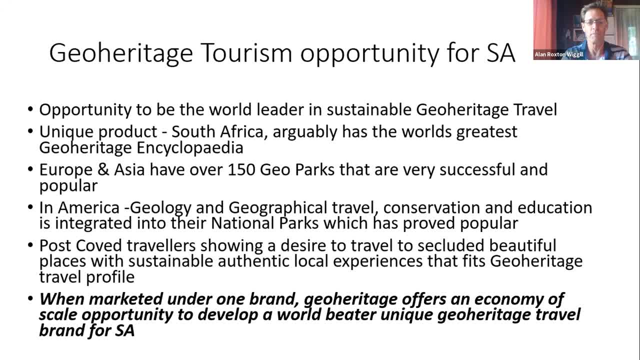 from our point of view, because that means people do like them. In America, geology and geographical travel, conservation and education is integrated into their national parks and it's also proved very popular. They haven't gone the Geoparks route and there's various reasons, many of which are similar to 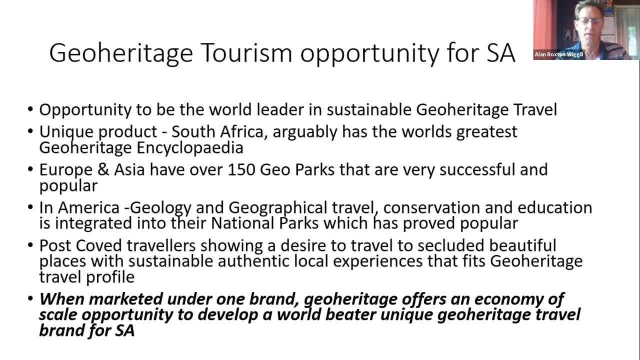 where we in South Africa stand, where the national parks are very strong and very big. so we have slightly different set of circumstances to Europe and Asia. If you ever look at the post COVID travelers, there's a strong desire to go to beautiful places that are out of the way and a very, very strong drive internationally for 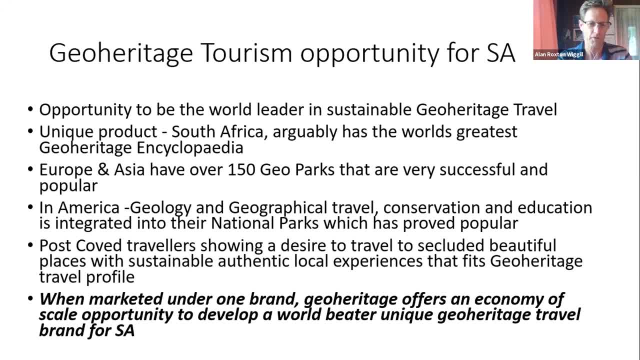 authentic local experiences and it fits the GeoHeritage profile very well. Many people- and I've just finished reading an article in BizCon- travel where the whole thing is about how people are changing their desires and their wants and a lot of what we see in GeoHeritage. 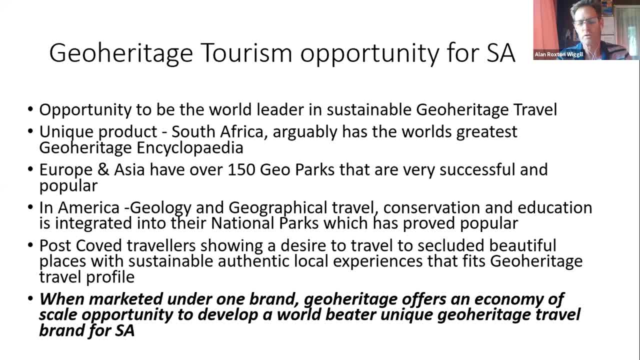 travel, which is going to far-flung places, enjoying local communities, local heritage and history, as well as integrating that into a geological story and why those places exist and why people exist there. It's something that's becoming more and more popular post-covert. 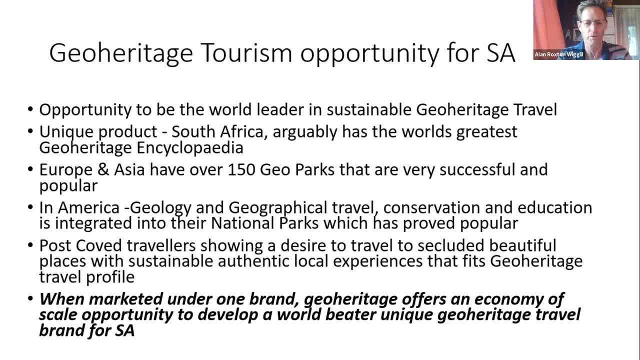 and although we currently only have local travel and we're about to open up to African travel, the market for the international people coming in will return, but there is already a fairly large-sized market waiting and available for us just from local travel. 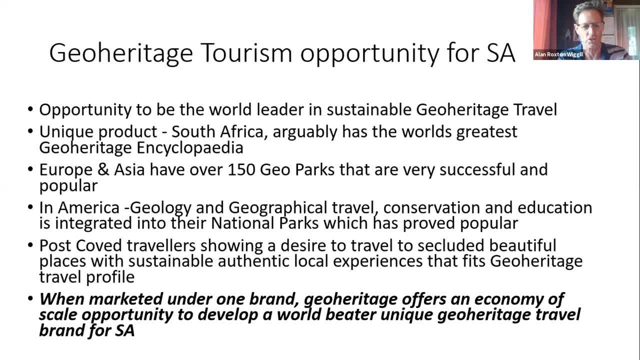 So we will probably focus on that initially And what we see is really important over here. We don't have a group of us GeoHeritage scientists and community working together under a single brand of GeoHeritage. that'll offer us an economy of scale to develop a world-beater, unique GeoHeritage. 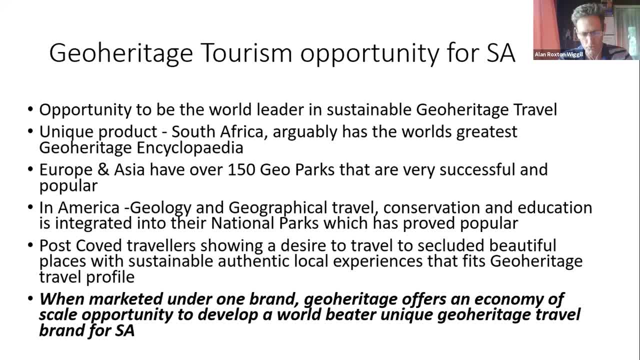 travel brand for South Africa. So we really we believe it's important to get a unified community. we work together to create what we want to do and we're, at the same time, we need to give what we're doing a brand or something to actually work with. 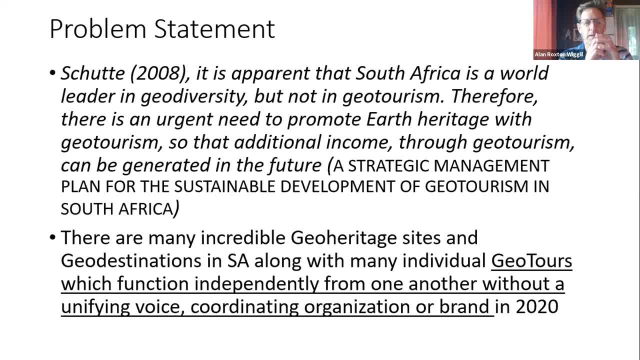 Just quickly a problem statement: 2008 scooter from Nairobi. Please let me know if I forgot the problem statement. Northwest University during a strategic. well, in his strategic management plan for sustainable development of geotourism in South Africa, He said it is apparent that South Africa 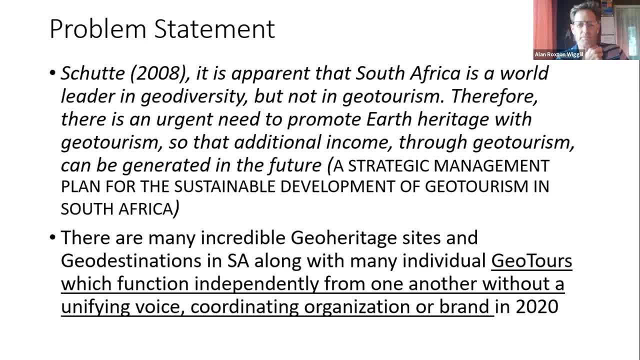 is a world leader in geodiversity, but not in geotourism. Therefore, there's an urgent need to promote earth heritage with geotourism so that additional income through geotourism can be generated in the future. This was a it's a document I've gone through many times and I've 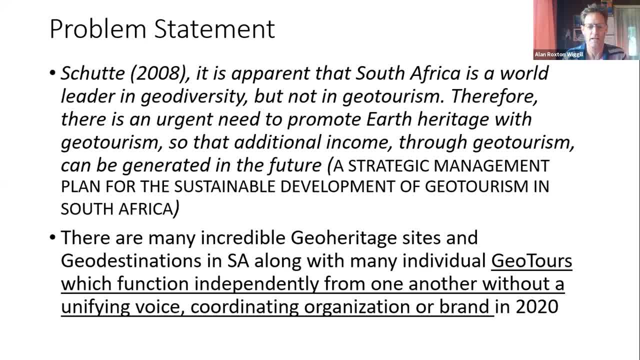 used much of it to help me get a structure and an idea of how we need to move forward in terms of our geotechcom, which we've named. for the moment It's not set in stone, So, based on that sort of development strategy that the UNESCO gave, we have come up with some ideas on how we might move. 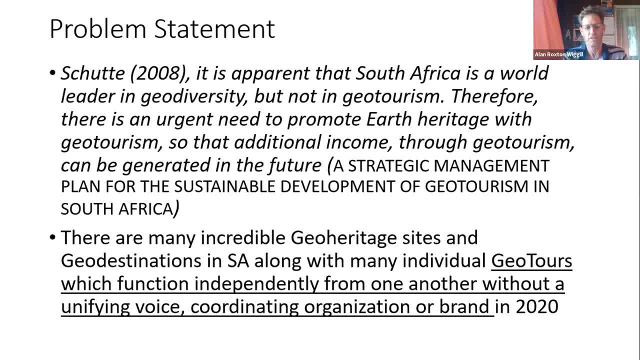 forward as a group. There are many incredible geoheritage sites and geodestinations in South Africa, along with many individual geotours which function independently from one another Without unifying voice, coordinating organization or brand in 2012.. 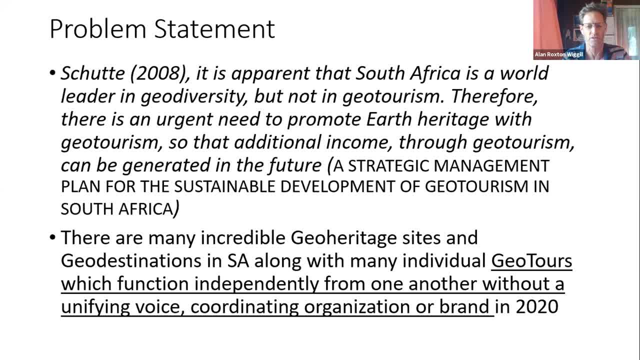 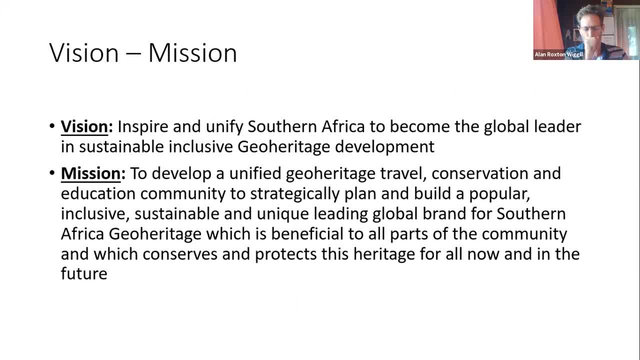 So that is something we obviously would like to change. We'd like to create that voice where we work together. I've chatted to a number of people, including some of the ones we've mentioned already and various other people in geology and geoheritage, So we've come up with a 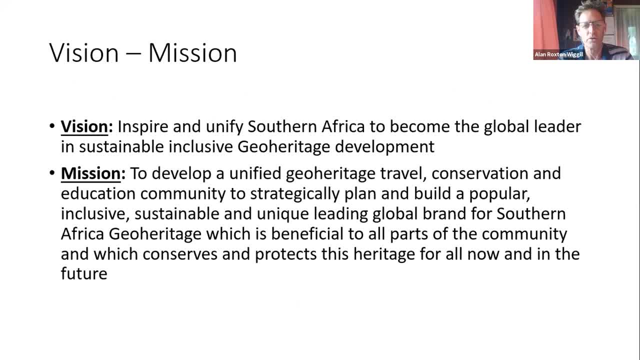 and it's again. it's an initial thing, but we've come up with a vision for our community: Inspire and unify Southern Africa to become the global leader in sustainable, inclusive geoheritage development. It's a broad statement and it may need. 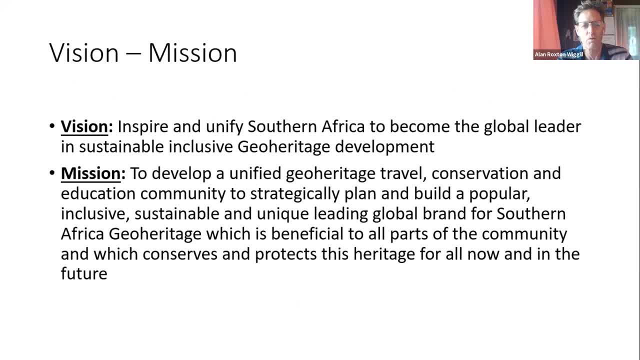 some refining, but it's a starting point. We have taken quite a few different ideas from different people and that's what we've come up with for the moment. The mission to develop a unified geoheritage, travel, conservation and education community, to strategically plan and build a popular 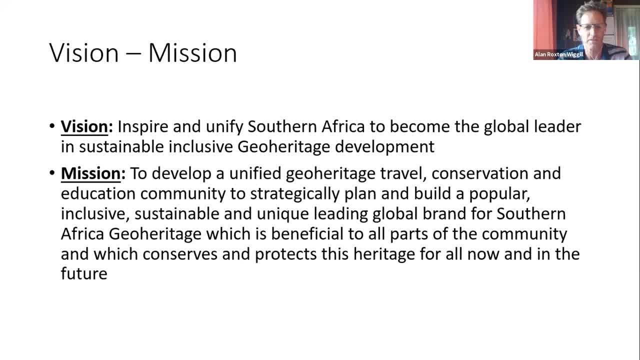 inclusive, sustainable and sustainable geoheritage development. The mission to develop a unified geoheritage travel, conservation and education community to strategically plan and build a popular, inclusive, sustainable and sustainable and unique leading global brand for Southern African geoheritage. 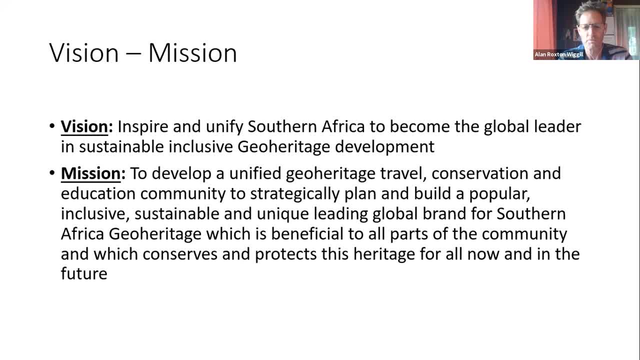 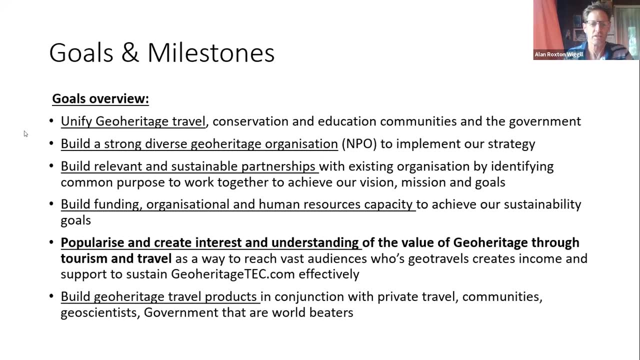 which is beneficial to all parts of the community and which can serve and protect this heritage for all, now and in future. And we've listed a few goals. I'm not going to go into these too much. It's on the, it's on the screen. 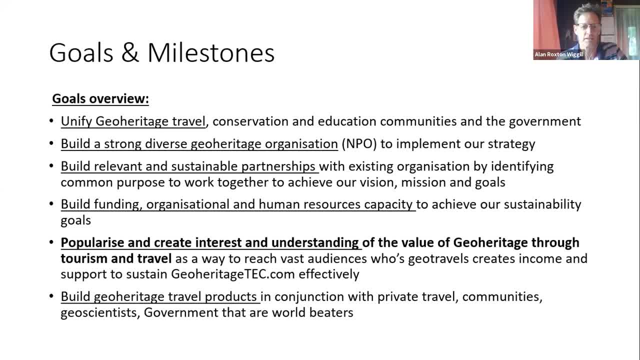 So anybody can access this at any time. Basically, it's again, it's a unify, it's a build. a strong, diverse geoheritage organization build relevant and sustainable partnerships. This is very important because we're effectively, as a community, just coordinating an effort to make geoheritage more popular. 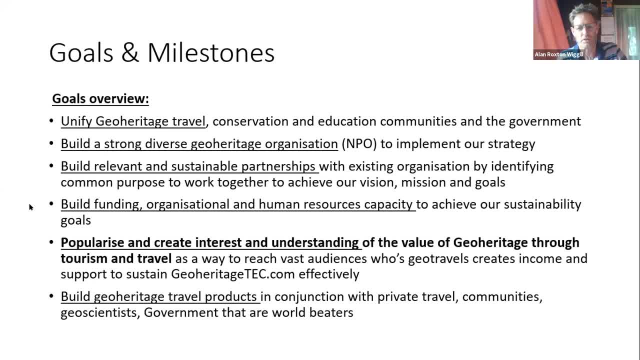 better studied and more accessible. We'd like to build some funding and resources. Again, we need to be unified to do this and we need to have a voice and a brand, Popularize and create interest and understanding of the value of geoheritage through geoheritage tourism and travel. 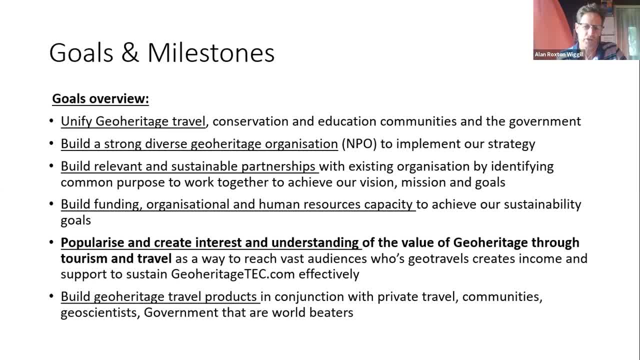 In other words, we need to tell the stories linked back to geology and the geoheritage as to why humans live where they do Build, geoheritage, travel and products. So obviously, without the products and the, we don't really have anything to offer people, So we need to build something that. 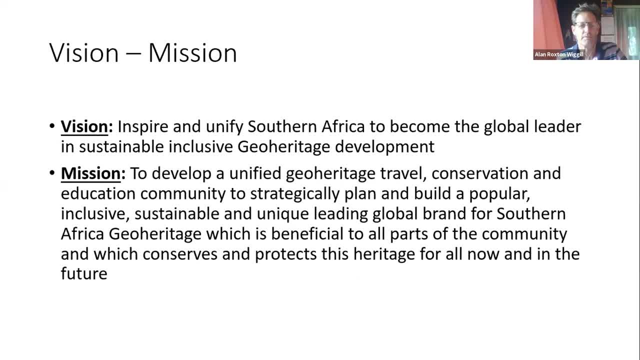 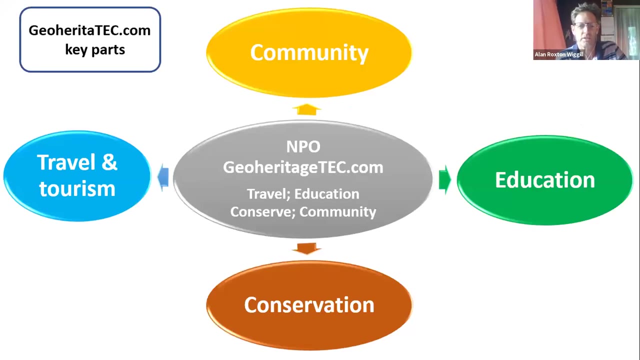 people can actually look at Vision, inspire and unify South Africa to become the global leader in sustainable, inclusive leading. sorry, let me start again. Done that one So effectively. the community will consist, or should I say the geoheritagetechcom will have. 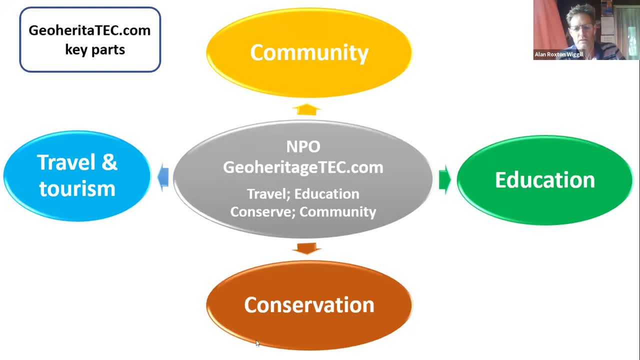 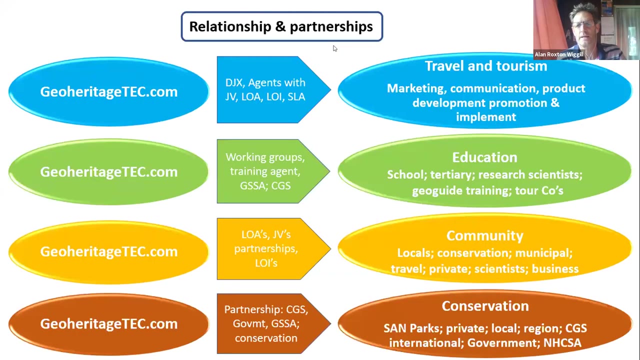 a community. It has education, conservation and then travel and tourism. Most of my discussions from here are going to be about the travel and tourism, because that's where I have specialized in. Just a brief, a brief indication over here is this is: this is the four sections that we deal. 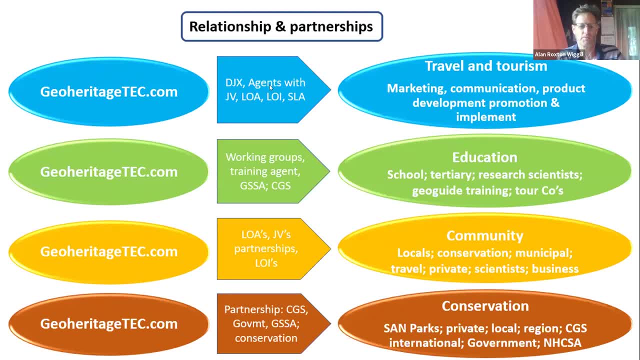 with. This is how we create a partnership And this is obviously geotecheritagecom. So, on the travel and tourism, we will be concentrating on marketing, communication, product development and promotion and then implementing this process. It will be done. 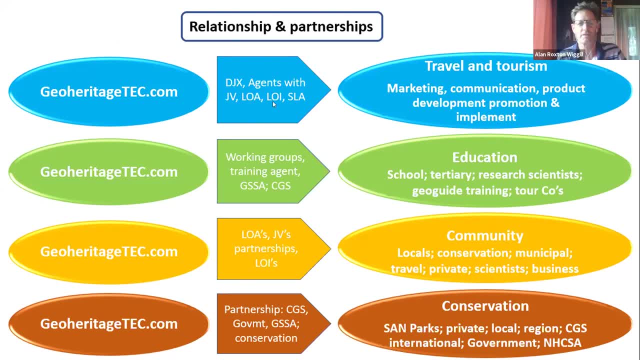 through an agencies or joint ventures. It will be done through an agency or joint ventures. letter of agreements, letter of intent and service level agreements. Education: it would have working groups, training agents, training agents being for when we want to train. 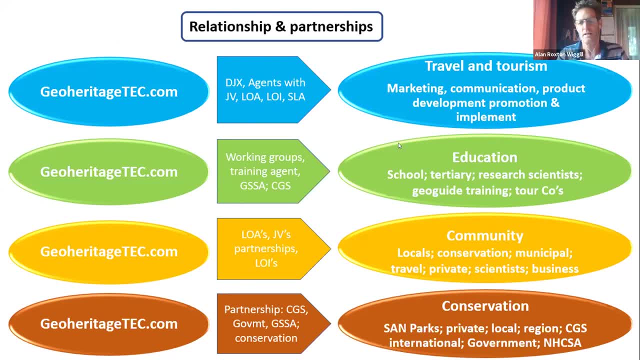 guides, et cetera, on how to present your heritage. There will be a strong input from GSSA and CGS over there Community when we start developing geo heritage destinations as opposed to geo parks. the destinations would cover. 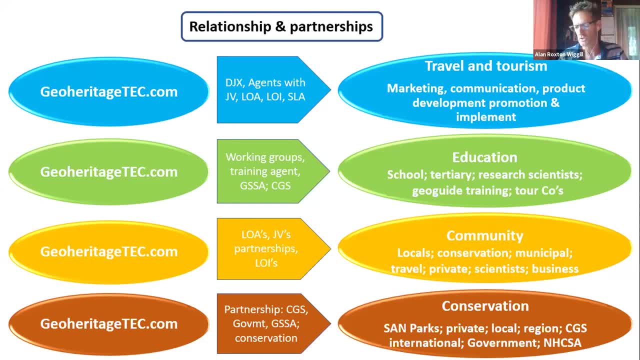 reasonable sized areas of not necessarily very defined geographic boundaries, rough geographic boundaries, but it would include very significant geo, geological and geo heritage components. We have the conservation and again that would have a partnership with various people, including the CGS, GSSA, and obviously it would include sand parks, because they are. 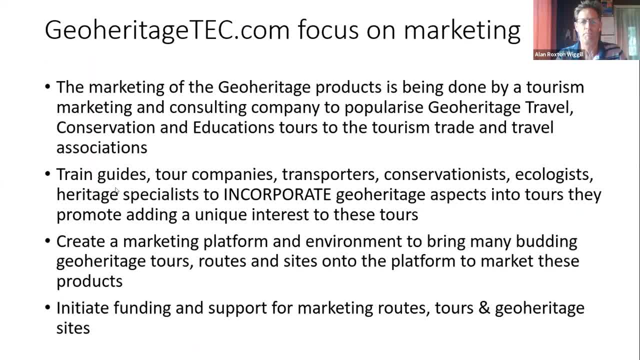 unimportant in that area. I'm going to move a little further. The marketing of the geo products is being done by a tourism marketing consulting company to popularize geo heritage travel, conservation and education tours to the tourism trade and travel associations. That is what we're trying to actually share right now. 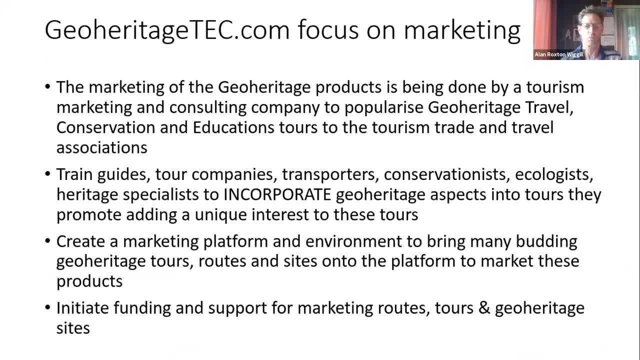 In that direction. we've actually put an application into the Western Cape for grant funding from them to develop various geo routes and geo tours over there. We would look to train guides, tour companies, transporters, conservationists, ecologists, heritage specialists to incorporate geo heritage aspects in tours they promote. In other words, we're going. 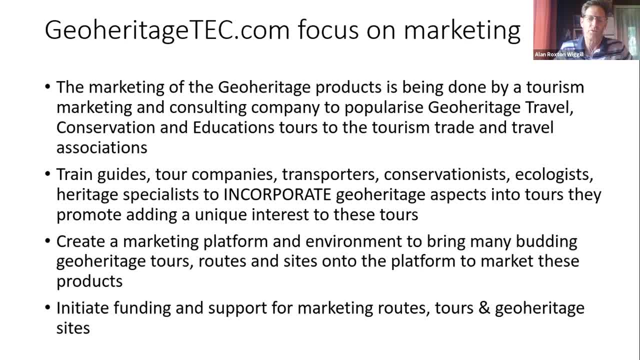 to go to the tourism trade to make this popular using their broad reach to, should I say, other potential clients that we have by introducing geo heritage routes, tours and site visits where either they have a specialized guide or we, through our association, could provide specialized guides. 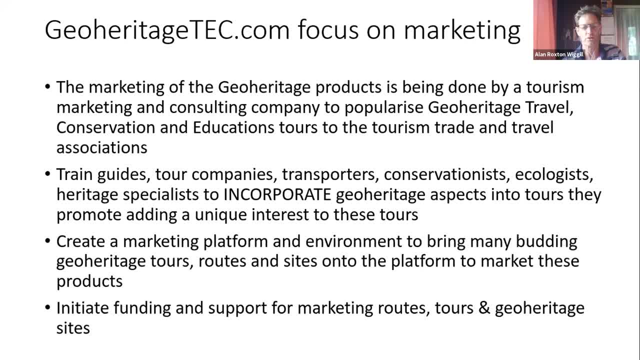 We'd want to create a marketing platform, which would include a website and then many other things that go around it. We would obviously need some funding and support for marketing routes and geo heritage, but a lot of this is private enterprise driven, so individual peoples and companies. 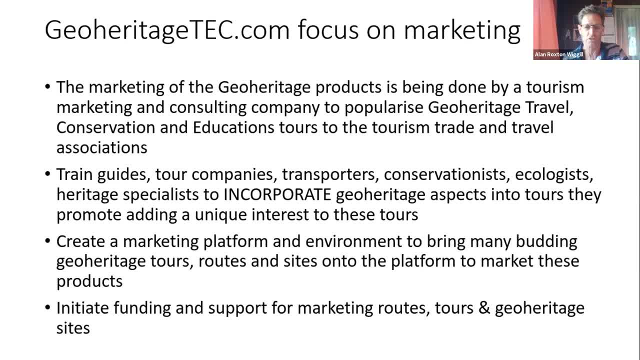 will start seeing the value of this. Many of the geologists and archaeologists and paleontologists have already started developing routes and developing areas that we can actually work with. Essentially, we will coordinate and help with the marketing of this. The Geo Journeys is the name that has been chosen. 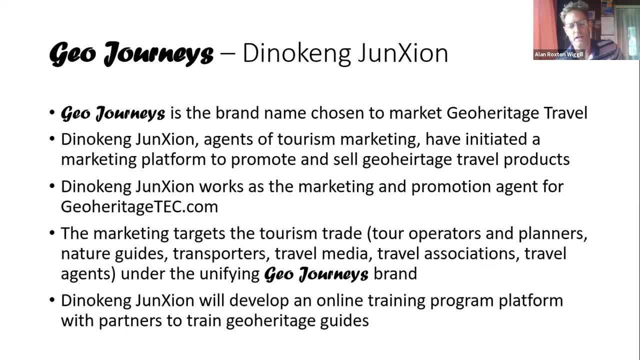 by Denikin Junction, who's been asked for the moment to do the Western Cape presentation, or should I say application. That application is in. we are under consideration. We are waiting for an answer to that application to get grant funding. 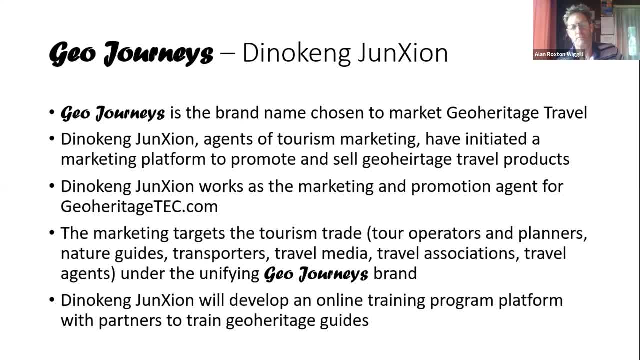 And we've applied for about 670,000 rands. The money would go a lot to virtual tours, to developing our website and then to create links with the different areas of tourism and tourism trade within that area and then to work very closely with Western Cape tourism. 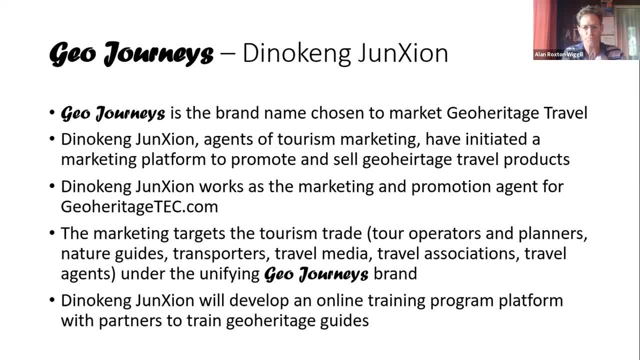 to try and develop geo heritage travel. So basically, Denikin Junction will initially be the agent that the geo heritage community uses. It's all on risk at the moment, so we'll see what comes out of that. The marketing targets, the tourist trade. 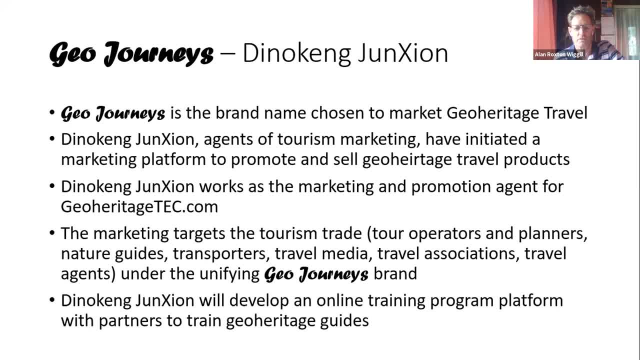 tour operators, planners, nature guides, transporters, media, et cetera, et cetera. So, as I said, we're focusing on the trade of tourism, not on the end user, not on Joe Public at this stage. 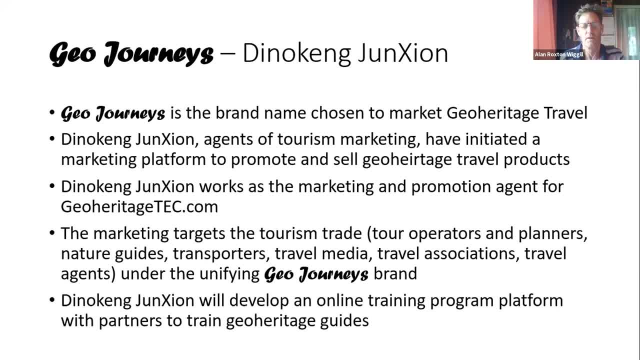 So we would use these guys who are very, very experienced in getting to tourism, and we have spoken to them quite extensively already. They're pretty keen on the idea. They obviously don't fully understand it yet and we would need to do a lot more presentations. 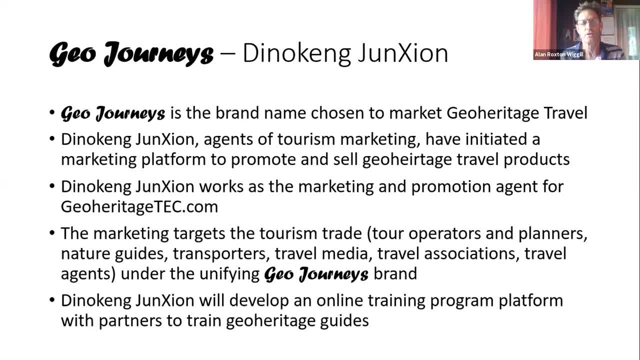 and create a lot more infographics, videos, et cetera, to help them understand Why geo heritage could actually add a lot of value to their tours and could differentiate them from anybody else in the world, Because most travel specialists these days are looking for something which differentiates them. 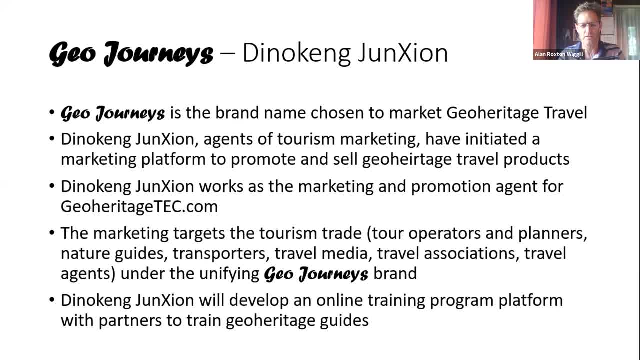 from the rest of the world, as opposed to just from each other within South Africa. So our South African tour operators and the people who bring people to South Africa are looking for something that sets us aside or makes us special and different And really South Africa, with its incredible geo heritage. 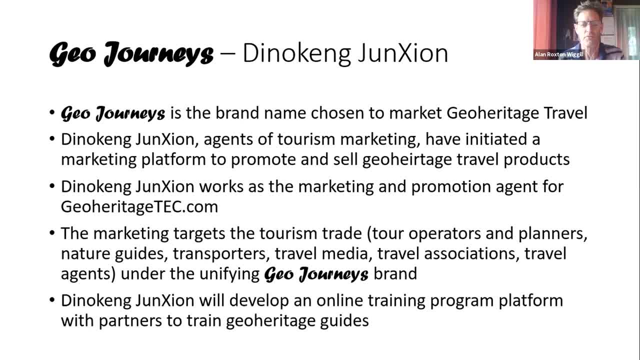 is actually incomparable. if we get it right And if we get everybody, including government and local communities, working with us to create this product, it will give us that uniqueness that so far South Africa hasn't really got itself- a single unique product. 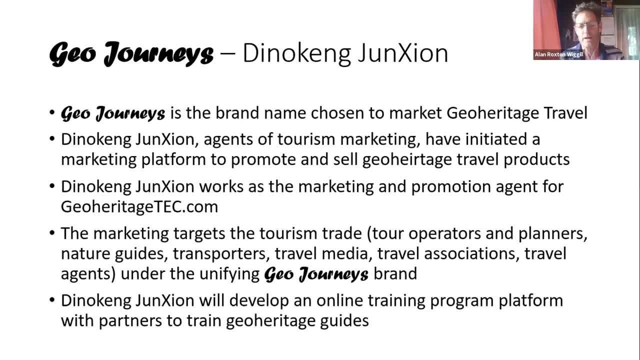 So we do see that this is a very interesting way of going about it. It's easier for us to reach the travel trade and the travel media and the travel associations and the government department. Then it is trying to go straight to a public who really doesn't know anything about this. 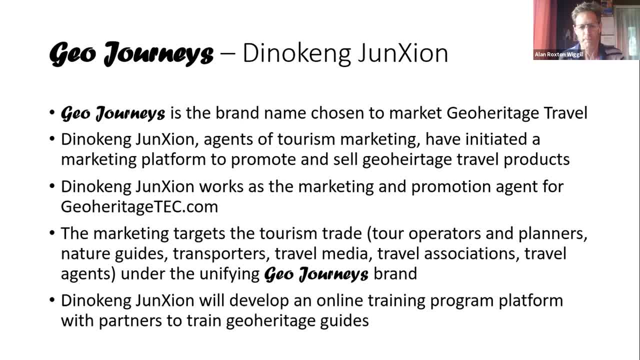 and would battle to understand what we're trying to put across. initially, Dinneking Junction will develop the online training program platforms with partners to train geo heritage guides. This will be very important because by training the geo heritage guides one thing, it creates a revenue stream for the community. 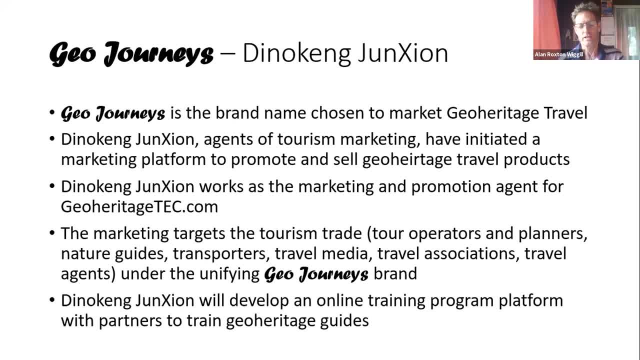 because these will be charged for. And secondly, we can actually get to a much wider range of people training guides who are then available to the tour operators or touring companies, local associations, et cetera, And these guides can often will be just standard nature guides. 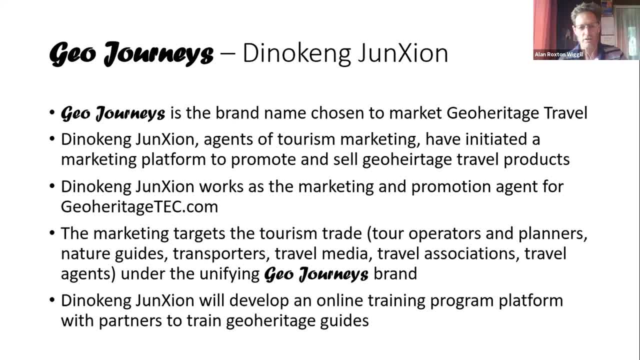 who really know a lot about nature but may not have incorporated geology and geomorphology and landscapes properly into their presentations. So it adds an extra string to their boat and it creates some uniqueness within those tours The people adopted early. Okay, so I just want to round off quickly. 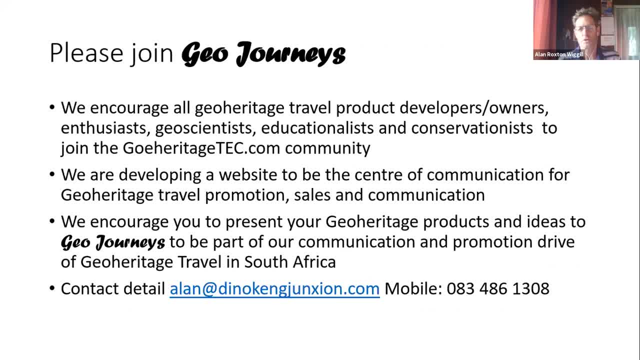 by saying geo journeys. We encourage all the geo heritage travel product developers, owners, enthusiasts, et cetera, anybody who loves this geo heritage field. We encourage you to come and join us. We will put out broadcasts through various areas and channels to explain to you what we are trying to plan. 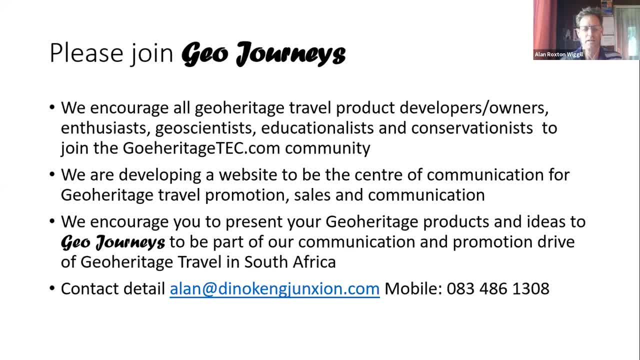 This is not a top down community. It's a bottom up community, driven by innovation, by private sector and joined by the tourism trade associations and government to try and build up something which is unique to South Africa. So I do stress that this is definitely a bottom up. 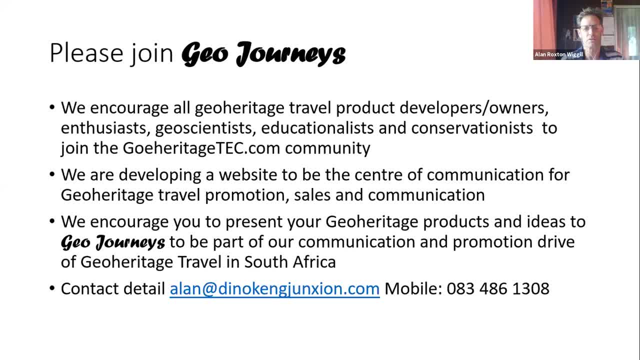 not a top down. We've had to start the way we are now because you've got to get something going and we desperately would like everybody to join us and give us the inputs on how to make this work, How to make this a better program, a better community. 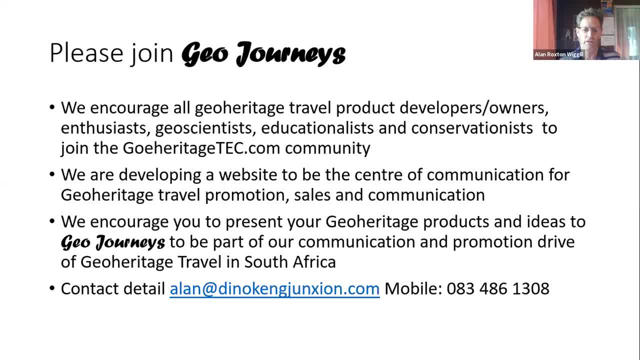 At the moment we're really developing a website, a center for communication for geo heritage, travel promotion, sales and communication. that's underway. If we are fortunate enough to get the Western Cape Grant, that'll happen a lot faster. but we do also have other possible areas. 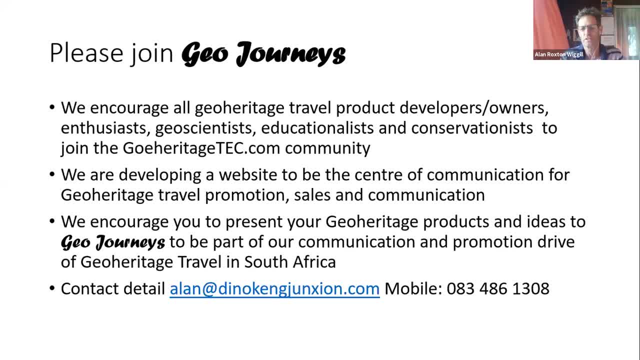 of funding to create this. We encourage you to bring your geo heritage products and ideas to geo journeys to be part of our communication and promotional drive of geo heritage travel in South Africa. I can't stress this enough. We have so many incredible products all around the country. 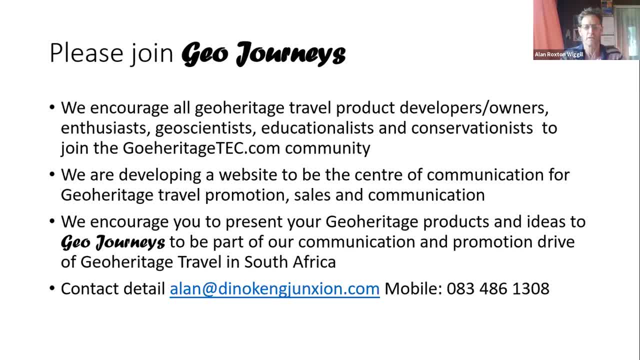 They developed, they're ready to go. They've got great people itching to show people stuff And I've lived through this because I've done tours to Cullinan. I've done tours down to the low field, which are geo heritage tours. 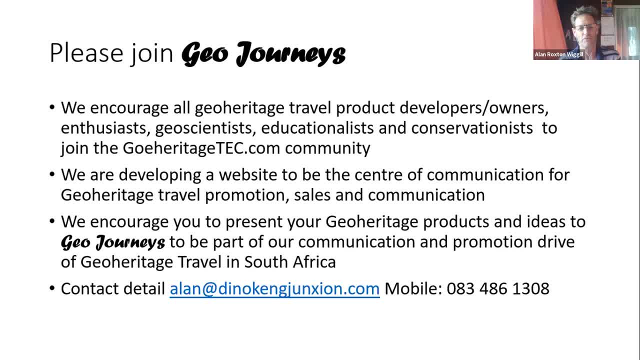 And I have my little pet one, which is the Tuai meteorite crater, as I live right near it And people absolutely love these tours. but to convince people to go there from, you know, from the top of the mountain to the top of the mountain- 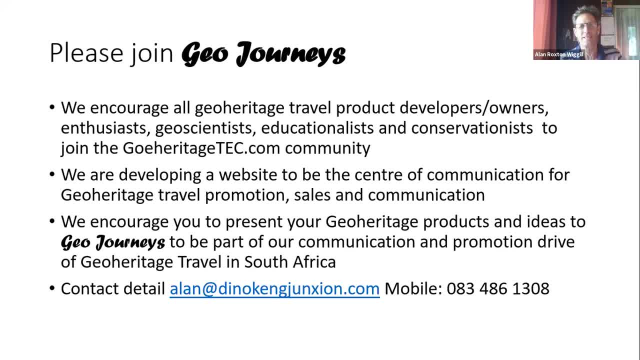 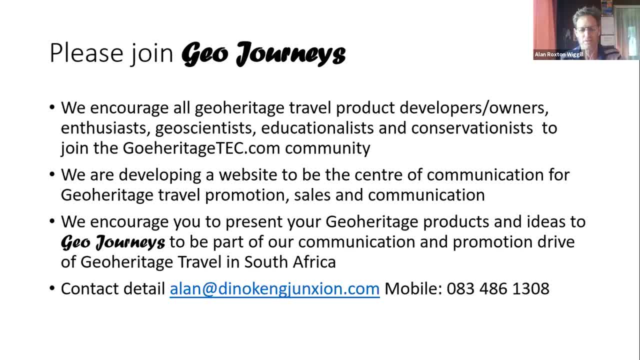 in geo heritage tourism will have got a spot discouraged because it just doesn't happen the way it should happen. We know we've got a good product, We can present it so well. People thoroughly enjoy it when they do come and see it. And yet they don't know about it, so they don't come. 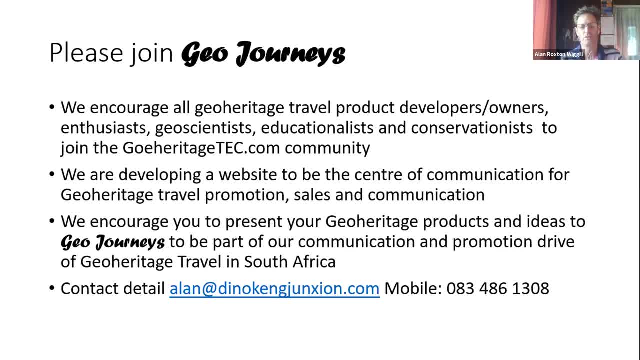 So our idea is to get everybody together, to get our ideas together, to create a globe of geo heritage travel in South Africa. the more of us who do it, the more we promote it, the more we're all going to benefit on it. 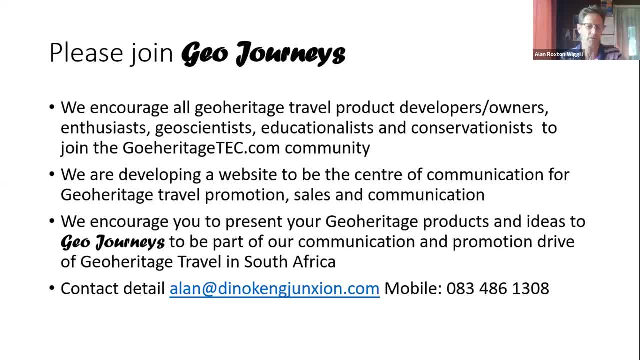 And eventually we should be able to achieve the goal of becoming the leading geo heritage destination in the world. Okay, I think that's probably me, So I'll hand it back to you. Thank you very much, Alan. Thank you, Richard. 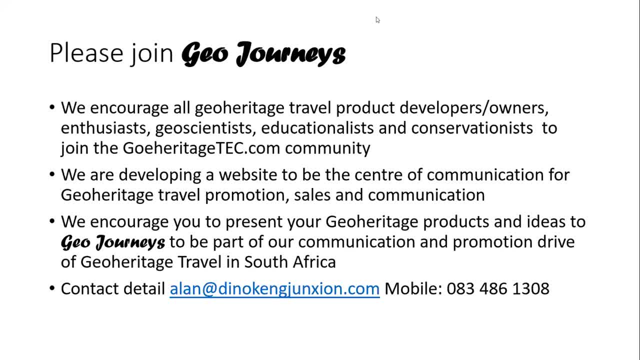 Thank you, Morris. I'll open the floor now to comments and discussion and questions. If anybody either raise your hand or jump right in and unmute yourself and go for it. Do we have any questions or comments? Maybe I'll start with one, Alan. 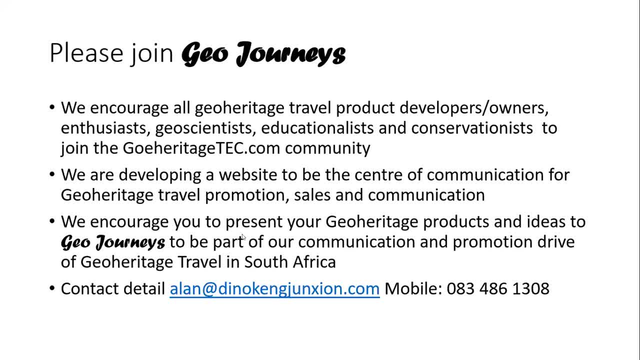 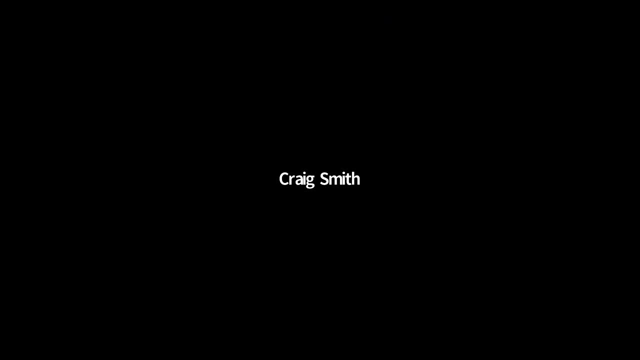 The vision that you're looking at here. it is very commendable and, I suspect, also very expensive If we wanted to roll this out countrywide with, say, 20, 20,000 operators, for example, under some sort of umbrella. I mean, how much money are we looking at? 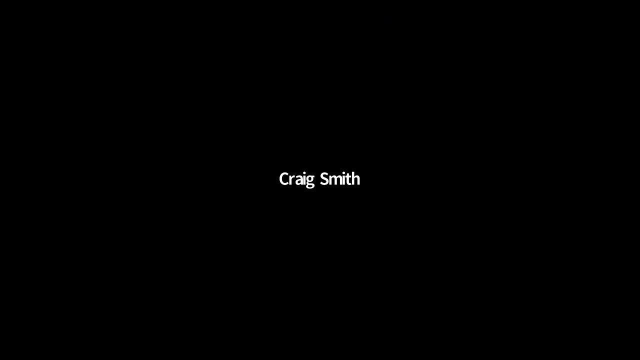 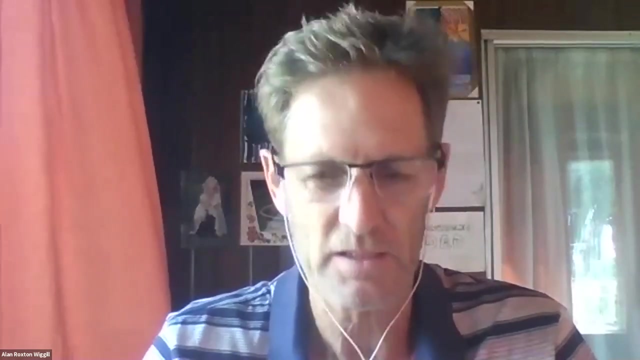 for getting this thing started. Any ideas? I don't believe we're anywhere near there. We're going to have to start small And I think, going back to the discussions that even you were involved with right from the start, I don't think the mindset has changed. We have to start somewhere. We have to start small, So it may just be one Western Cape tour. It may be a three to four turn. It may be a garden route tour. We start with those, Depending on where we can find some funding to initiate it. 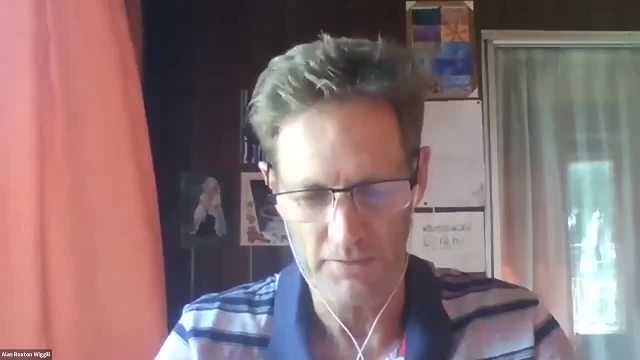 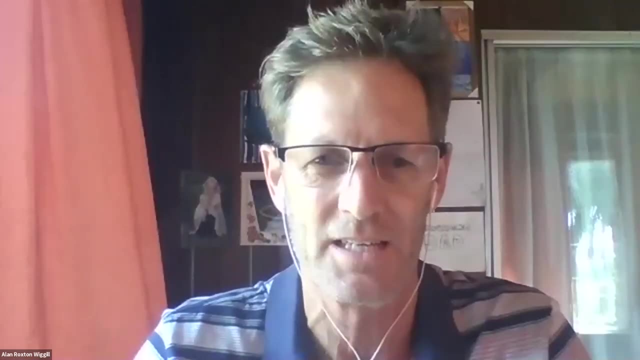 There are a number of people who are interested in it and but have not really got involved. A because they haven't been properly briefed on what is going on And we do not have a proper communication document yet, The result of us not having formed the community yet. 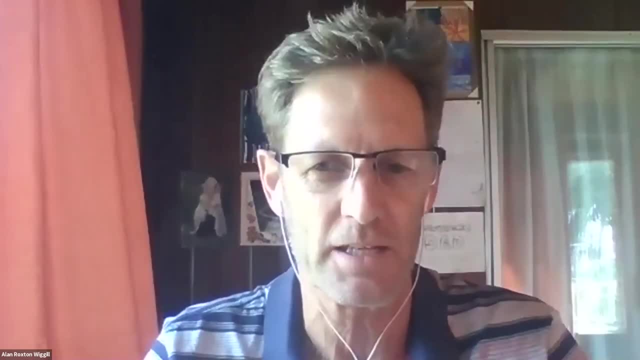 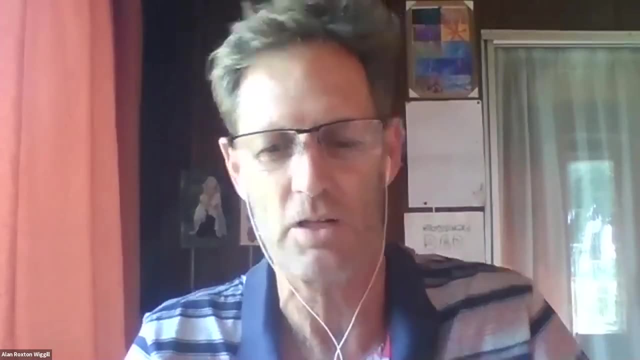 not official body, official name that actually represents the community and the community. So we have achieved that now. So this is a step-by-step stage. I couldn't put a amount of money on it because a lot of the money, as we put it. 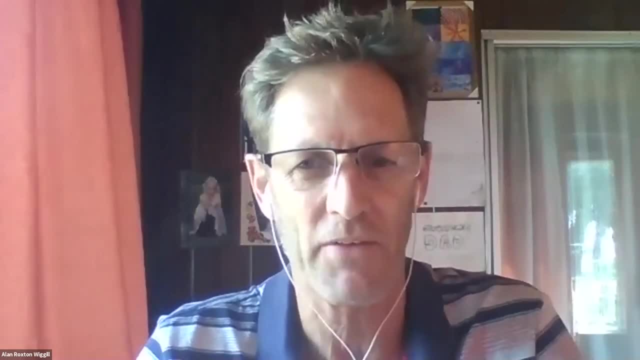 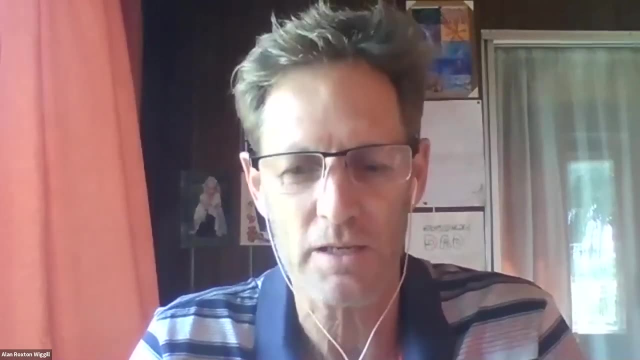 is more about sweat equity, So it's actually getting people together to put products onto our website where we can market ourselves and where we can start promoting ourselves. That is first choice. You've got to get that website going. We need to find enough money to initiate that properly. 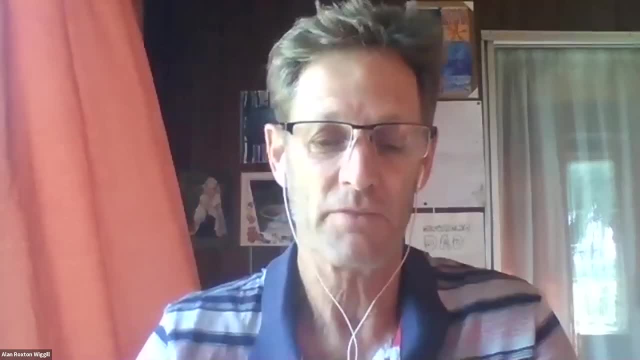 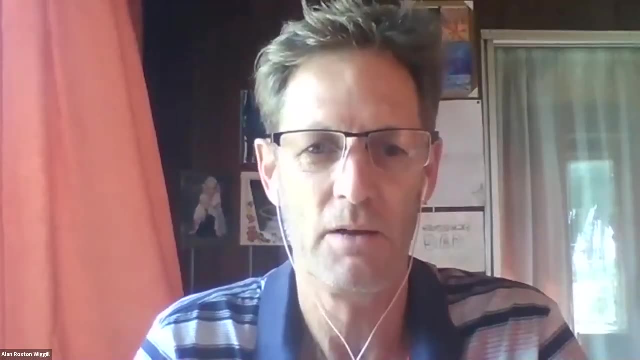 to be able to have it as a booking tour platform. Much of that work I have done myself, because I already have Denneking Junction as it is and I'm busy building exactly that website for myself. But I will be hosting whichever geo heritage products we can get. 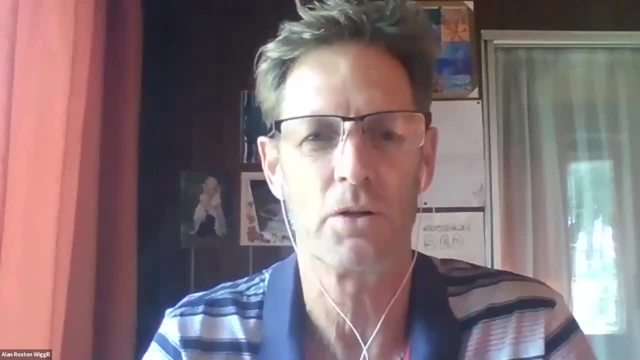 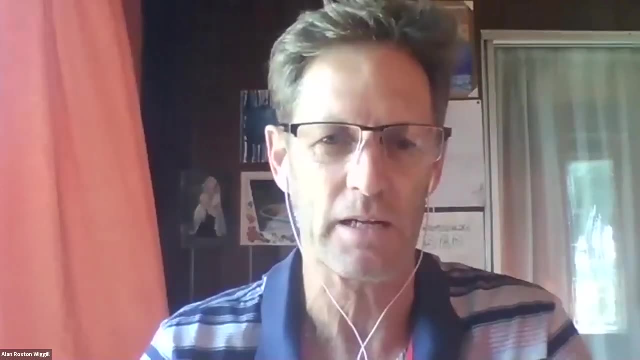 I will host them and sell them on my own company's expenses, But that's just my love of what we're doing- geo heritage and travel- So I'll be doing that anyway, And there are revenue streams from that And that is really where your long-term 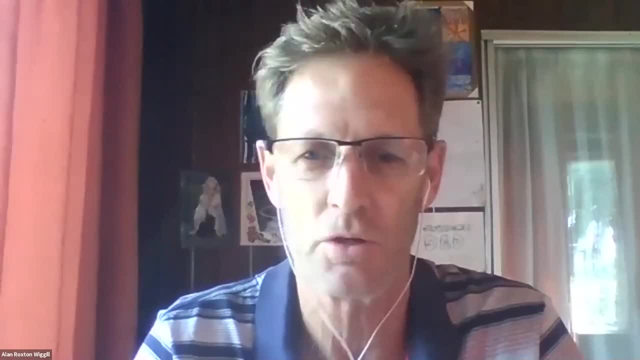 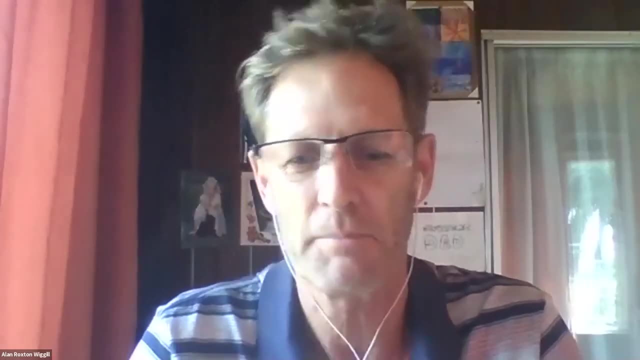 revenue streams come from. It's from your online bookings And from your tour bookings. you take a commission. Part of it goes to our community to help run the community organization And part of it goes to whoever it is who has developed the tour, runs the tour. 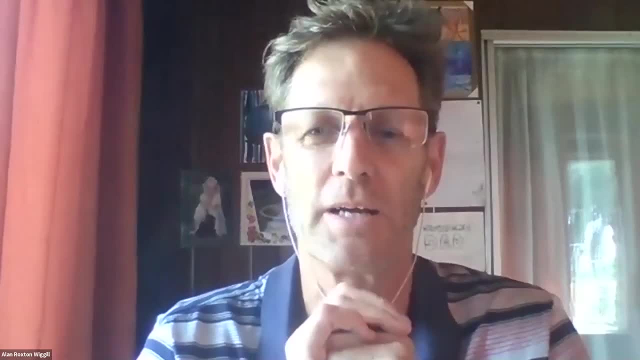 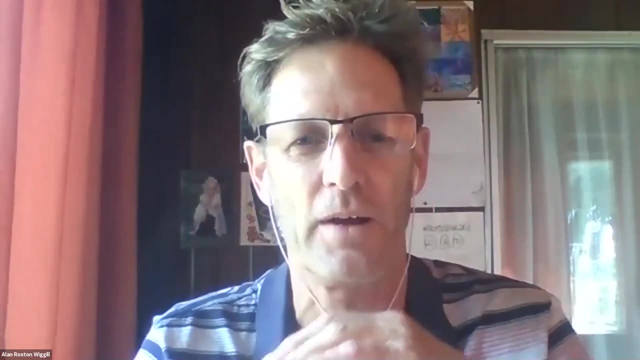 operates it, sells it along with us. So on a long-term basis. I mean, how long is a piece of string? We would need a million rands right now to be able to launch four or five destinations, with two or three routes in each destination. 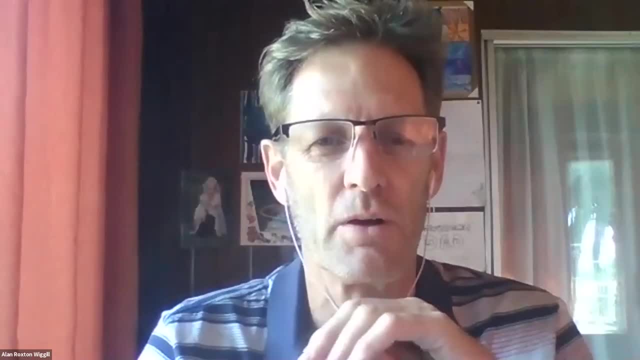 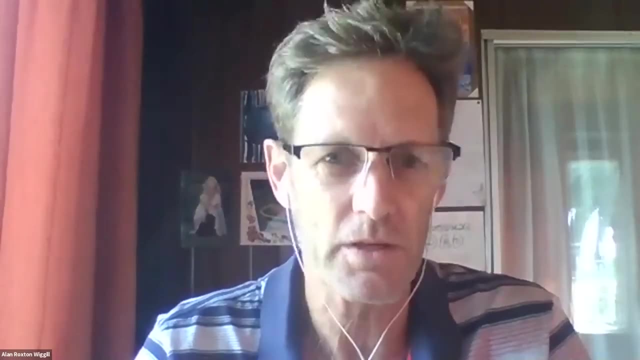 and some excellent virtual events. So we would need a million rands to be able to launch four or five of those, And then we would need a million rands to be able to launch a tour in each or two of the kind of structures that we need to do it. 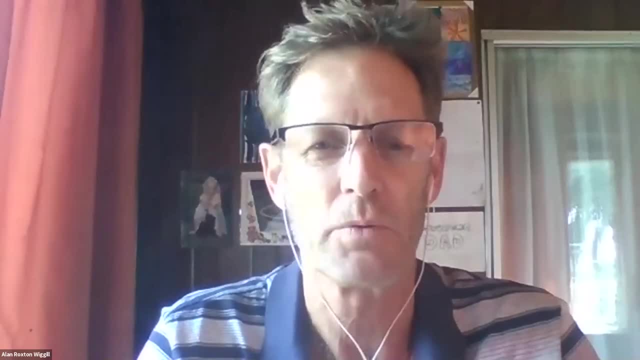 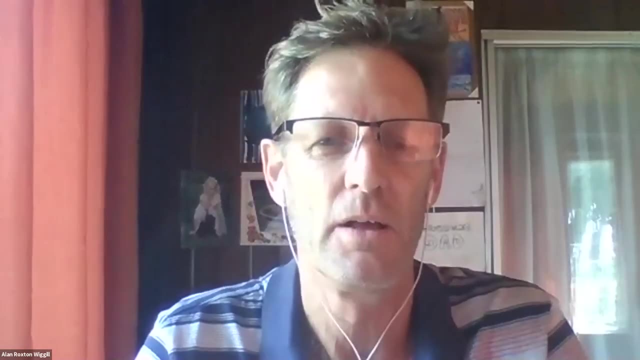 So a million rands would kickstart us with three tours or three regions- should I say three regions, destinations, In that we can incorporate a lot of routes and we would have sufficient collateral, marketing collateral to do it with. on that basis, 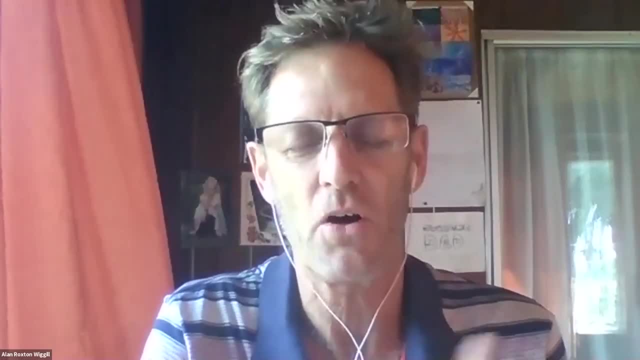 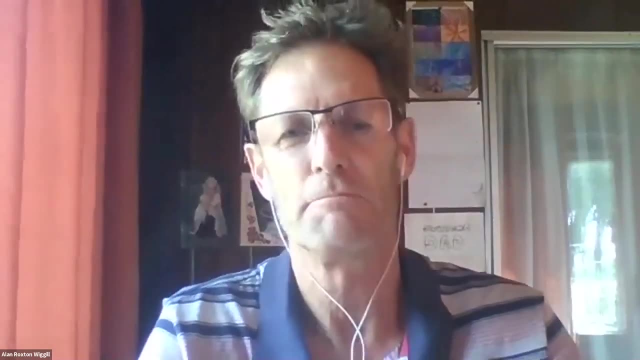 Plus we would have some money to go and do quite a lot of social media marketing towards the tourism trade. So it's far easier to reach and far cheaper to reach than it is to reach the public, because that requires massive broad marketing. This is a very narrow range of marketing. 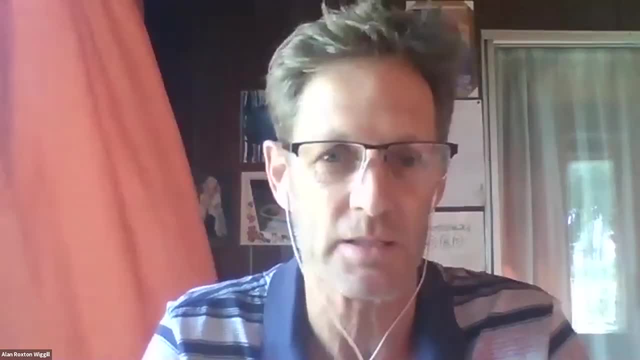 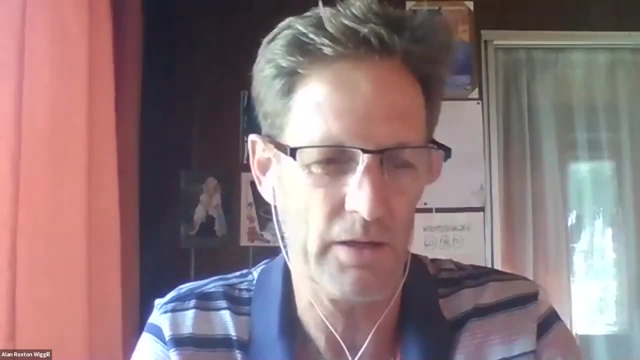 It happens to be where I'm a specialist, and I've been doing it for nearly 20 years now, So that's really my bread and butter. I know the tourism industry well. here I ran, for example, I see, of the N12 treasury development. 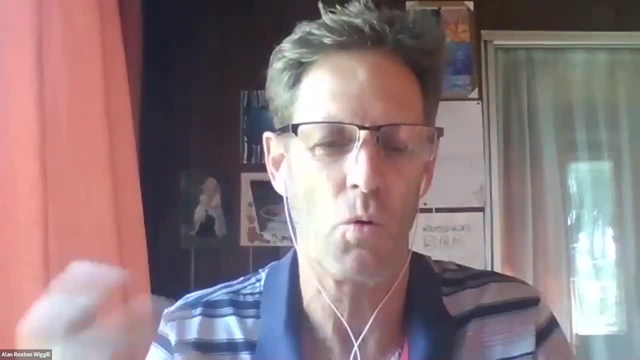 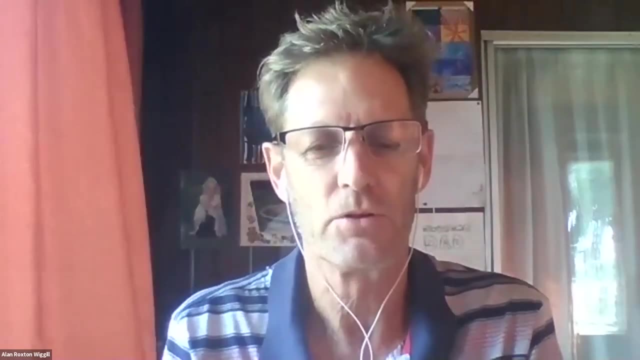 and I started- I was chairperson of the Denikin Game Reserve, which is a coordinated tourism product that's been produced, So we can reach far more people far more effectively through marketing, through the tourism trade, And to do that we need a good website. 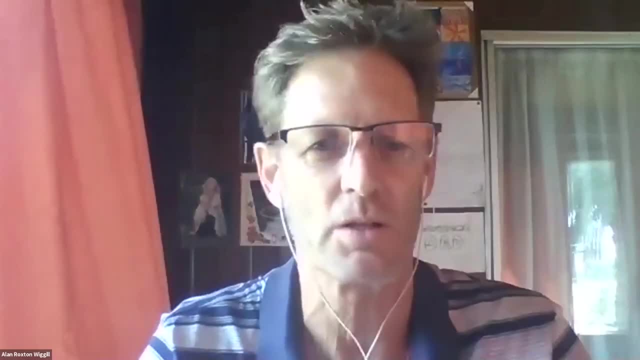 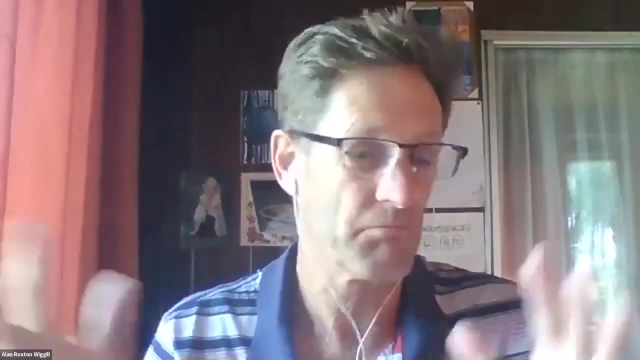 with great content in it, which we have. We have incredible content really, really available. I've spoken to Bruce Rubidge, Wendy Taylor and many other geologists already and paleontologists and archeologists, And they all have what they've got it. 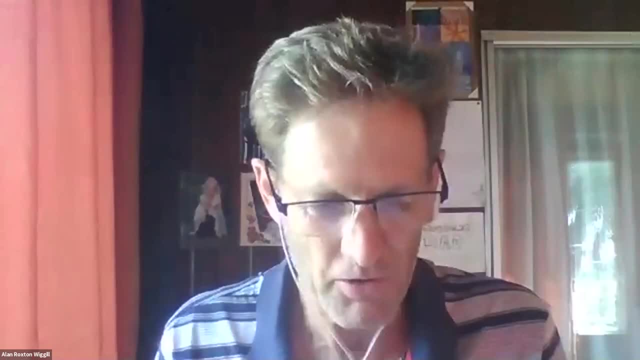 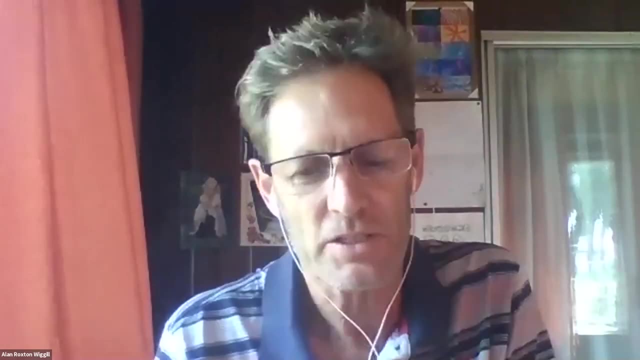 Everybody's got it. Richard and Morris are frustrated because they're not getting their tours out there. They're not getting their tours out there, getting the stuff that they developed and all the content out there. so how long is a piece of string? we should aim at a million rands. we'll be able to market this thing very effectively. 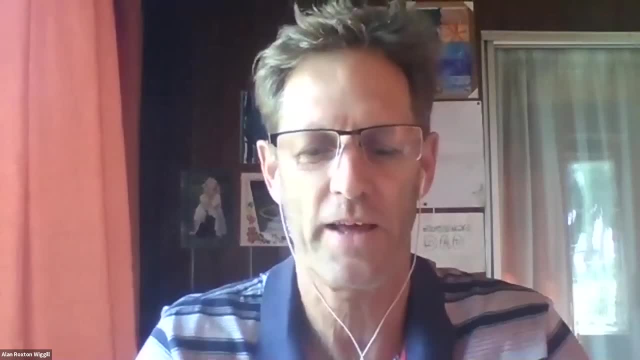 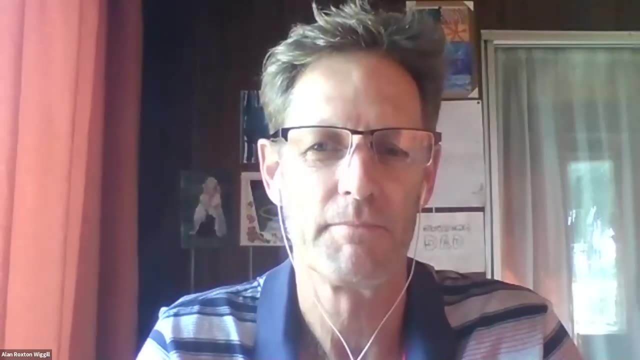 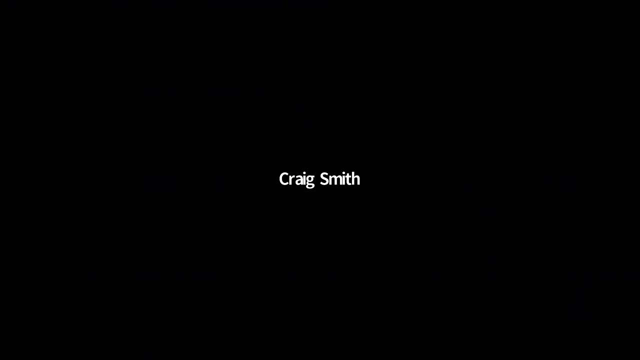 into the tourism trade for the next two years. anything more than that would be an absolute bonus, and we can start producing some really incredible stuff to go to market with george. you have your hand up, george, are you there? george, you've got your hand up and you're unmuted, but i can't hear anything. 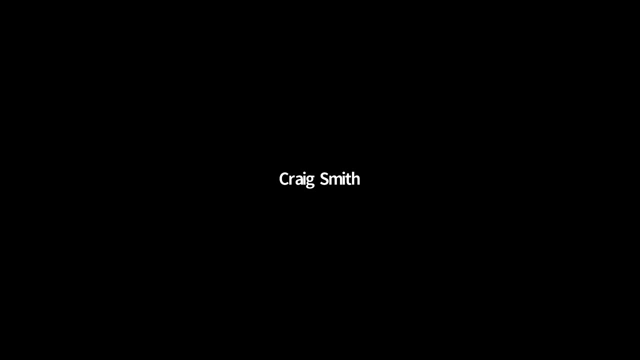 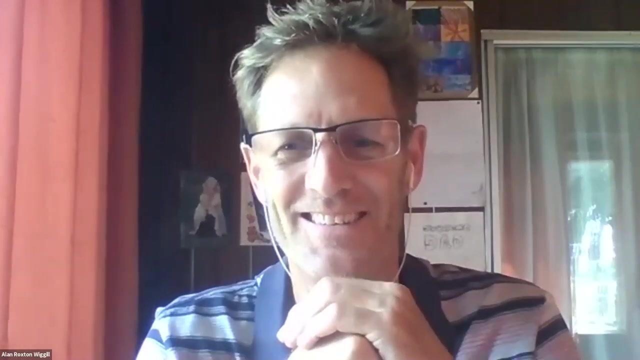 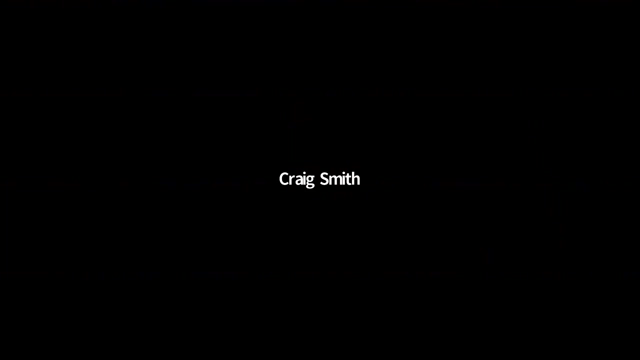 is there anybody else with comments or questions? i didn't think i covered it that thoroughly. come on, guys, don't be shy. everybody's got ideas. everybody's got ideas. george has disappeared. well, if, if, no one has any more comments or questions, i think you've given us a lot to. 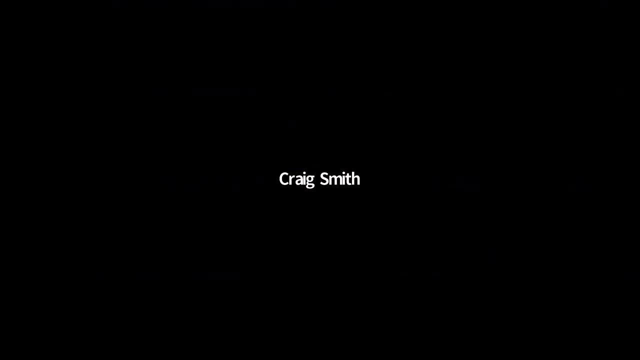 think about and some sort of structure is needed, i think pretty clearly for post-covid times. it may take a while to recover but it will recover. and of course, south africa does have the super superlative geology and i think it's going to take a while to recover but it will recover. 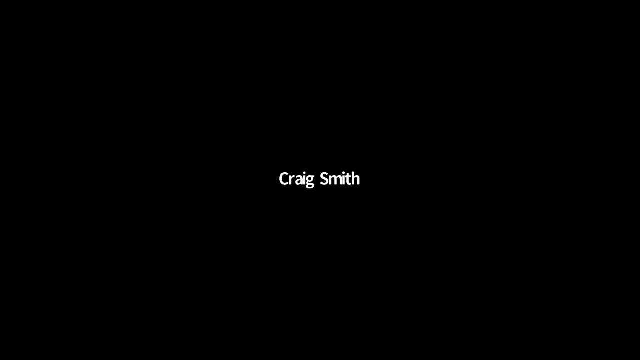 everybody's called georgia. it took a long time to solve the geology to show everybody georgia. i must say that as the as the manager of the gssa, i routinely get calls from vom brittain from elsewhere in the world. i'm coming to south africa and i'm going to such in such a place. what rocks can i go? look at? 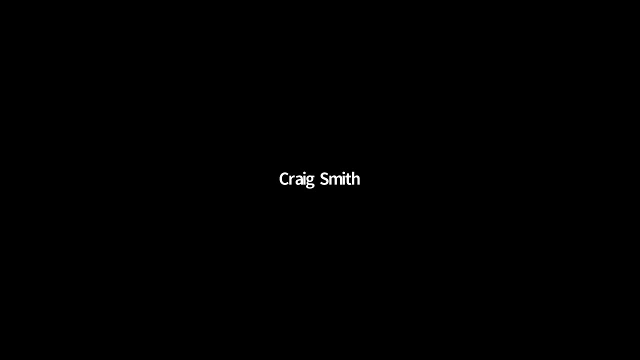 and this usually comes from interested lay people, not professional geologists. so the interest is there, uh with with that, i'd like to thank once again takoma strategies for for uh, we're on the governor's side- for sponsoring the session, and thank you to Richard Morris and Alan for providing. 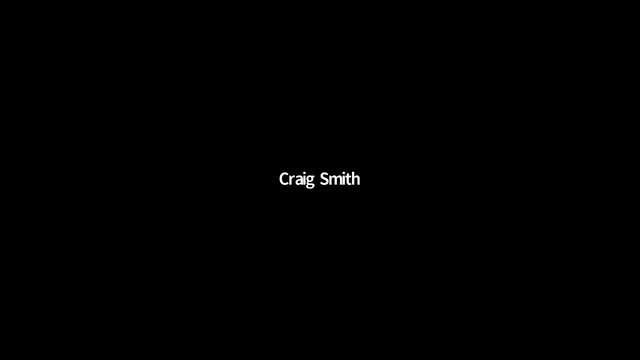 some an excellent presentation and food for thought. with that I'll give it one last chance for comments or questions. going once, going twice, it looks like you've sold your product, so with that I'll close the meeting. thanks for attending everybody. have a great remainder of the day. thank you very much. 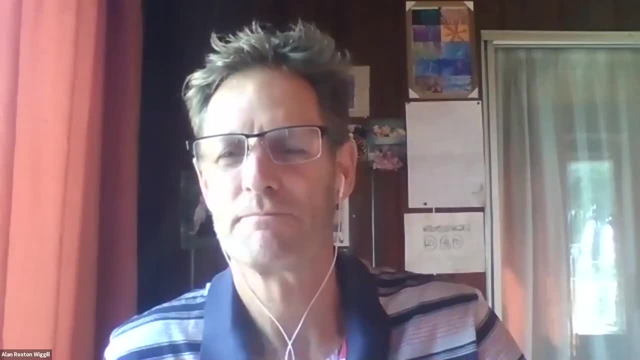 I'll end the meeting now. thank you, Craig.